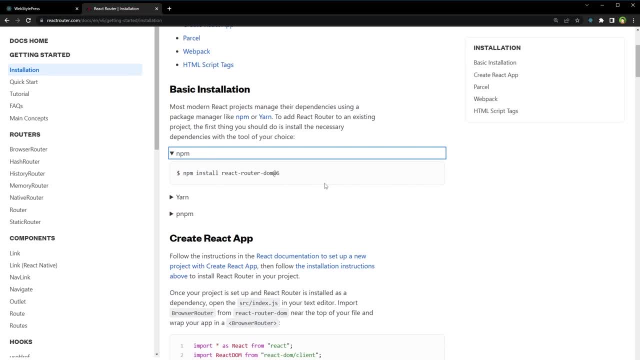 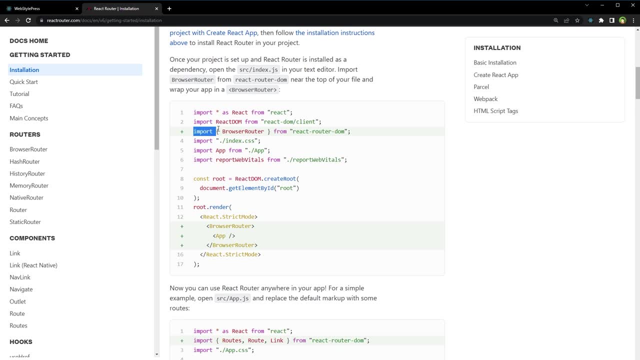 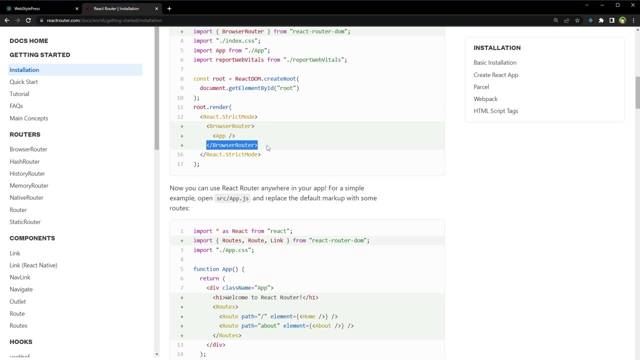 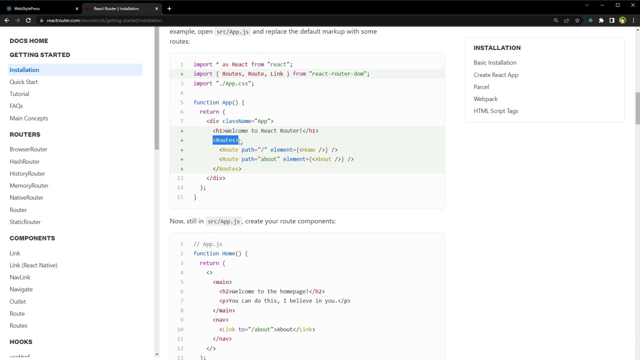 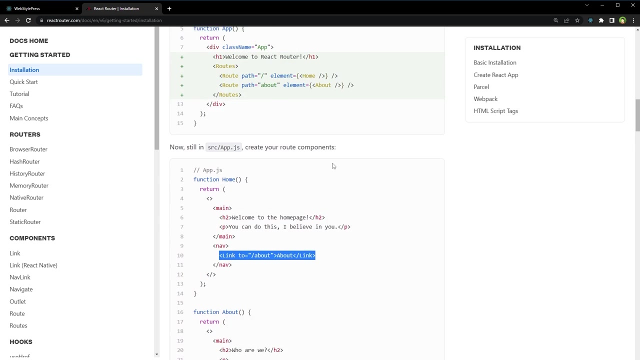 we have got installation page and for npm: npm install react router dom. import browser router from react router dom. and then browser router will wrap the app. and here are the routes: this is parent route. route is using path and element, two props and these are pages: home component about component and this is link component from react router dom. 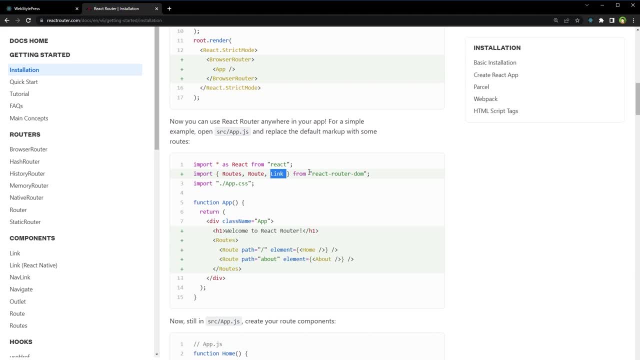 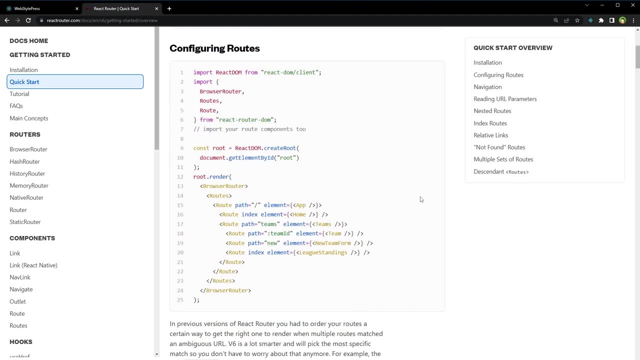 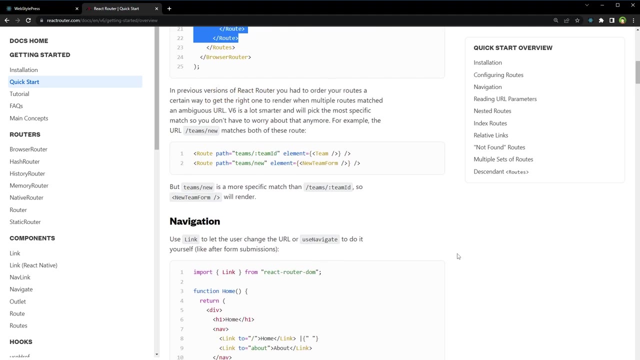 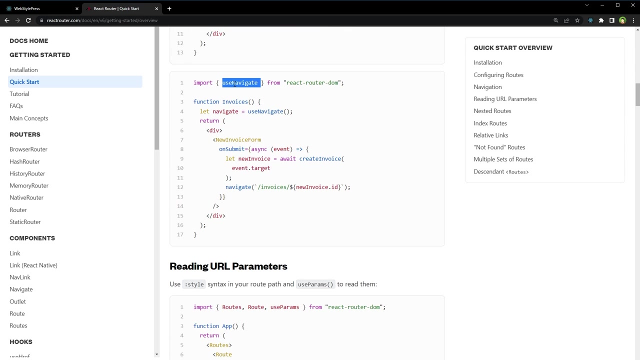 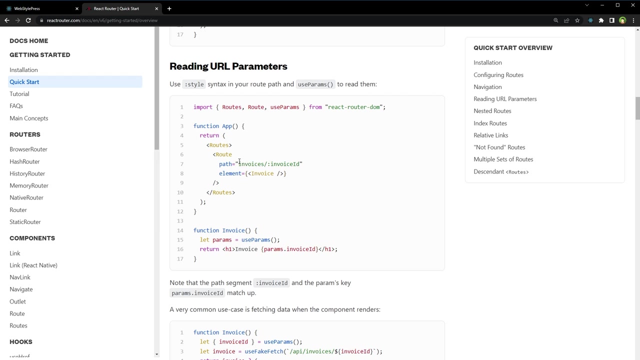 routes, route link are imported from react router, dom also browser router, quick start browser router. parent for the routes and these are the routes for the navigation link can be used to navigate to different location. we can use use navigate hook. we can read url parameters. we can have nested routes. 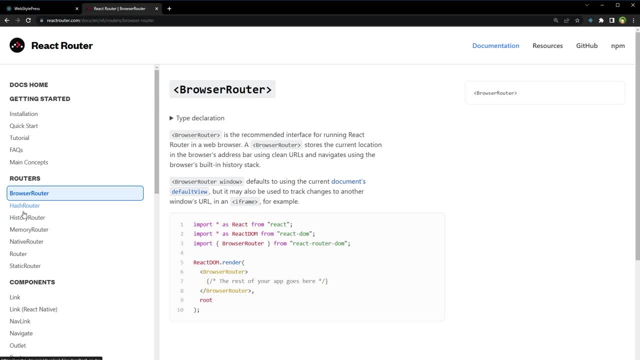 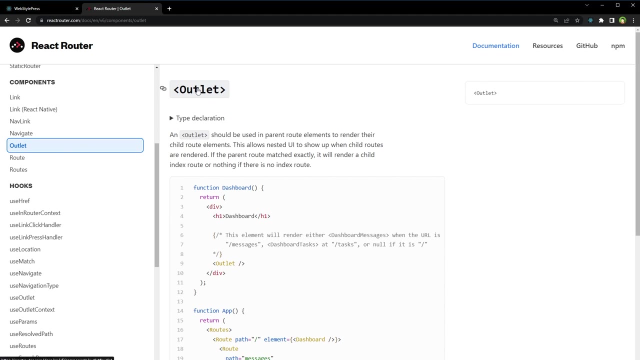 react router provides browser router, hash router, history router, memory router, native router router and static router. also for components we have got link, nav, link navigate, outlet, outlet is very important. we've got route and routes and for hooks we have got use match, use location, use navigate, use outlet, use params. 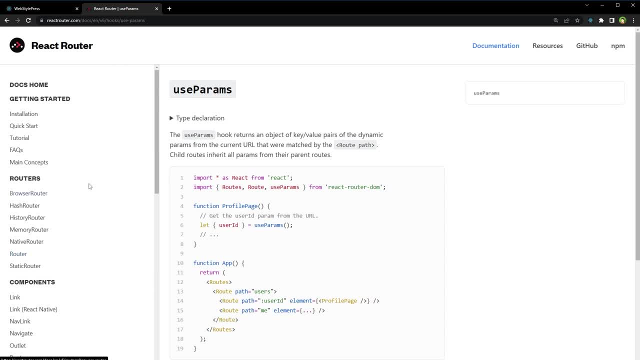 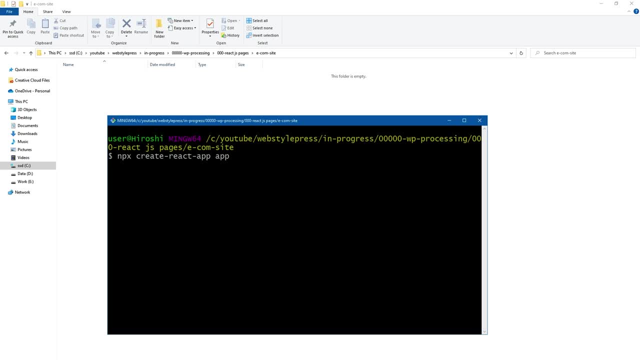 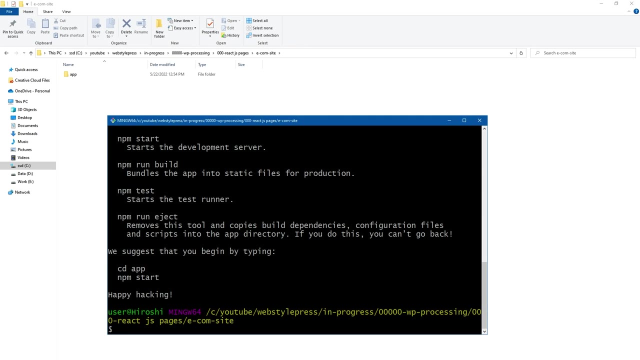 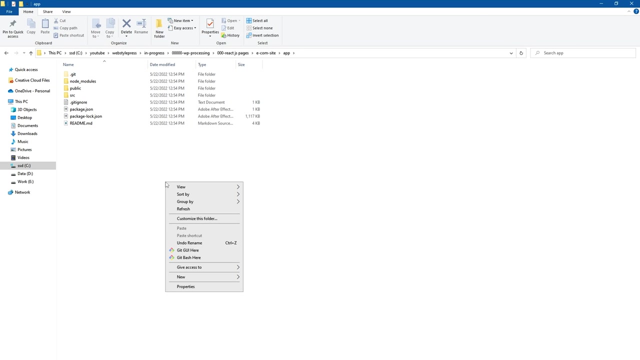 and more. okay, so let's start. first of all, open your terminal. i'm using git bash, use command npx, create tracked app and use app name. our app is installed. close this terminal, go inside the folder copy path, right click git bash here or open terminal again. 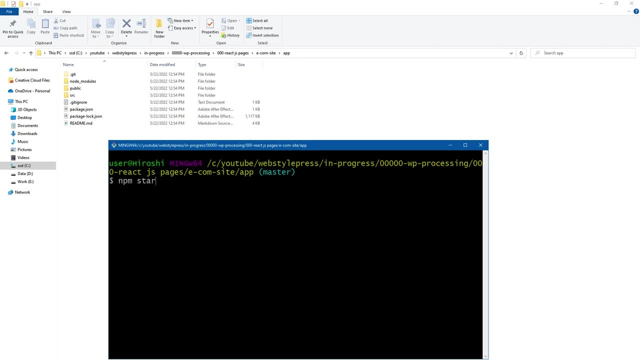 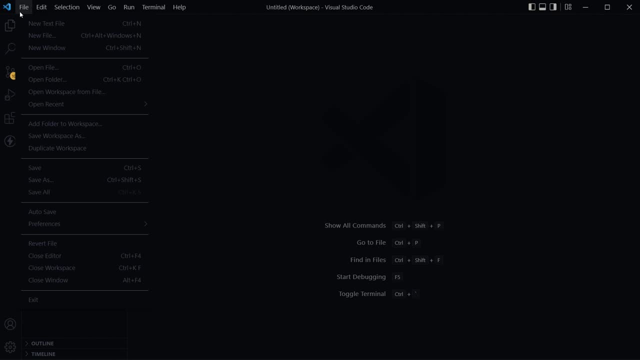 this folder. use command npm. start to start the app and also open the project in code editor file. add a folder to workspace. browse to the folder, add the folder and here is our app and it is running here. let me just remove stuff that i don't need for this app. 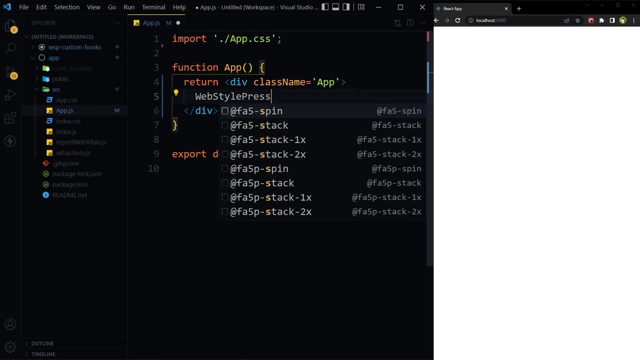 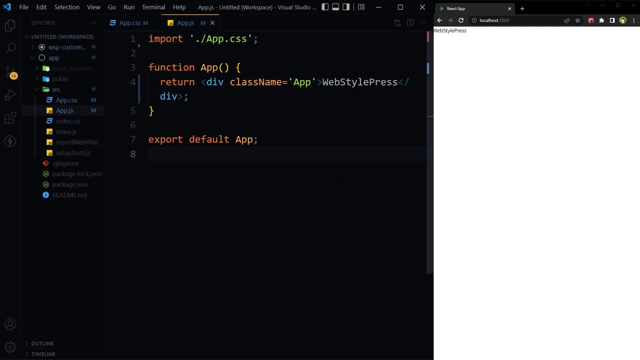 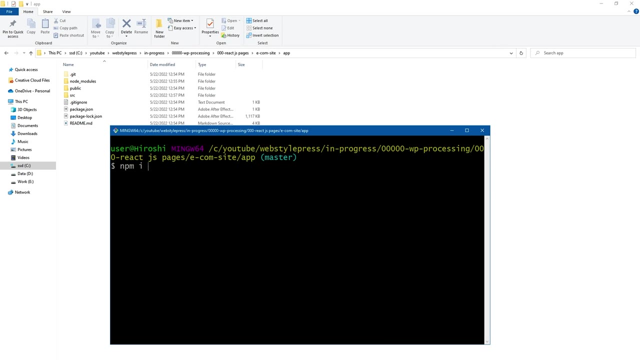 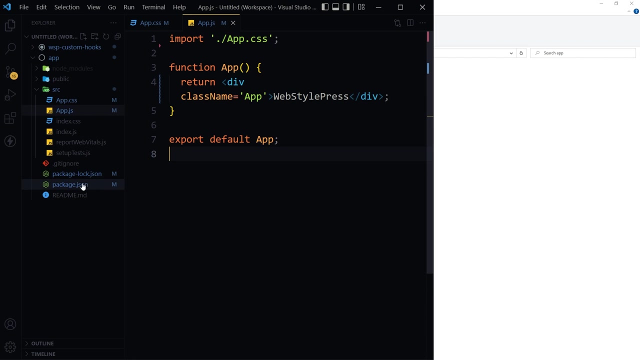 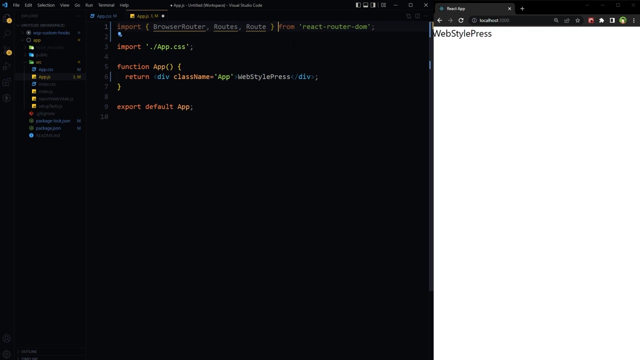 okay, right now we have this, let's install dependencies. i will open another terminal in the same folder and use npm. i bootstrap and react router dom package is installed. bootstrap and react router dom you okay. so let's import browser router routes and route from react router dom. 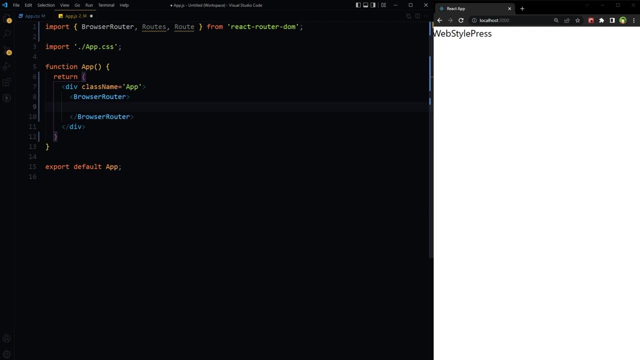 browser router. it will connect the app to the browser routes. this is parent for all the routes and then route route will contain actual pager path. route uses two props: path and element. path will be page url, like here we can use slash, and here for the element or for the content we can use home and let's use about here. 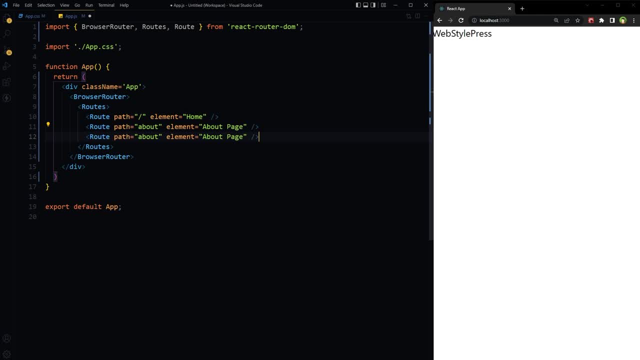 about page: products page save. and now site is reflecting home and from the url. if i type about, it gives me about page and if i type products, it gives me a parts page for the element. instead of this simple text or content, we can use component like home and here we can have about. 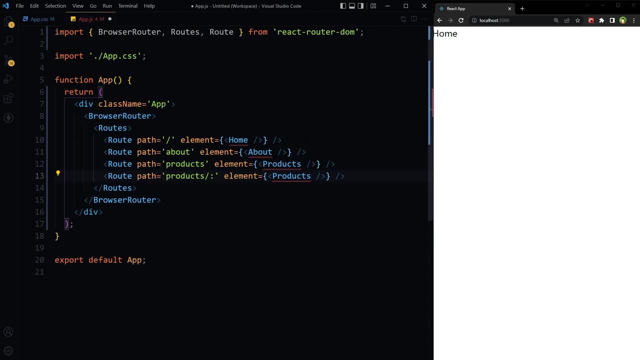 products for single product. products for single product. products for single product. this is, this is, and also one of the most important parts that this url will take to communicate with our user. so component will be here, which will be: this is id parameter, and here component will be used. 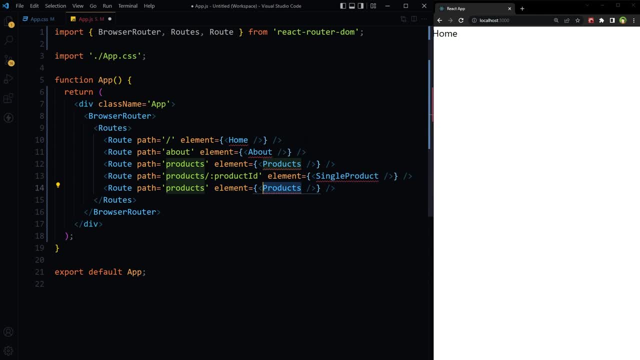 this macro line in the path comes, it will be single product and here component will be used. it will be single product. i will use another page for posts. its path will be posts and i will use another route with hysteric. this is basically everything, not including this. if url will not be linked, it will not connect to this tilpor. 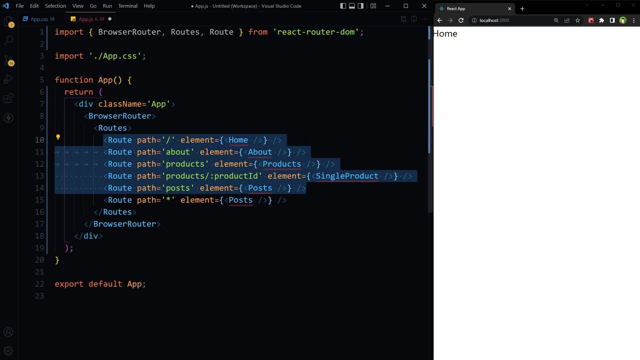 this is basically everything, not including this. if url will not connect to this until i get to the page, item is ready, will not have any of these component that will be loaded will be at a component, so this is our 404 page basically. so we'll have to create these components. basically home about products: single. 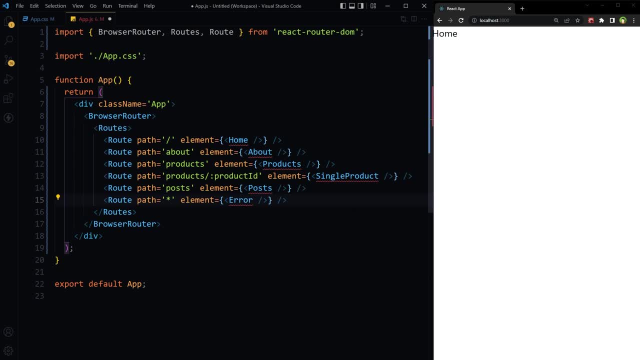 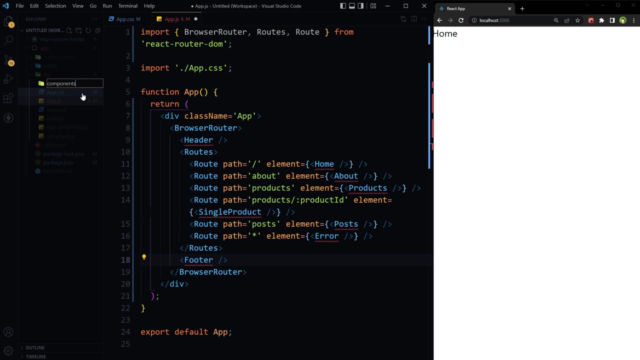 product and post never, and I will need two more components. those will be header and footer. I will use those here, head, footer, for now. let's quickly create these components. so these are components- header and footer- and these are pages. so I will create a folder called components. inside it I 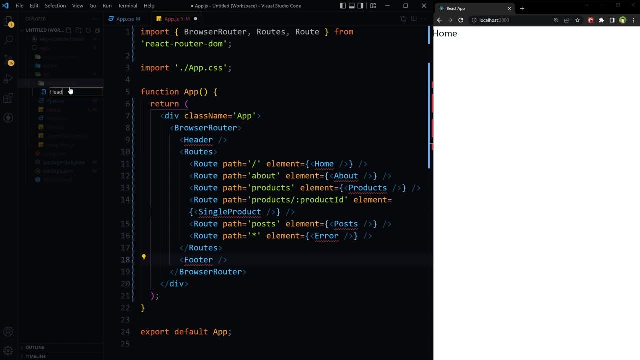 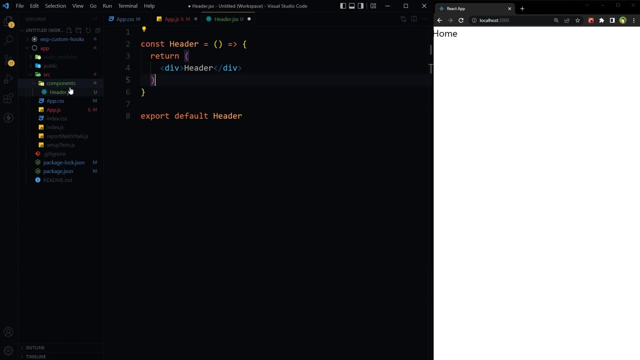 will create a file named a as headerjsx- rafc const header- export header. We can import link and nav link that we can use for this component from react-router-dom. Similarly, we will create footer for link and nav link For footer. also, we can have link and nav link. 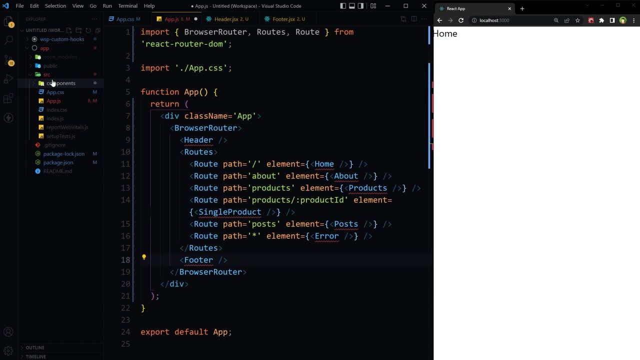 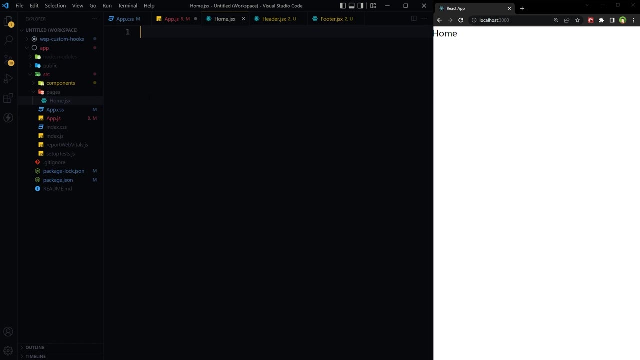 imported from react-router-dom. Now we can create these pages For that. I will create another folder pages inside it. file: new file: homejsx. home. component about component or page: products page: single product page. 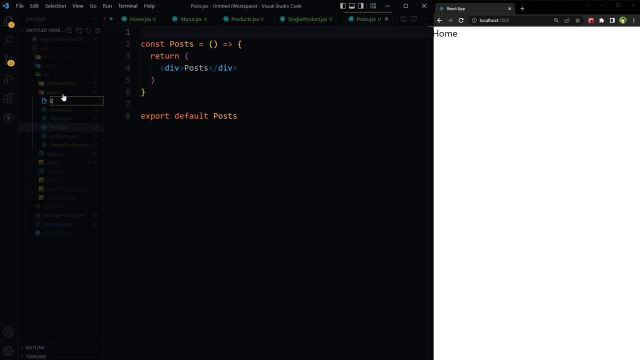 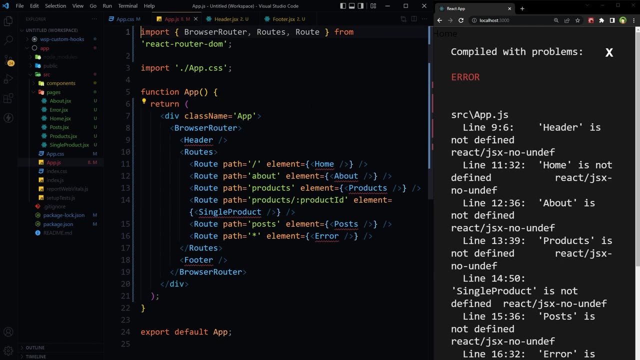 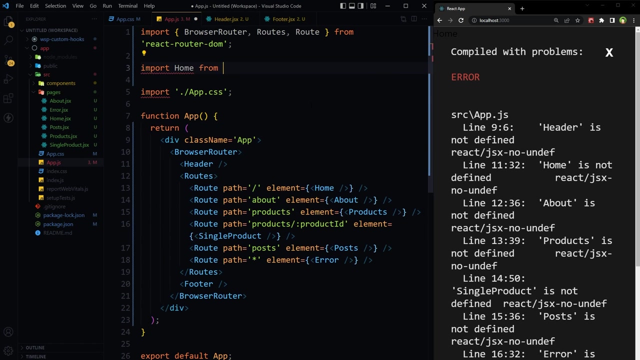 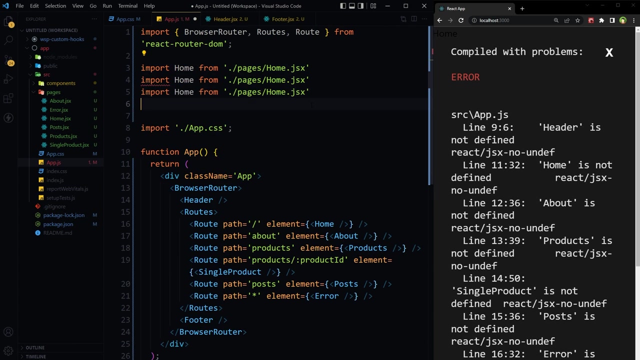 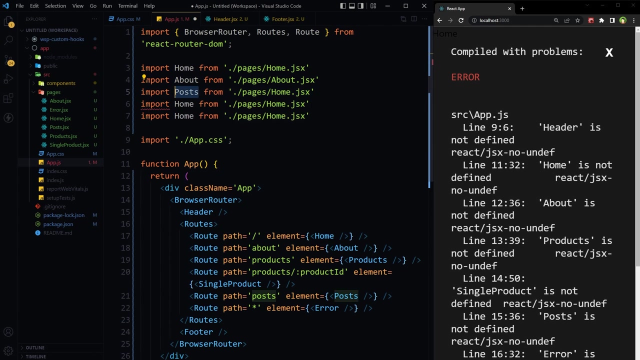 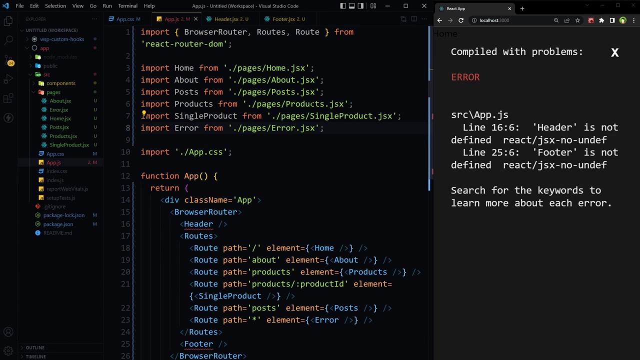 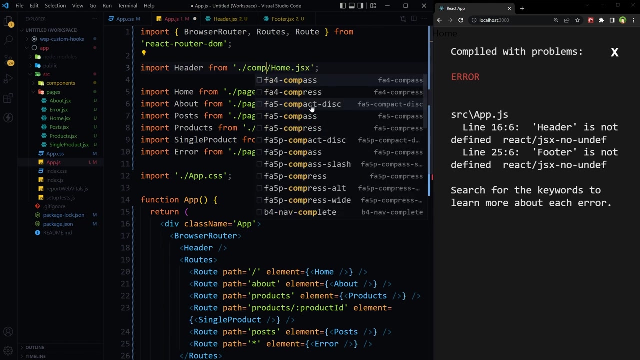 posts page and error page. Okay, Now we can import those pages and components here Home from pages home. Okay, this is home about posts products. single product header. header and footer are remaining. Import header components. 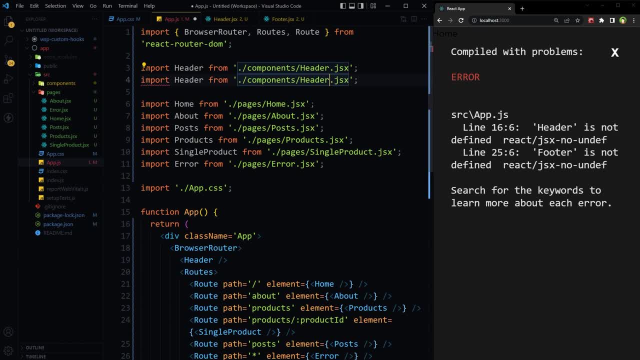 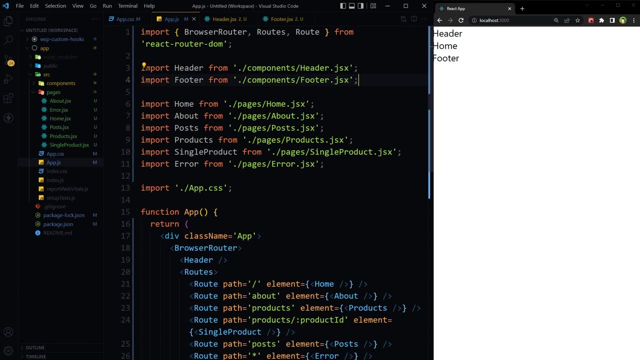 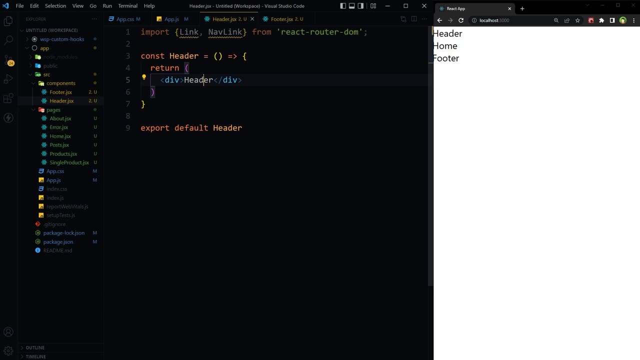 header and we have got footer Save. Okay, We've got header home and footer, So for the time being let's use a temporary navigation here for the header. So instead of div I will use header, header tag. 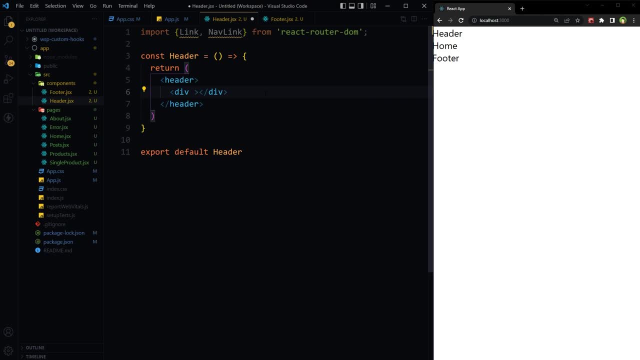 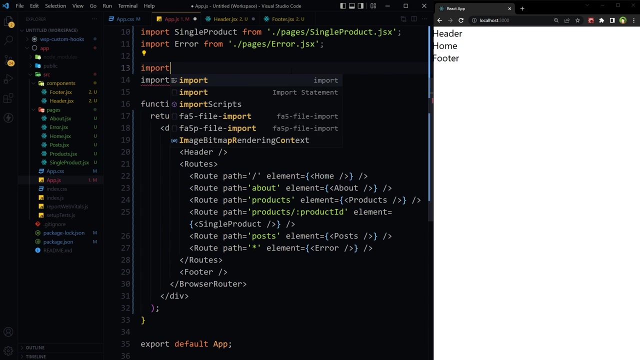 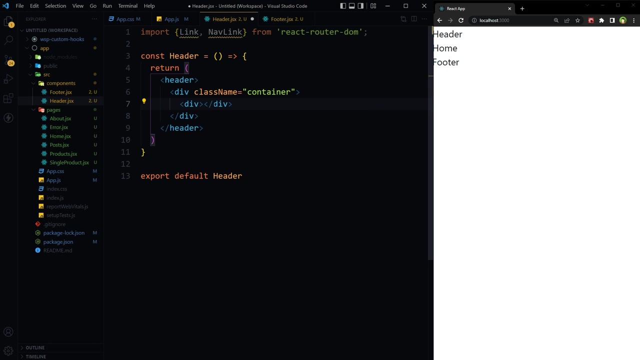 And here I will use class name container from Bootstrap, And I should also link Bootstrap here: Import Bootstrap test CSS, Bootstrap Bootstrapmincss. So here I will use class name display flex, justify content between and align items center. 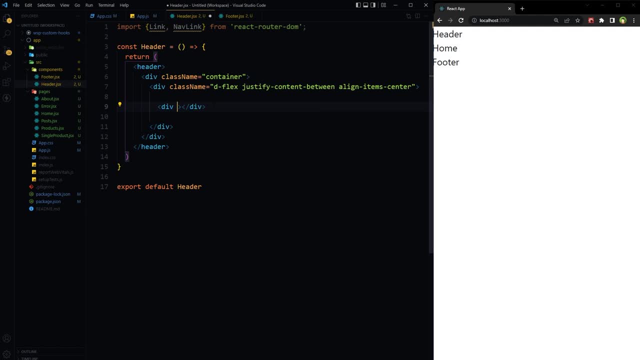 Okay, So here class name logo, Just use a text for the time being Link to home page WSB And for the class brand Save. And here class name: nav nav pills. Let's use single quotes. 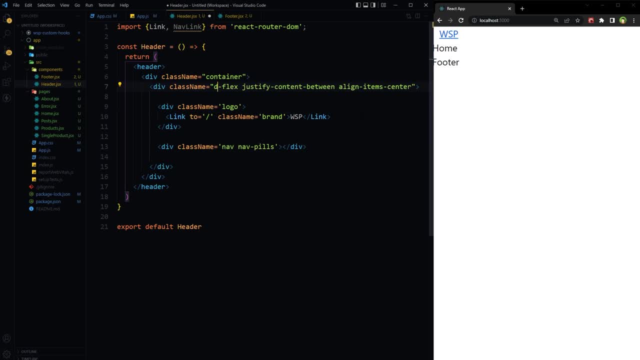 My code editor seems to prefer single quotes And let's use just links here. Class name: empty Home Save. So we have got the home About. It will go to about Products, Products page Posts Posts. Okay. 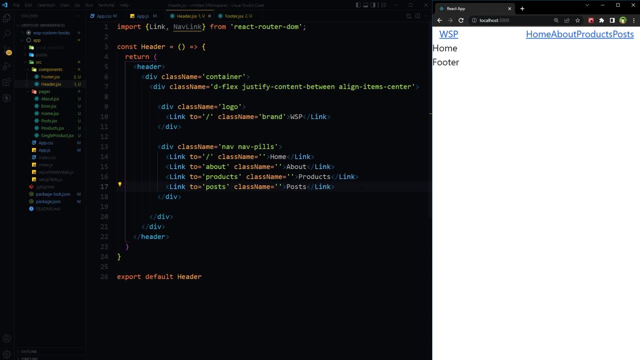 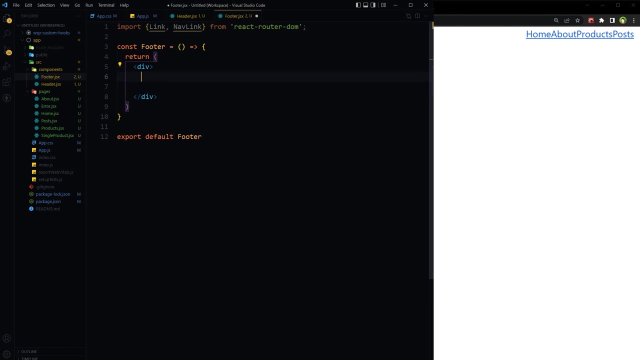 So this is supposed to be logo And this is footer, This is home. Let's just use same thing in footer. Okay, So home About Products Posts, So let's complete the footer as well, For the footer Footer will have same stuff. 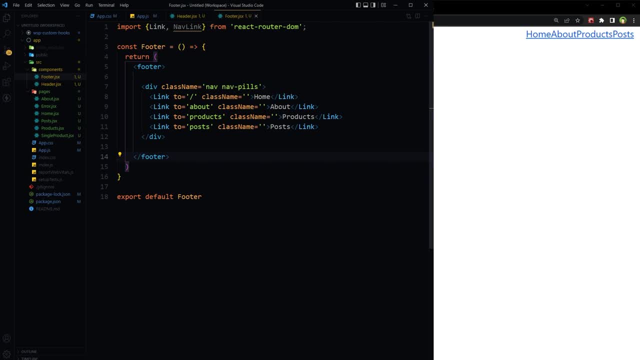 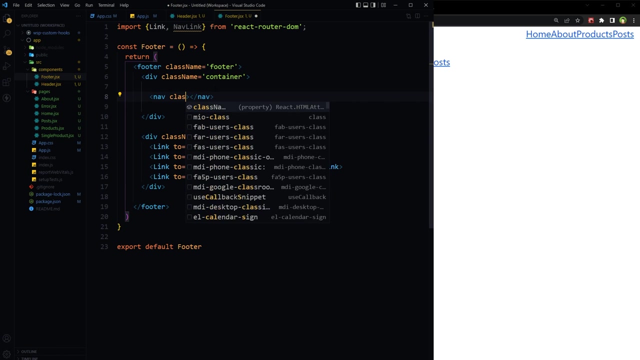 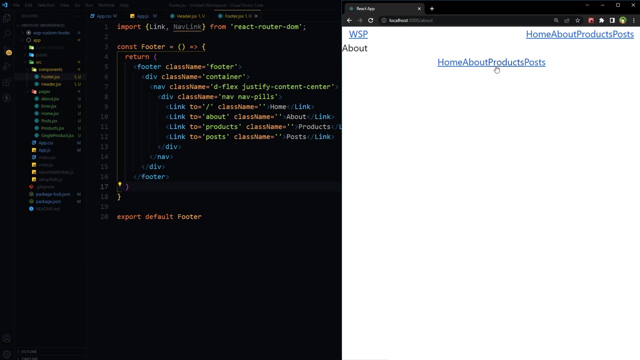 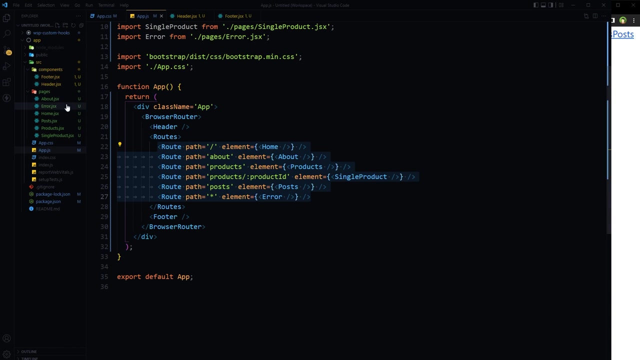 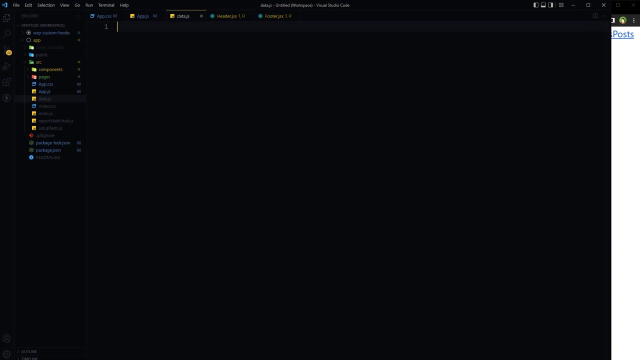 Footer tag: Class name, Footer Container Nav, Class name, Deflex and justify content center: Okay, Okay, So let's create and style this pages discriminators, but before that we'll have a data file: datajs- const products. 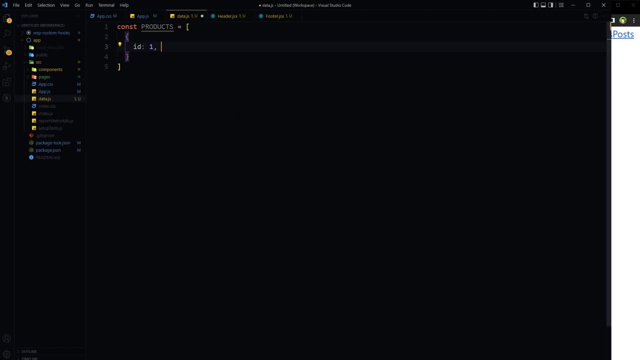 and this is one object. it will have an id name for the product price, for the product image, for the product images directory, one dot jpg and details. let's name it for the price. let's use 12 dollars for the details. this one, okay. so this is the structure. 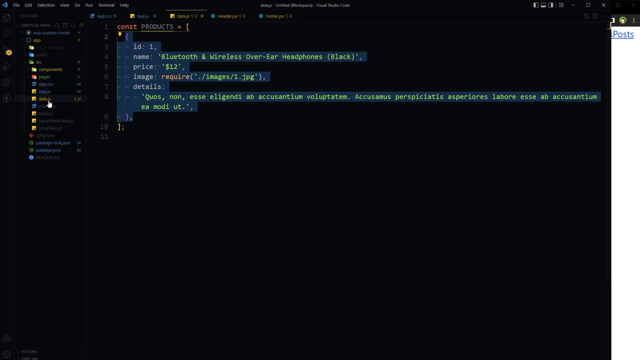 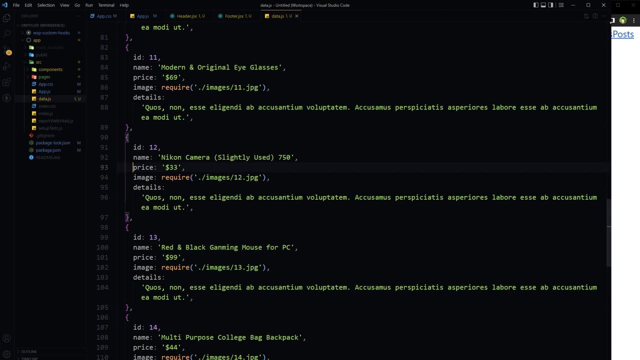 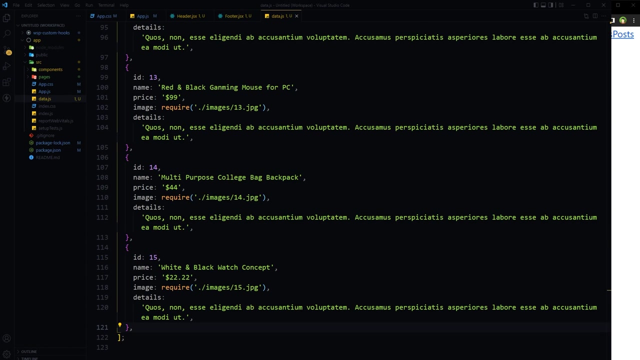 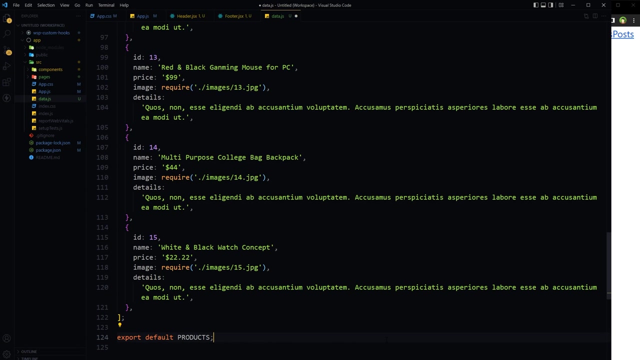 for our object, for one product in our datajs file and here are more products. so we have got around 15 products and because this is a javascript file, so it's like a module, so we'll have to export it, export default products, then we'll be able to use it. 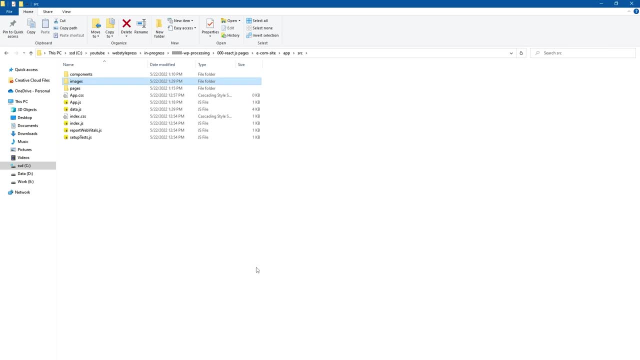 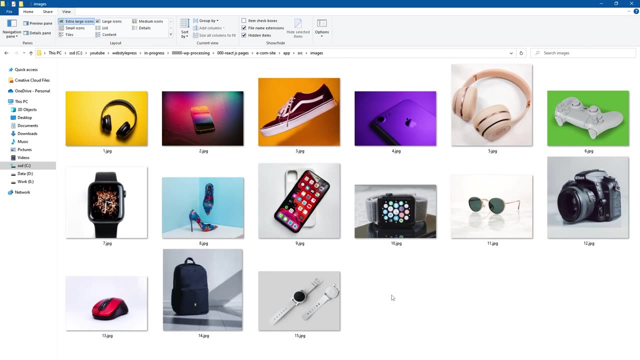 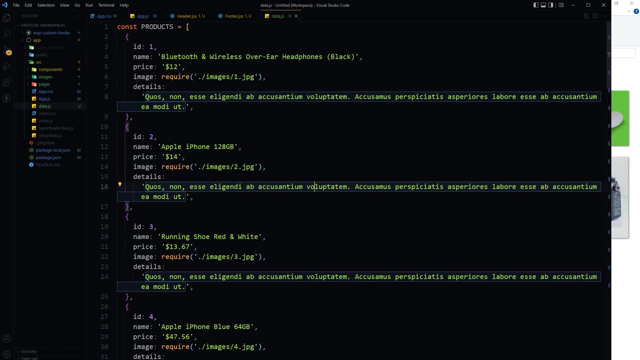 and we'll have a folder here for images and i will use these images. these are the images i have that we are using here, just one dot: jpeg, 2.jpg, 3.jpg. this is the path for the image that we'll use in our products page and single product page, so data will come from here, from this file. 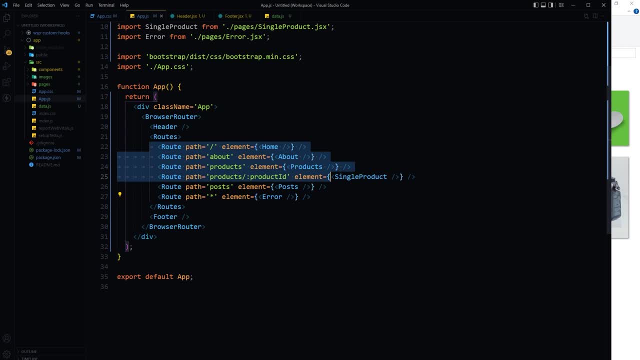 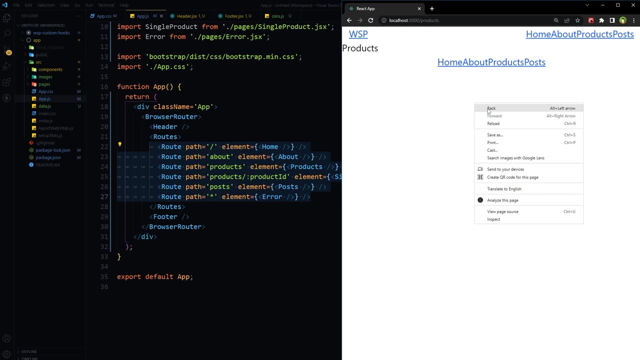 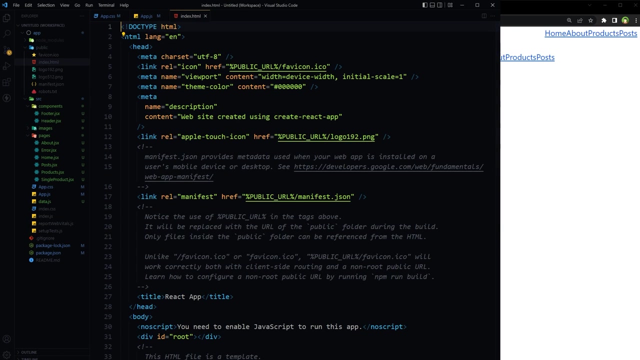 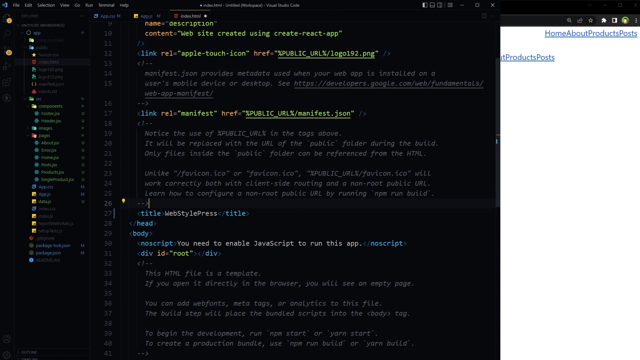 in our products page and single product page. so let's create these pages and style those pages and change look and feel for the app and make it better and improve everything. but before that couple of things- public folder- indexhtml- let's change title for the app and i will use one font family from google fonts. 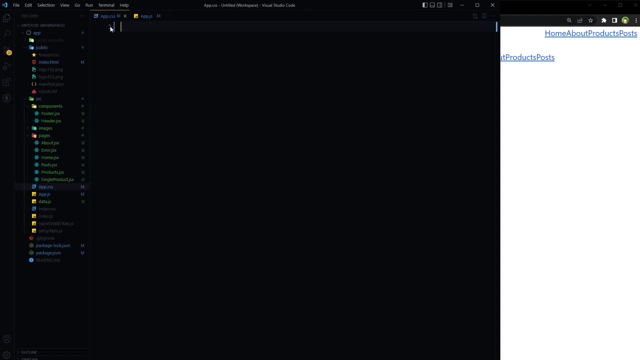 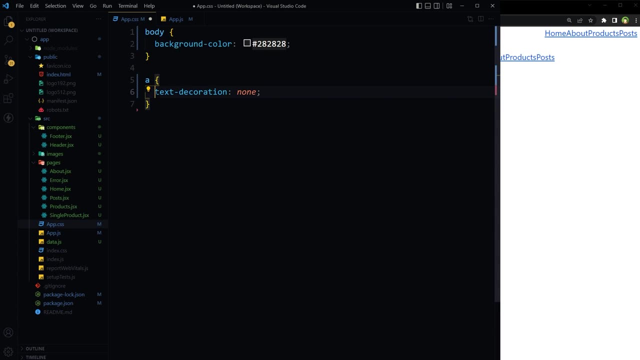 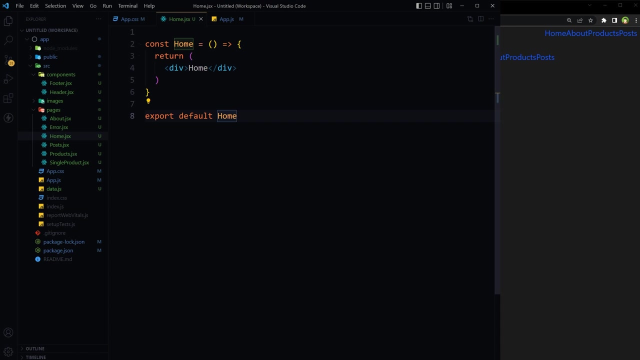 save title changed and also in our appcss basic styles: body background color, anchor text decoration: none, and that's it for now. close public folder. from pages folder home component: main container from bootstrap heading: welcome to web style press and this was header. this is content area with class content. here let's add: 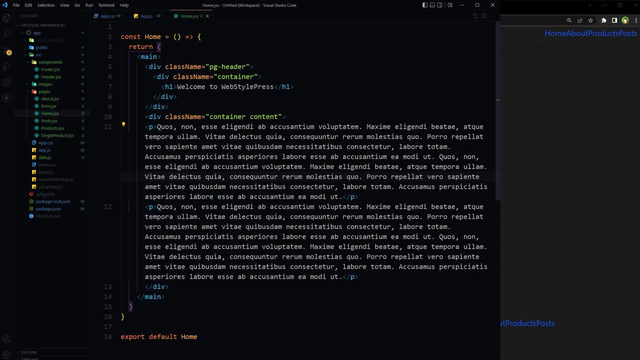 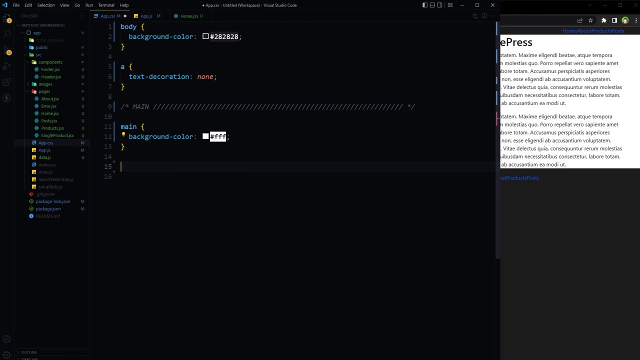 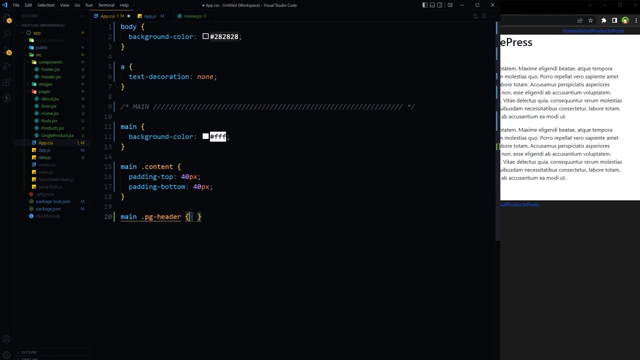 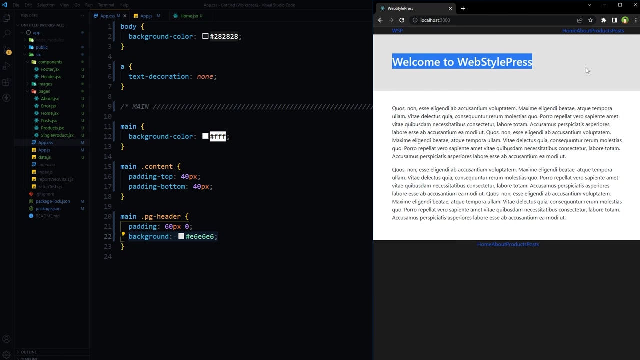 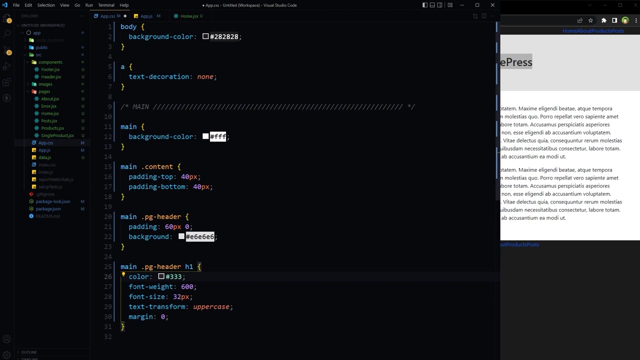 demi-content, maybe two paragraphs. again basic styling. we will need pg header content and main styles for these elements: main content: background: color white. main content inside: main padding: top and setting bottom PG header. that is page header, some padding and background so this looks better, right. and then s1 heading: color font weight, font size. 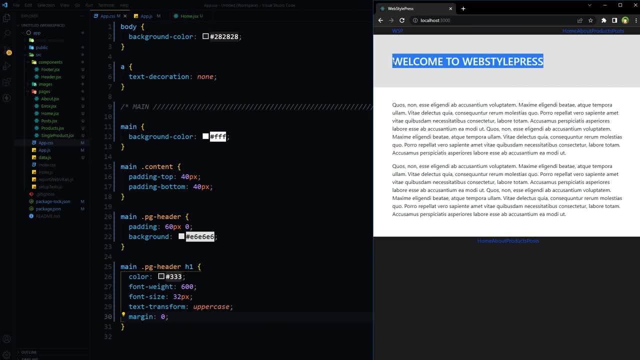 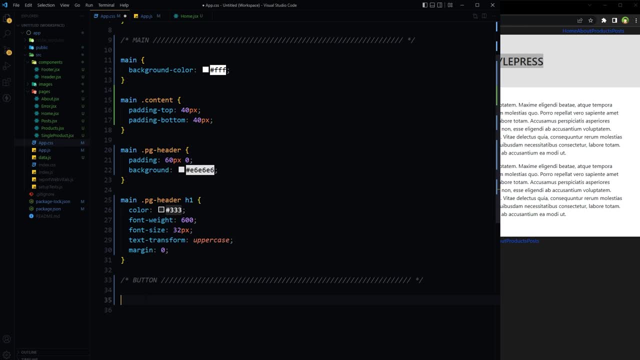 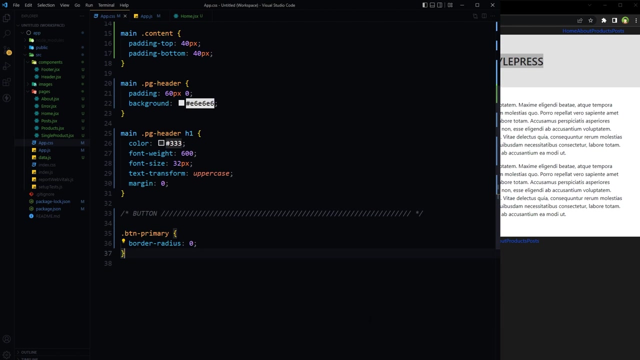 text transform and margin. I have also got style for button, because a button will be used. we didn't primary. that is inside bootstrap. we are overriding it, just removing border radius. we will also use breadcrumb, so let's style it as well. breadcrumb will have link. I want its color to be black and then a media query, if we'll have max. 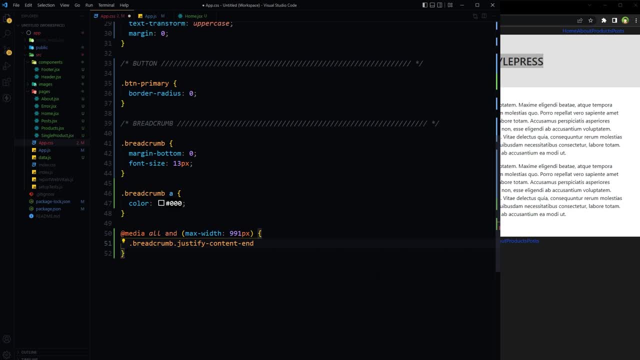 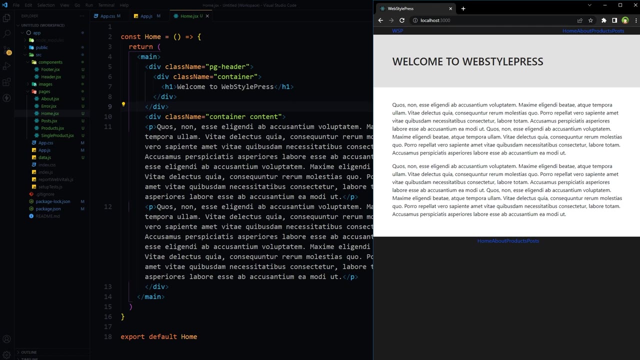 width: 991 pixels. then I want justify content and class to be changed. justify content, flex, start. that's it. so we have got home PG header and then container, then heading. this is the heading, this is heading area. we've got container and content and now this is footer and this is header. we will style header and footer in. 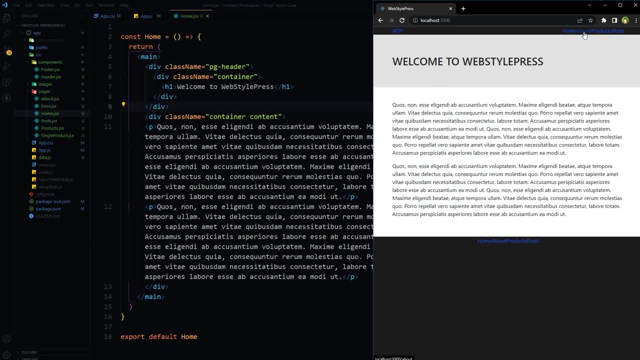 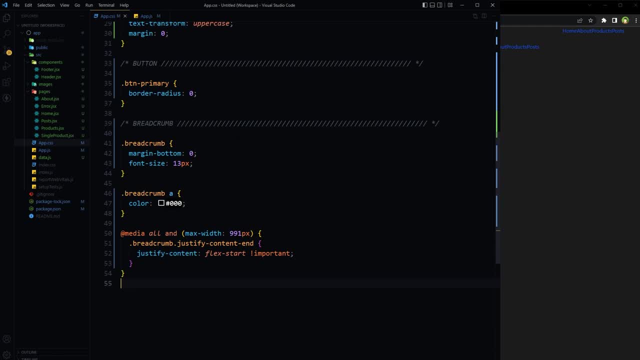 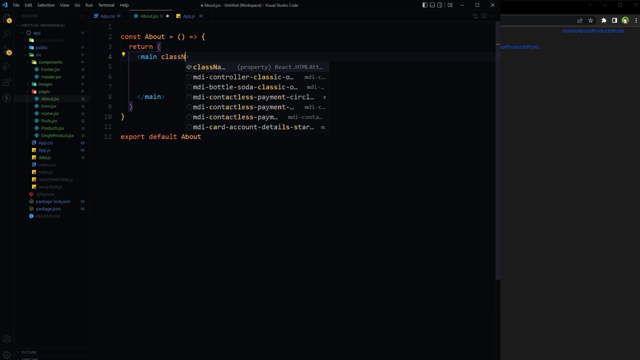 couple of minutes, but before that we have to add content for about products and posts. so home is done. let's go to about close home component and pages from pages folder about again same main. let's give it a class about. and we have pg header inside. we have 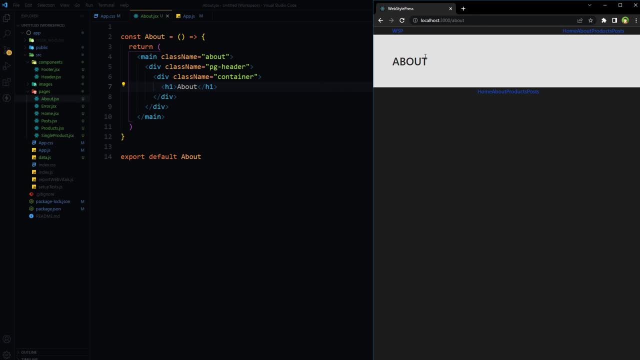 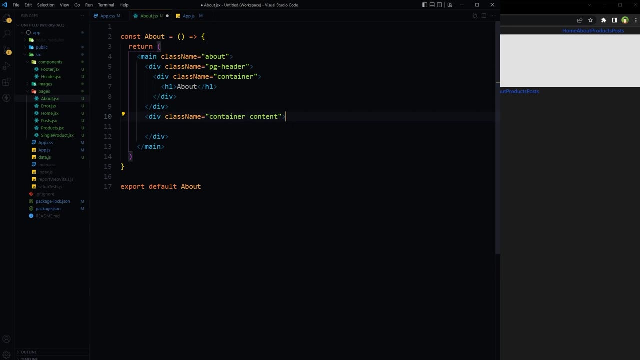 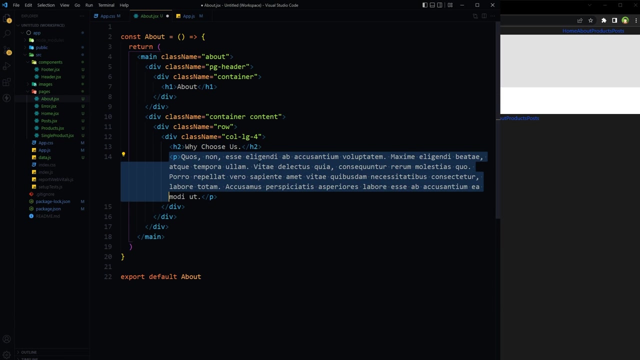 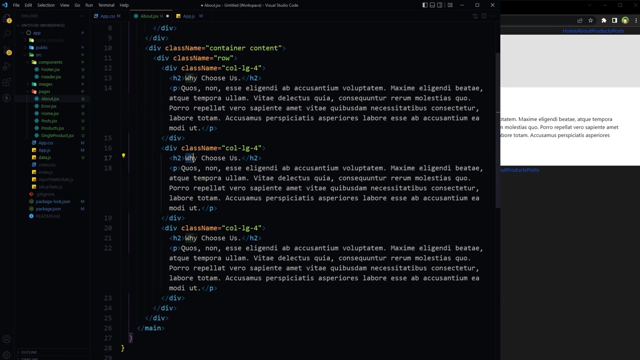 container and heading about then for the content: container, content inside it, raw, and then call lg4, save inside this column. we have a heading and a paragraph like this: let's make a copy of this column columns, let's change it to our mission and here what we do. 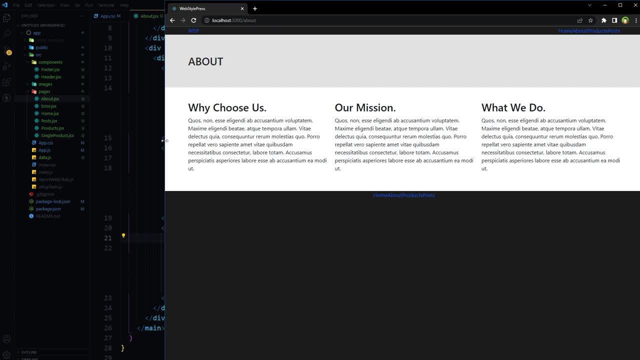 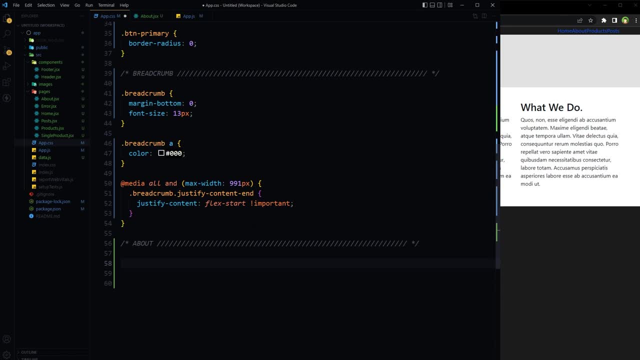 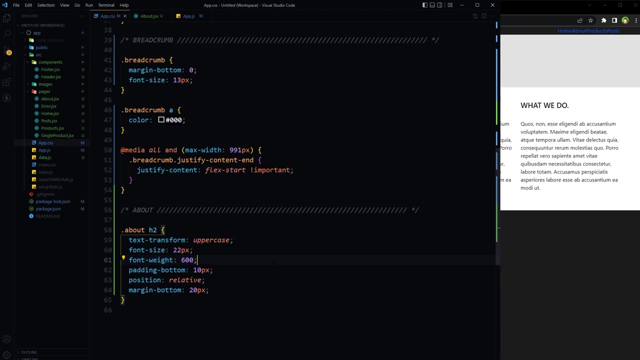 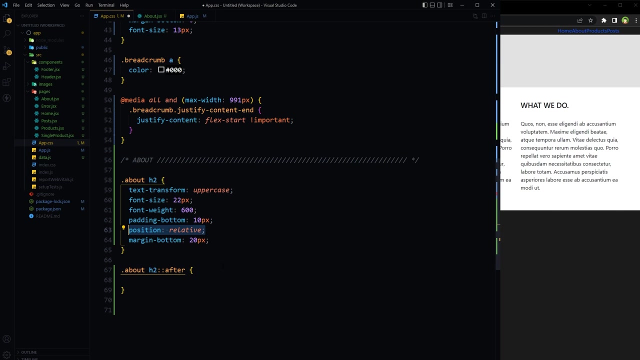 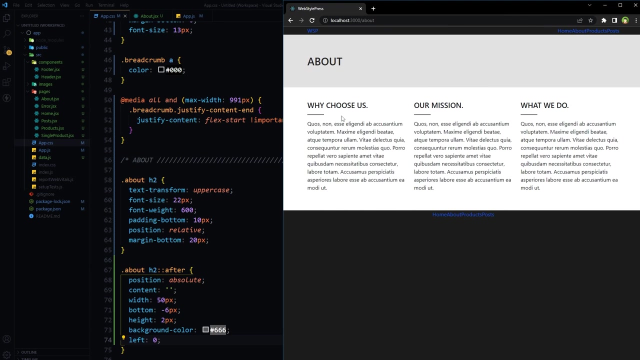 so this is home, this is about. so let's style about page, about class name, that's about H2. save H2 after and see we've got position relative for H2 and here we will use position absolute and basically we drew a line with 50 pixels bottom, minus six pixels, height, two pixels and 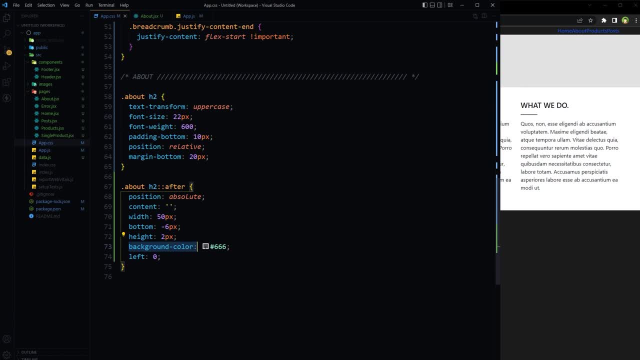 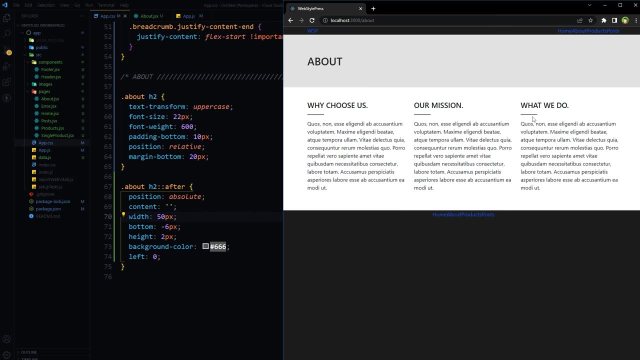 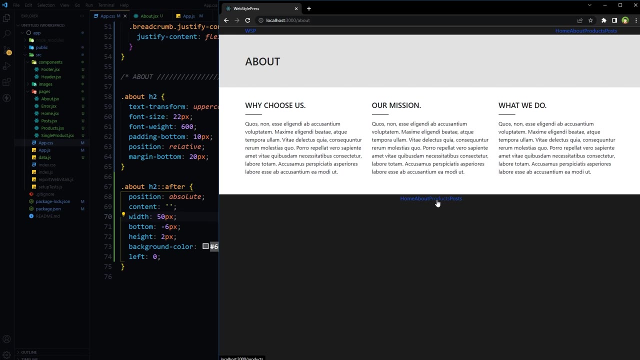 that's another whole and another look at. f said we could take a look at that other pictures, but these ones are two pixels and background color 666 and left 0 and its width is 50 pixels. right, that's about it home. about now let's move to products. about: page is also done from pages. 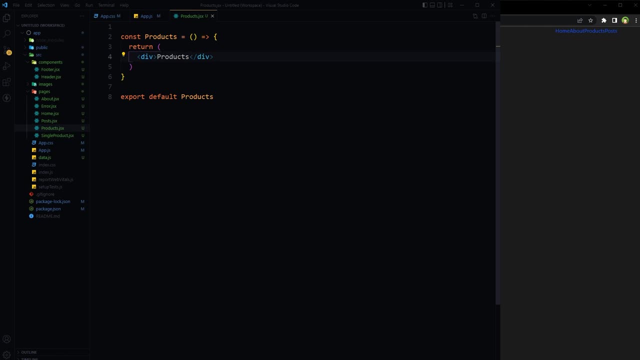 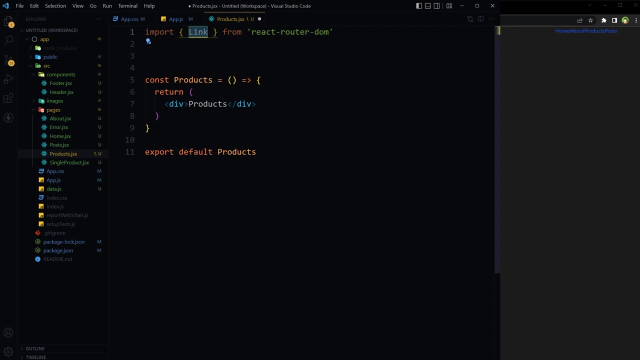 products. so first of all we'll import link from react router. Dom product will have an anchor that will lead to single product details, product details page. so for that we'll use link and then we will import products from data dot GS. so this component, products dot GS, is in pages. we'll go back one step. 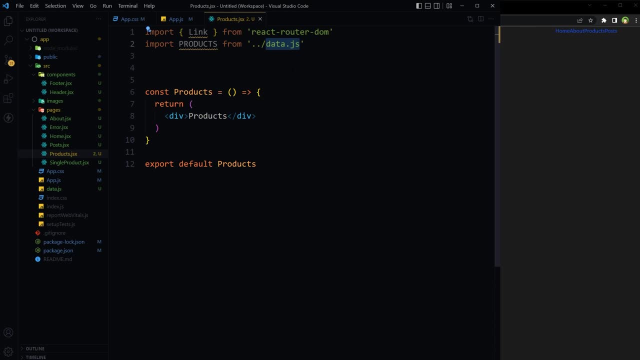 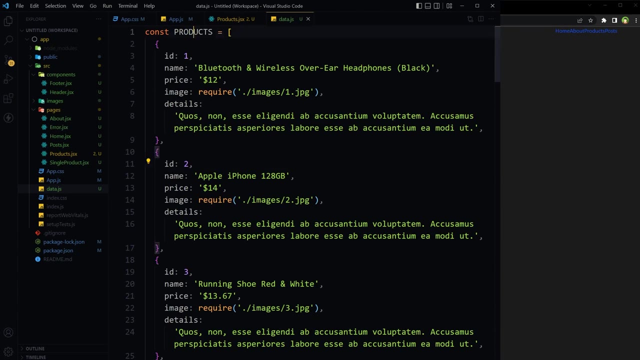 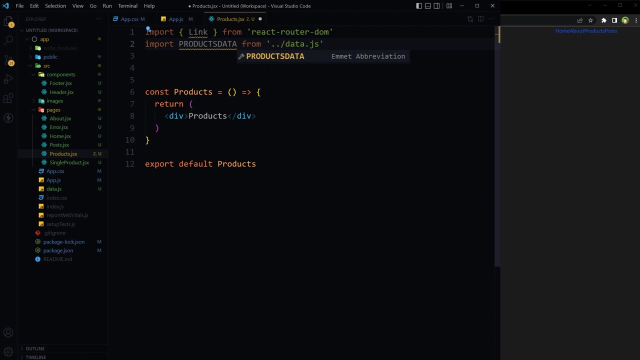 for that dot dot slash and then data dot GS. this file data will be fetched from this file products. we are calling that data with the name products. it can be any name, by the way, this is just the name. so man, man PG header will have container inside it. this is for the header area for products page. 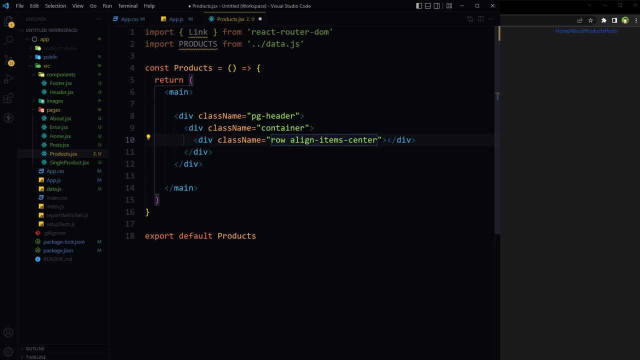 so inside container we will have raw and align items center and inside raw. we will use two columns. one is call lg7, with the heading and second one call lg5 and here we'll have breadcrumbs nav inside nav. well ordered list: class, name, breadcrumb. justify content and. 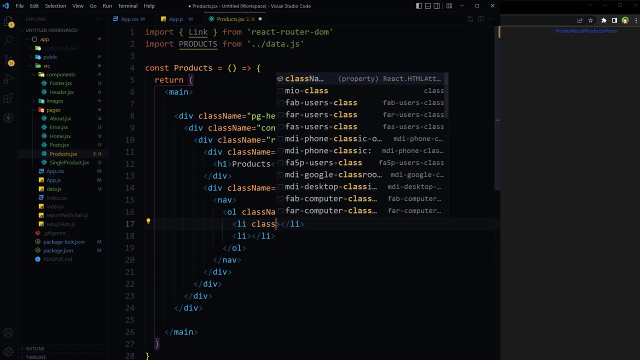 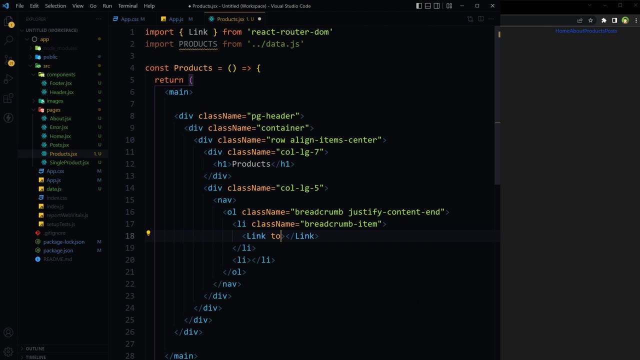 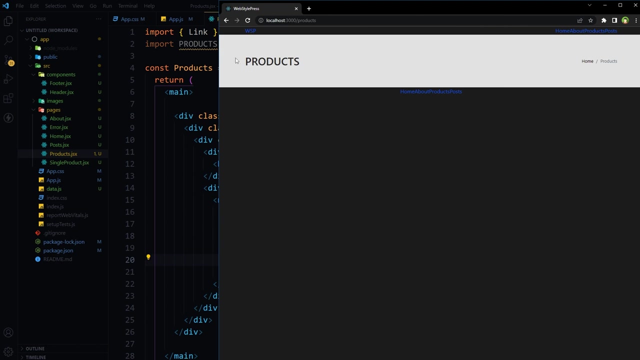 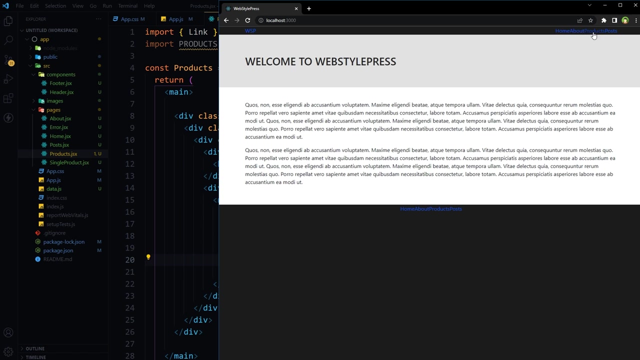 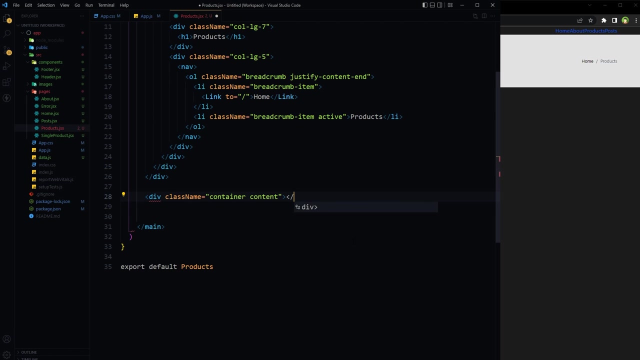 inside we'll have allies and here link home page with the text home and that's it also for second ally it will be active: gia page name, product, etc. page name. so this products and this is bread from home products. okay, that's that. and then we will have another container for the actual content and we will display products. so we will. 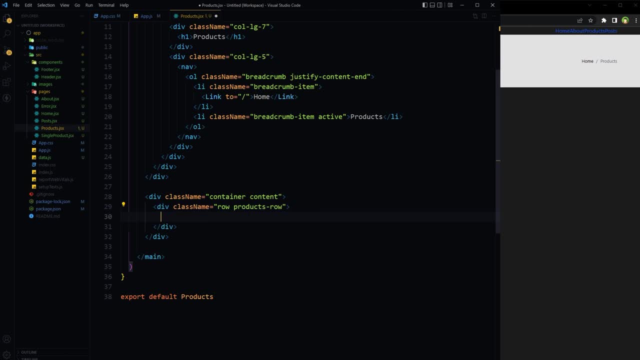 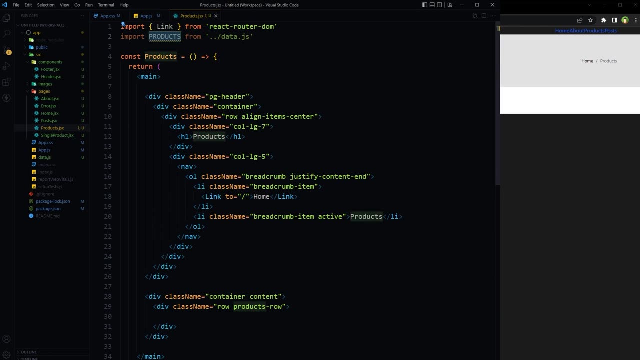 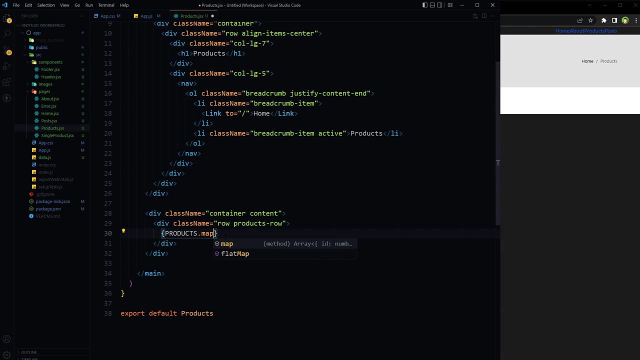 need columns and that is why we need a raw, raw products, raw, and here I am directly calling these products: yes, products, dot map, single product arrow function, return, and here will be it to column size will be called LG for, and here we need a key. let's use product ID: product from. 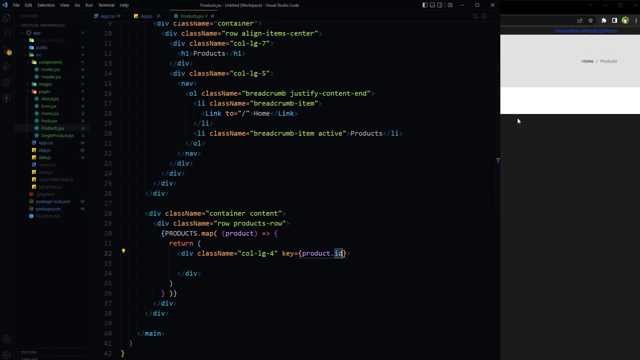 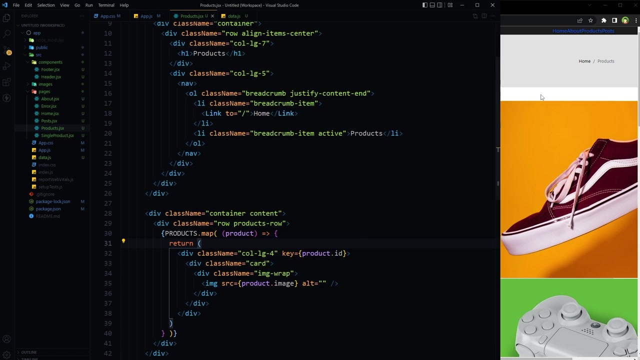 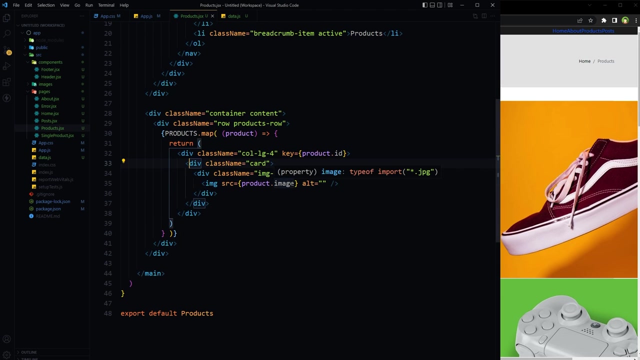 here and ID is this one. okay, now let's use card from bootstrap and then img wrap for the image: img, src, product, dot, image, art. so product from here and image this one, and we'll style these in a couple of minutes. so this is card and here we'll have card. 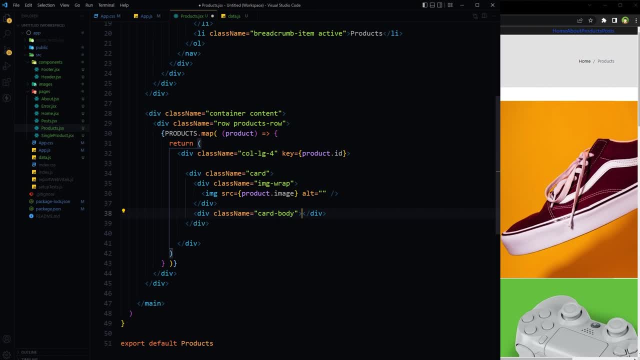 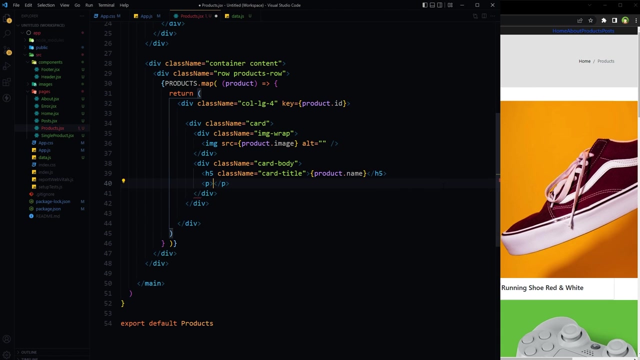 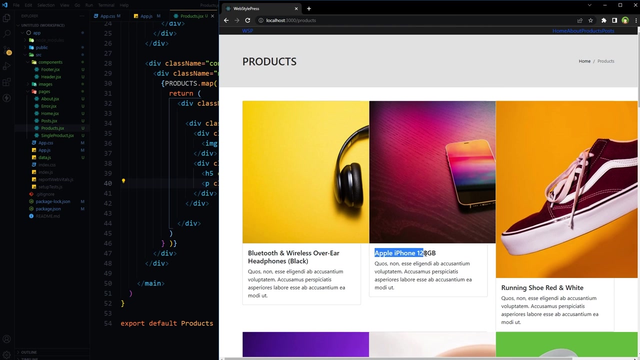 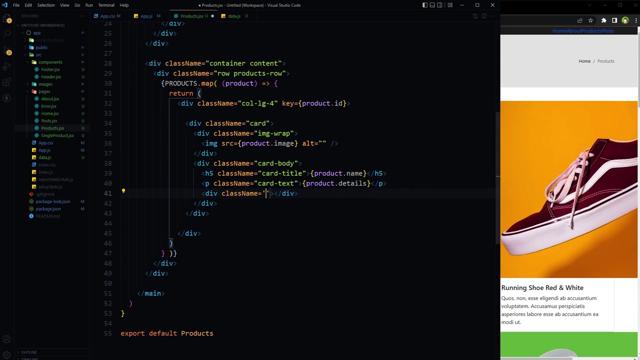 body H5: the card title, product name. this name paragraph product details, class will be card text save. and here we have got product title and product detail. after this, choose a div with class name display, flex, deflex- justify content between align items Center and here span and link. 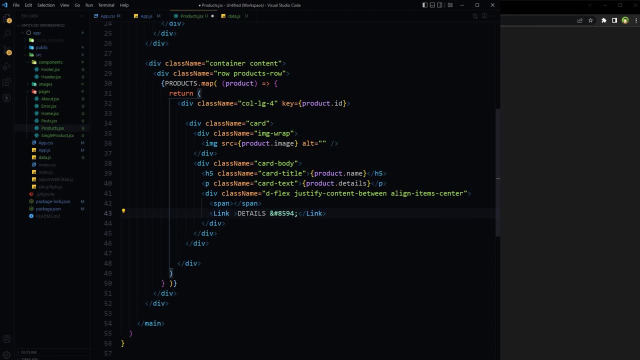 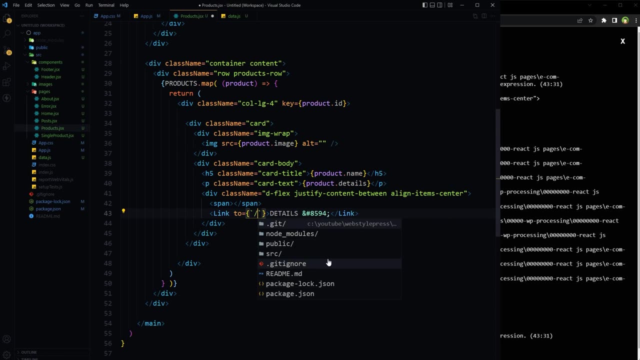 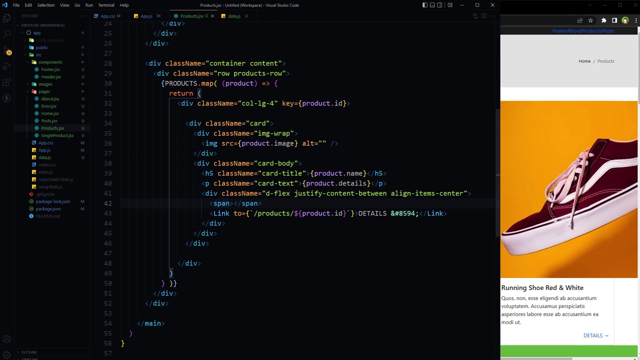 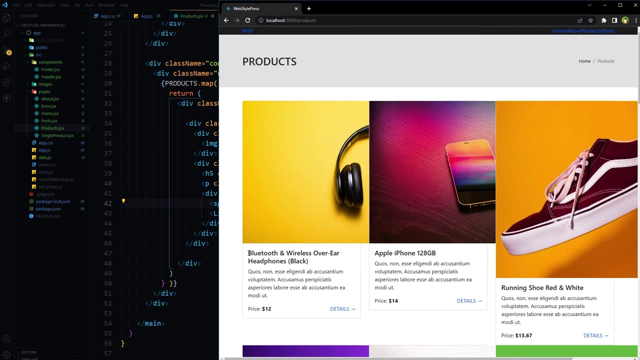 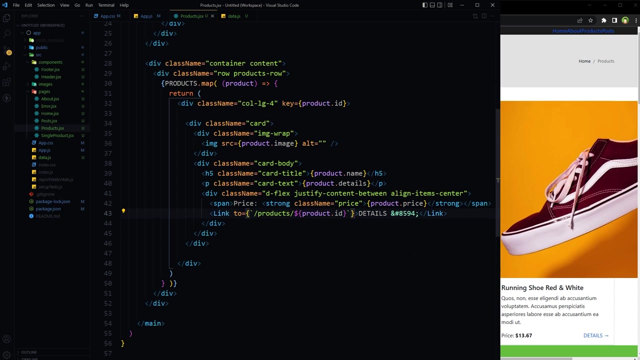 details link will have two attribute save. so here backticks, slash products, slash dollar sign, product dot ID: save. so here's our detail. and for span let's use price here price and product price. let's make bold, strong class name price. okay, so we have got title, description, price and details, and let's make it button. 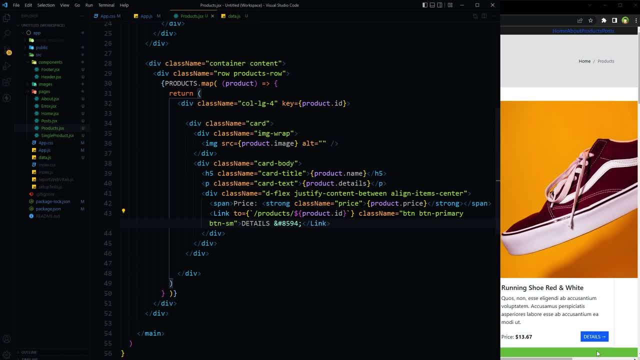 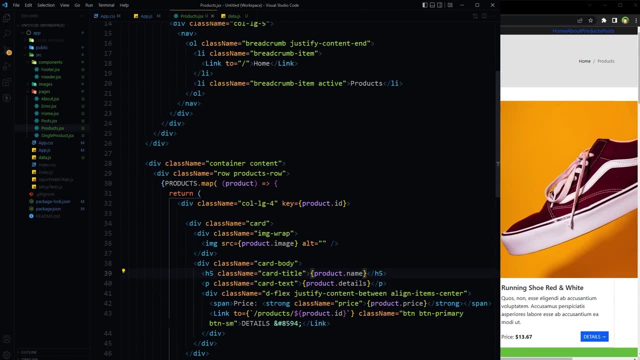 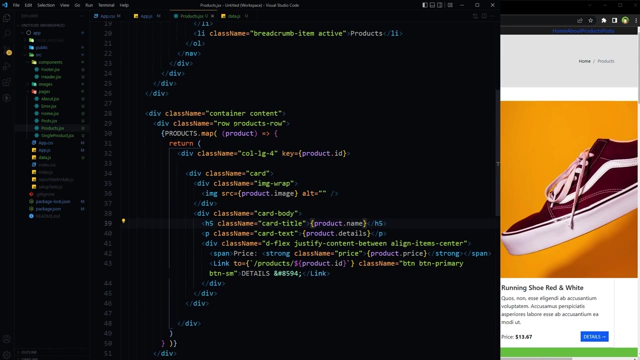 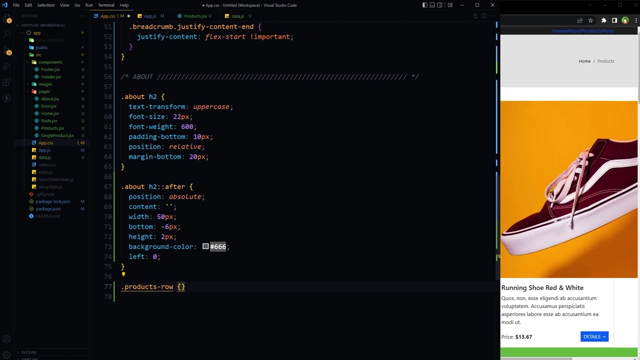 btn b10 primary and btn sm. okay, now let's style this page. we've got couple of new classes like products, Raw and a card IMG rep card text here: our products for extra card card to address mix and object возbrasil. i'm gonna change it to I'm a product wiv for CH and shout out to char Ortiz, John Roberts for productifen product raw card. wedding card card text held: God wrote for information your hadEnough. so we have for AND for products products law. the bno props are 한번. we have to define a third word again, or sometimes they will use also SB for transcribing products. Relax the products raw card. I'm sorry, okay. 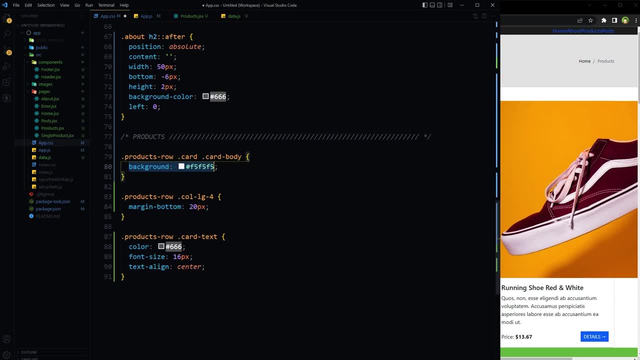 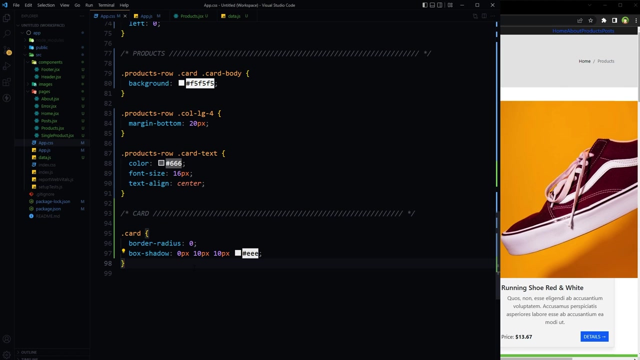 okay, okay, let's draw card card card text: it's fine, wait for business hair. I. card card body background color margin for the column card text style: save. and now styling for the card card will have border radius and box shadow looking much better now. card title style. 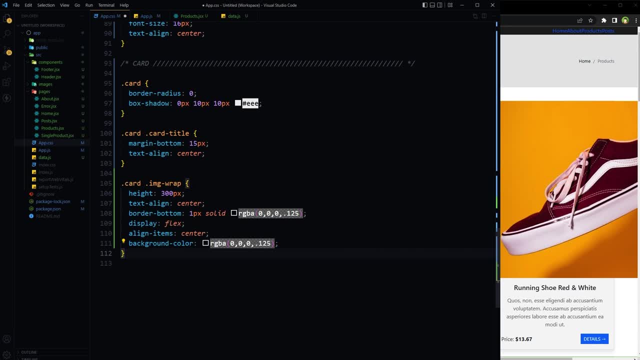 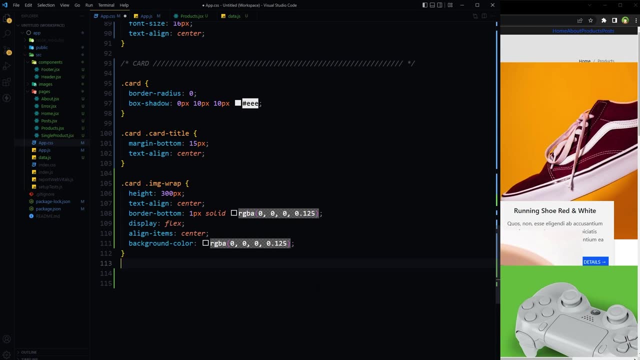 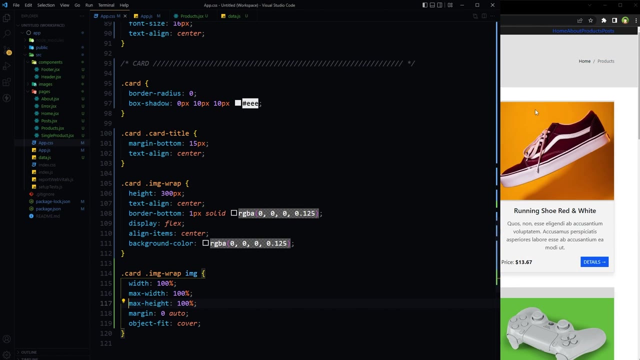 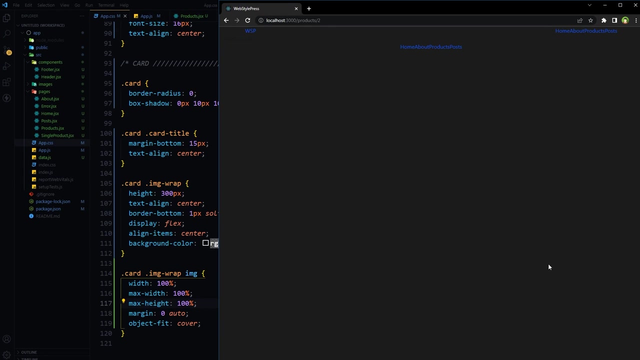 card image wrap and for the actual image with 100% max, with 100% save, say no, it is better, right. and if you go to details page we see this URL products and then ID for that product products and now ID is five products. that is because 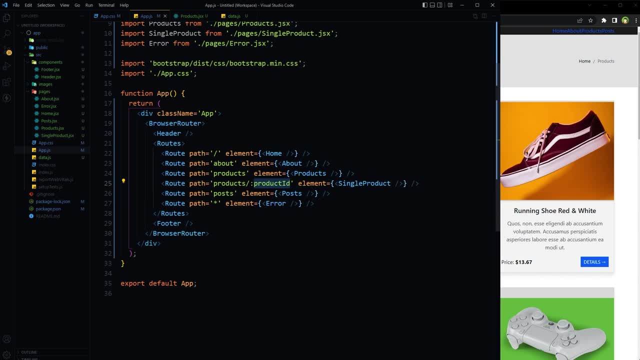 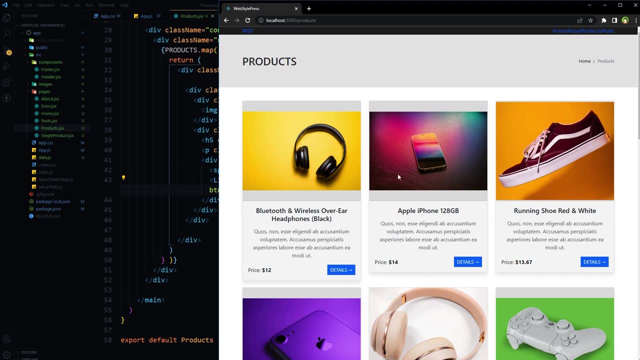 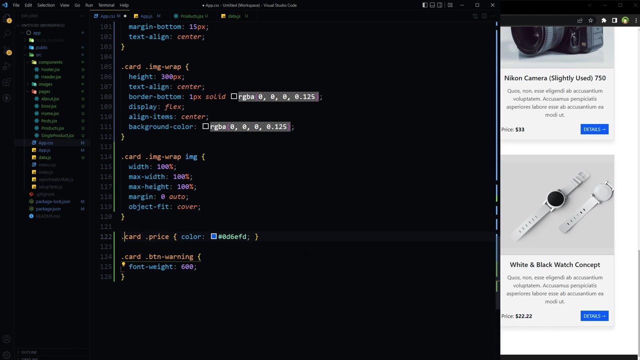 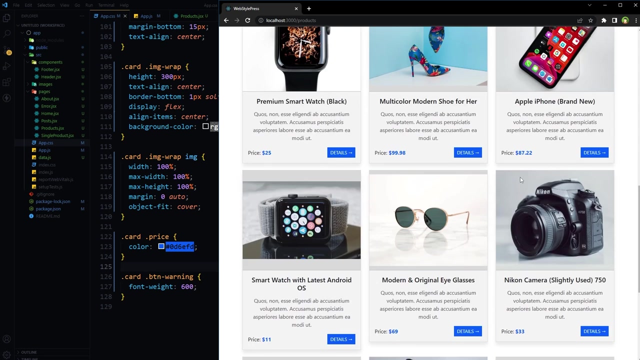 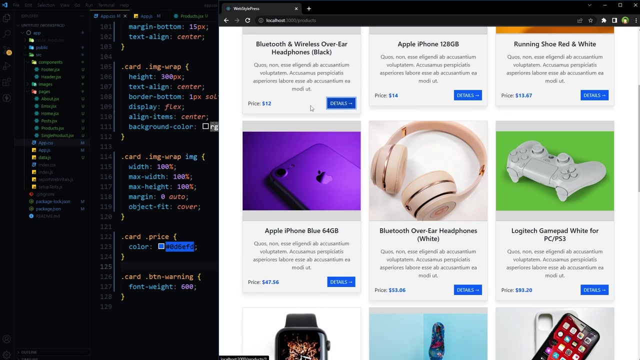 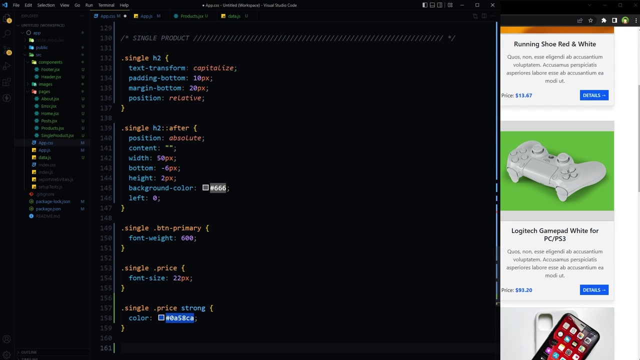 this configuration that we used here: product ID and here we are using this link. okay, looking much better, right and card price and card btn warning. this is even better. by the way, this is btn primary. yeah, we will also need styles for single product page, so these are here. 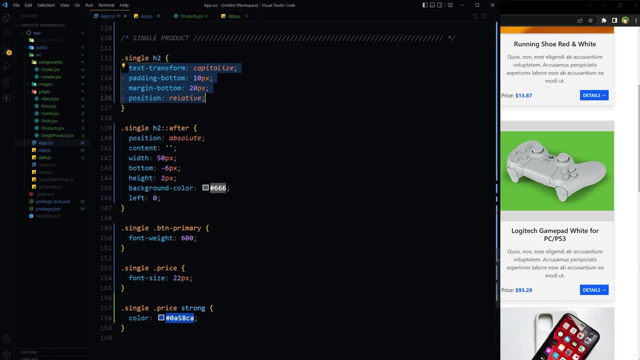 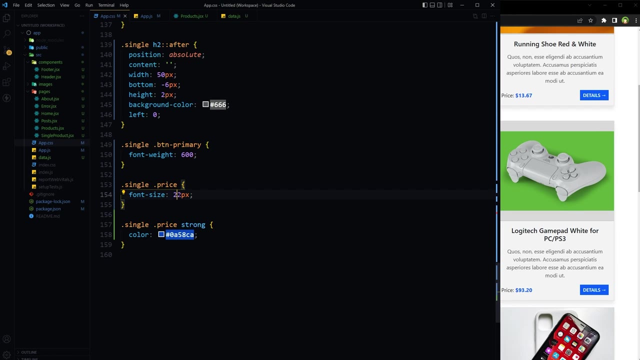 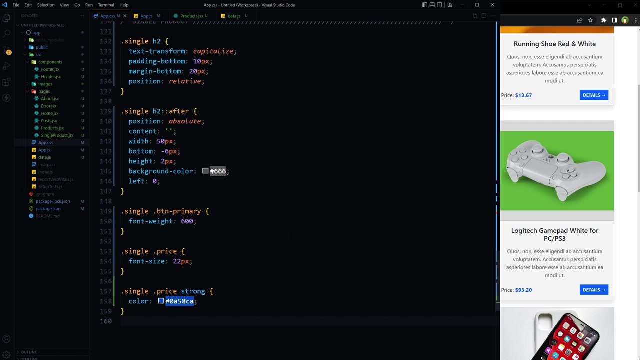 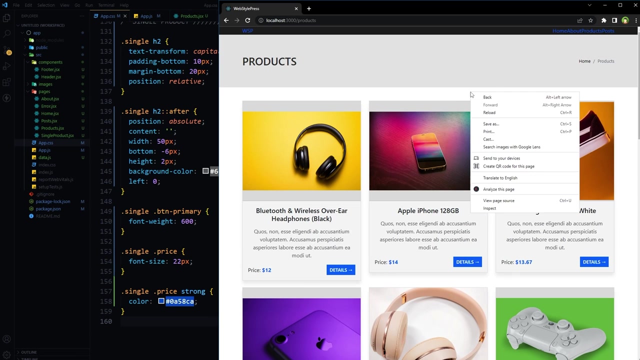 heading inside single div, these tiles, and then for headings, pseudo element that is after these tiles will have button at that page- and for price and simple styles. I'm basically not wasting time on styling the app and of course you'll get the code. you can understand it better by reviewing it yourself. my focus is on functionality, right, okay? 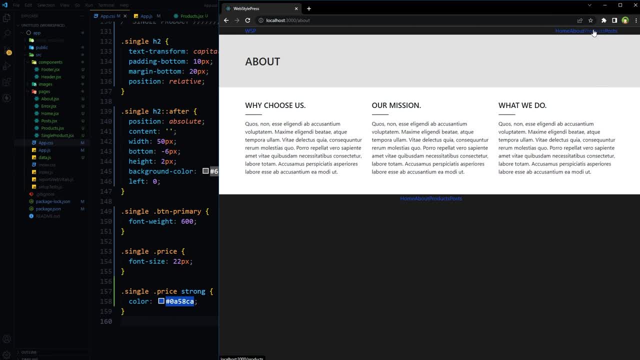 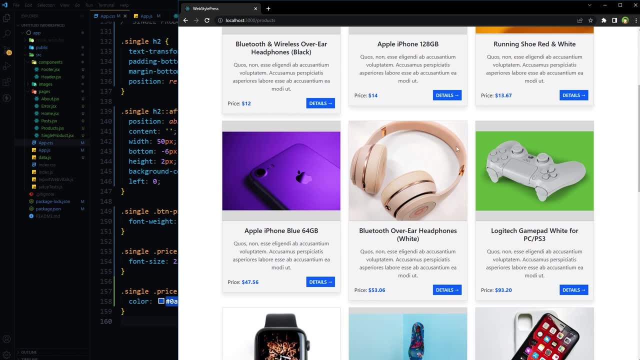 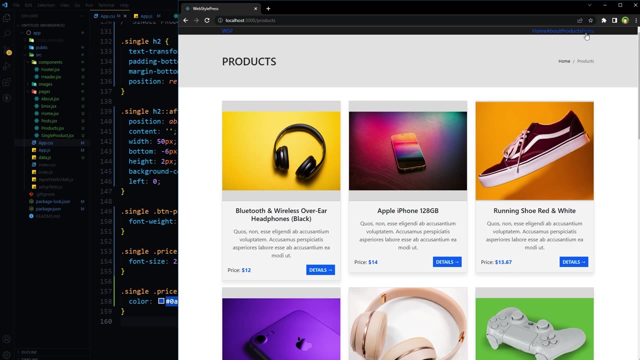 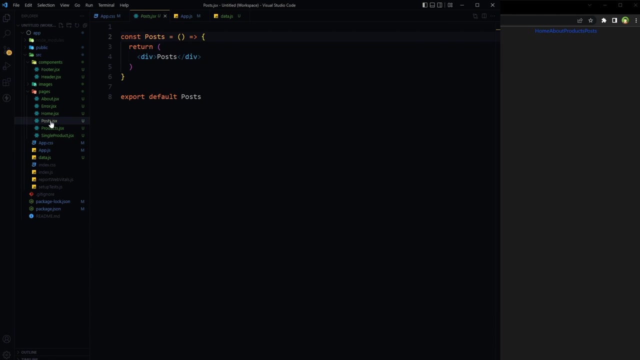 home about and it is responsive. let's start with sample this, but then it's readluable and then there is a function called this is needed. so device here, maybe not. here are some zombie code. here he is: serve the ads and page for the posts is this: 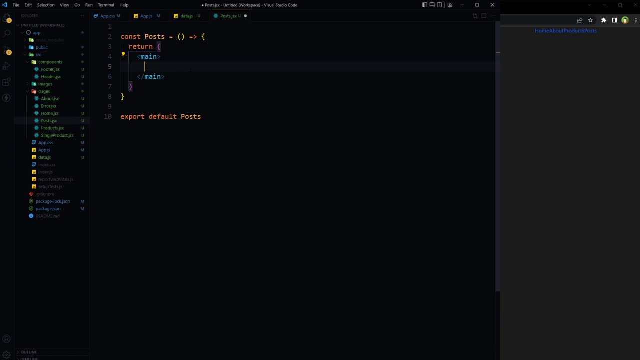 main man, because here we'll use hooks, use state and use effect and will need link from react router. dom class name posts: here let's have state const posts. set posts. use state and empty array: let's use another state loader: set loader: true. so this is a boolean value by default. 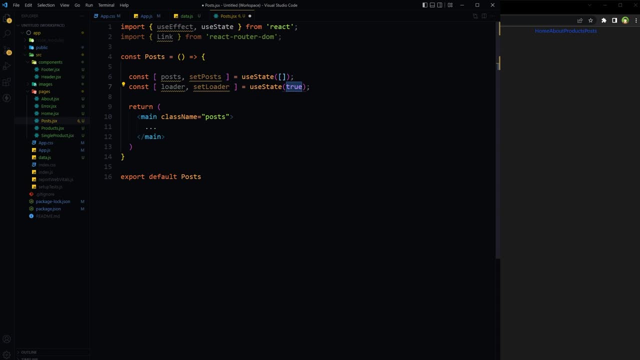 value for the loader will be true when the page will be loaded, or when the content will be loaded, or when po will have posts. then we will set loader to false and then we will show the content. so this is state and use. effect is here, and here let's use a function- fetch posts. and this is just a function, not defined yet. 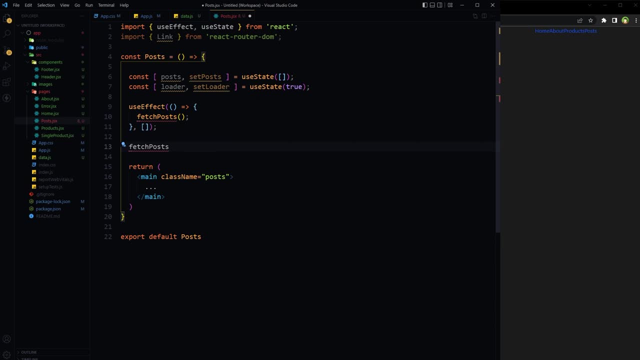 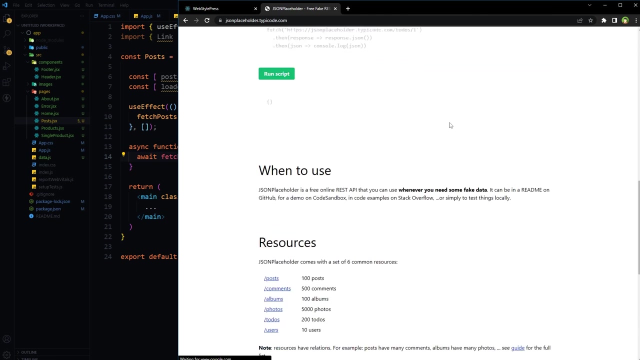 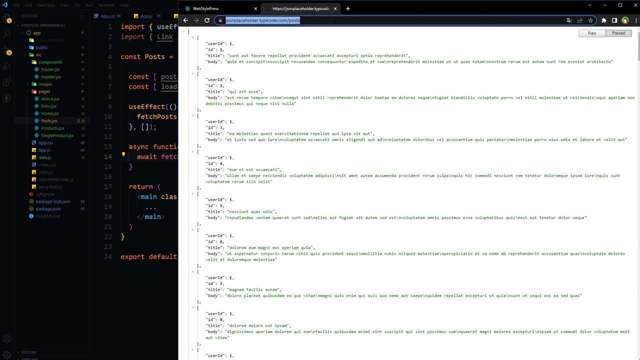 and here we will define it and we will fetch posts by using this function, but we will use async function. fetch posts, then await fetch. here will be the api url. how about json placeholder? json placeholder and we have got posts here: 100 posts, posts. this is the url that we are going to use here. 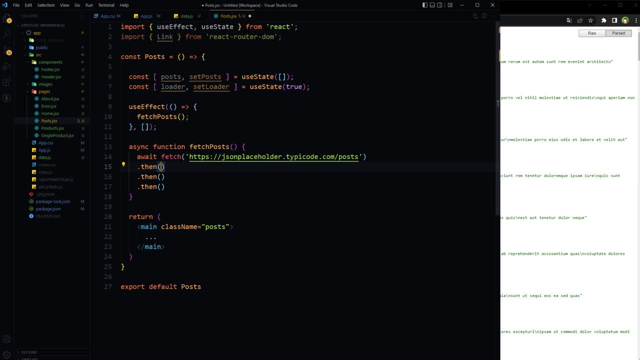 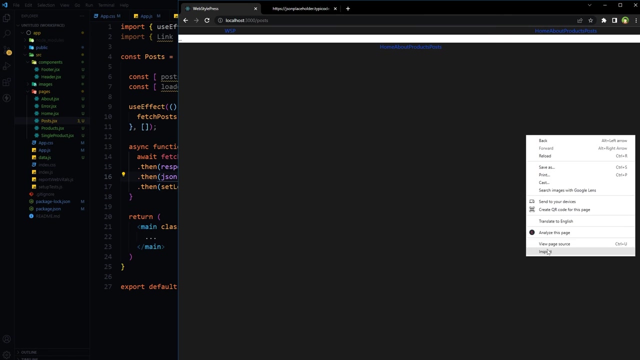 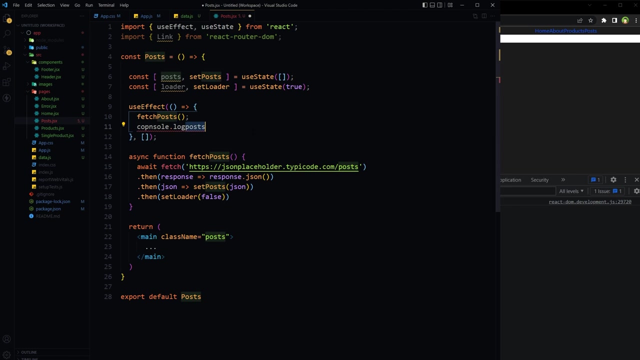 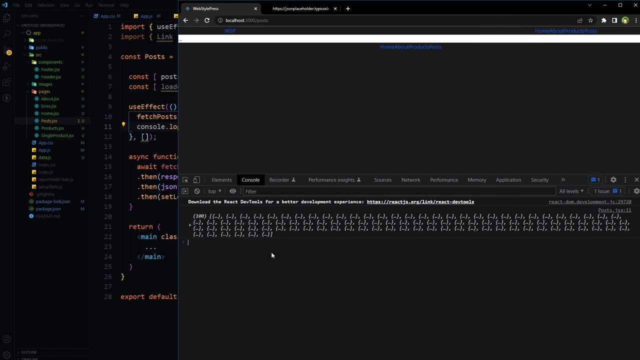 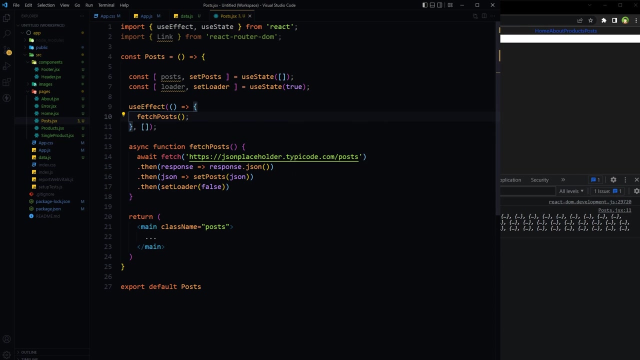 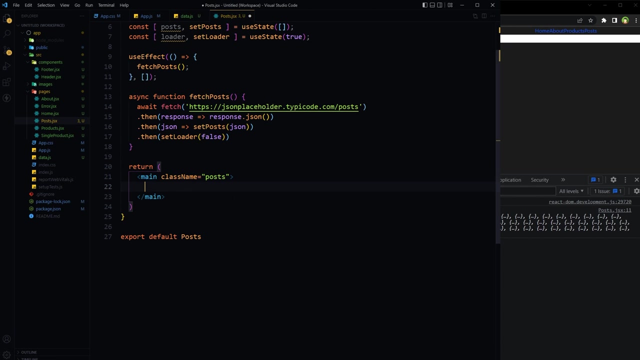 then, then then response: response: dot json and then json, and then json set posts. set posts json and then set loader to false right. so this is the logic. so console log, posts save, and here we have got 100 posts. okay, so now here we will display those posts, but first, as usual, we will use page header, pg header container. 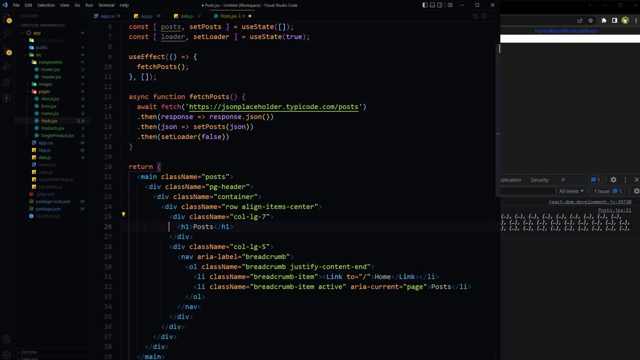 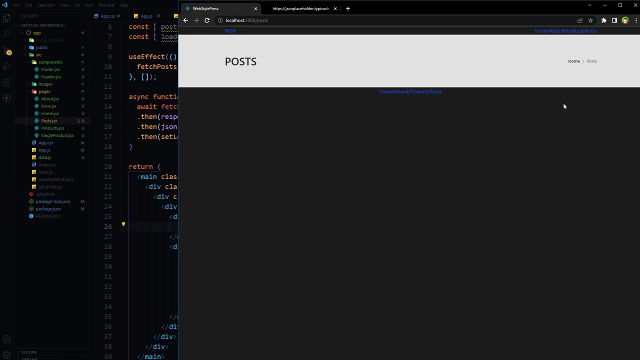 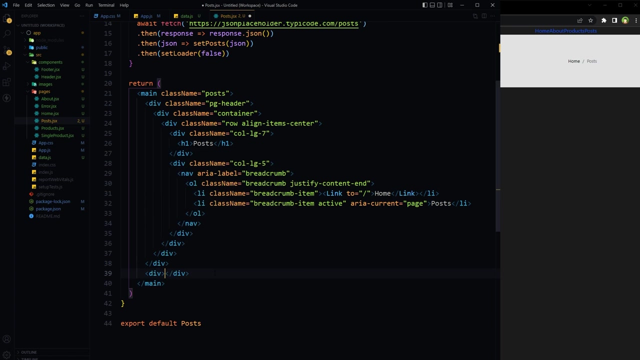 and inside we have got нал pg со heading with the text post and here we have got breadcrumb with class, breadcrumb justify content and and breadcrumb item link to home and simple text posts: save posts, home posts. okay, this was header below header will have content: class name. 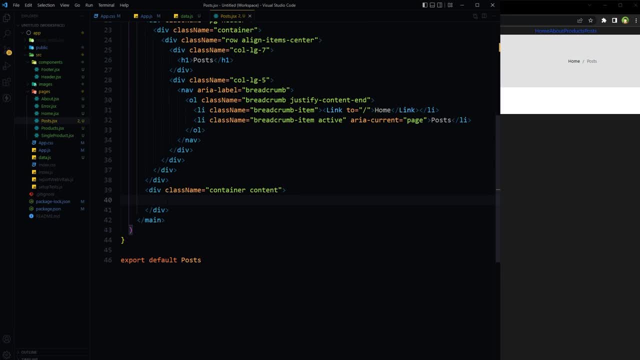 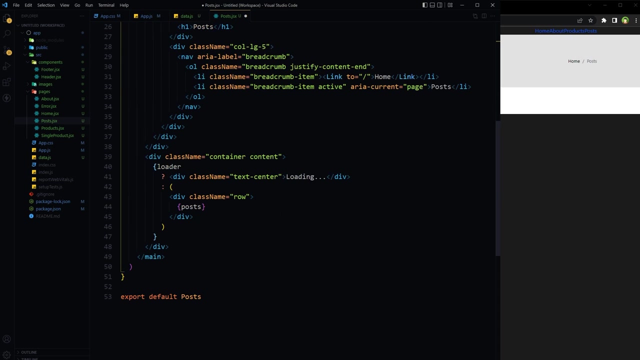 container content over here. if loader is true, then show this div with class name text center and with text loading. in other case or another scenario: return: display a raw, class name raw and inside raw will have posts from this state dot map post return and here column with class name, call sm6 and with key. 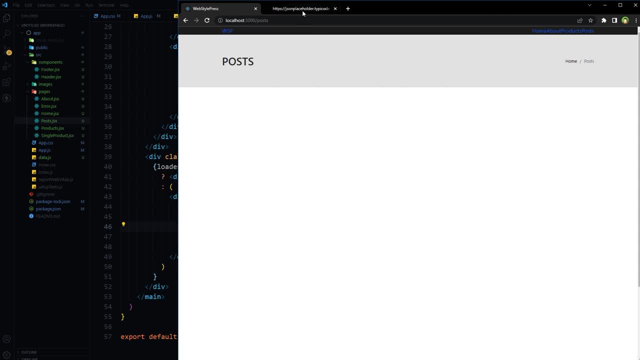 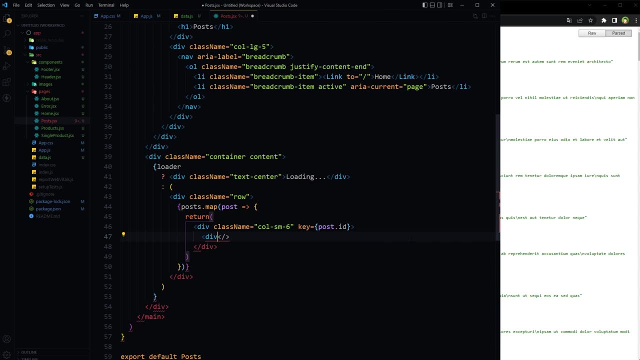 post id so you can see, here we have got id, title and body. so we'll again have card here. so we'll again have card here. so we'll again have card here. let's go over here: card card. we'll have card body. card body will have card title. let's make it heading h5. 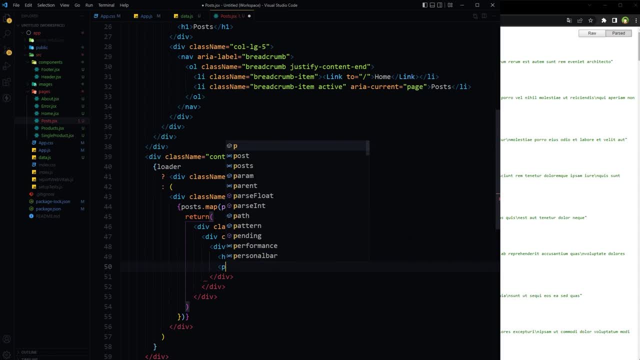 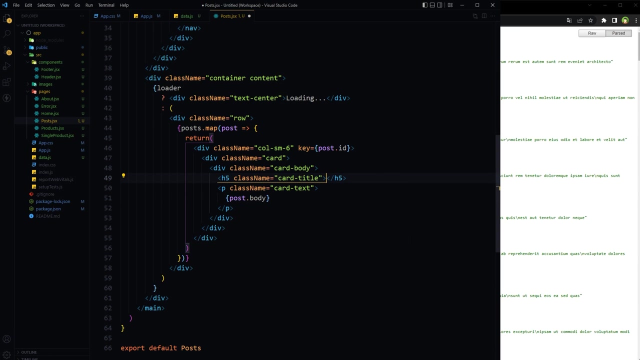 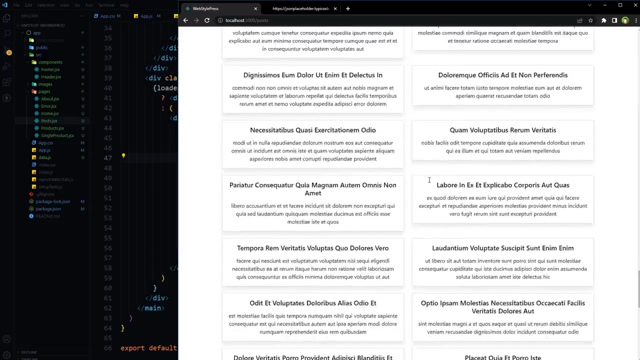 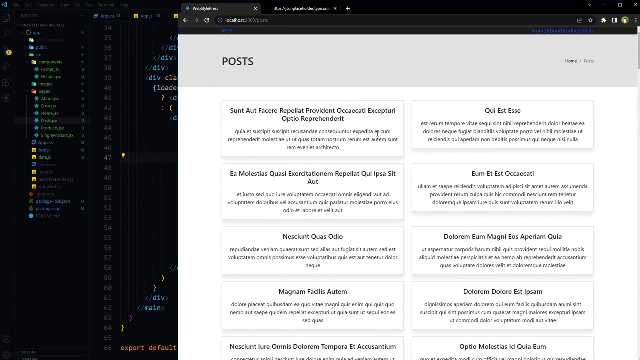 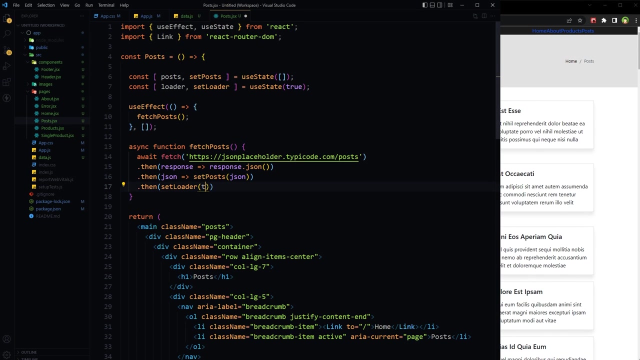 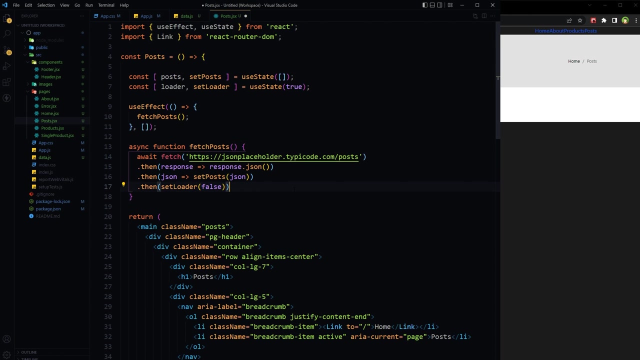 h5 and after that we'll have a small description with class name, car text, and here post body, post dot body and here post dot title, save and see we have got hundred posts listed here fresh. is that loading text? okay, if I make it true, then we see this loading text. so when this data will be loaded? 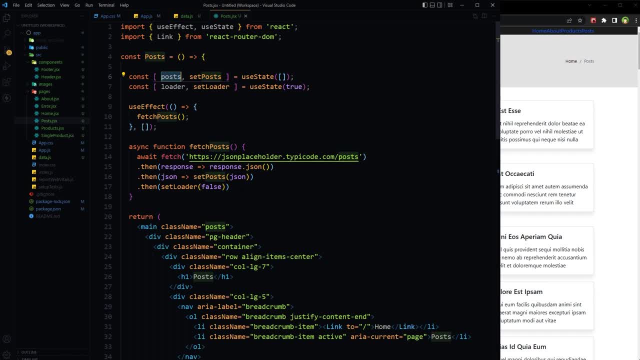 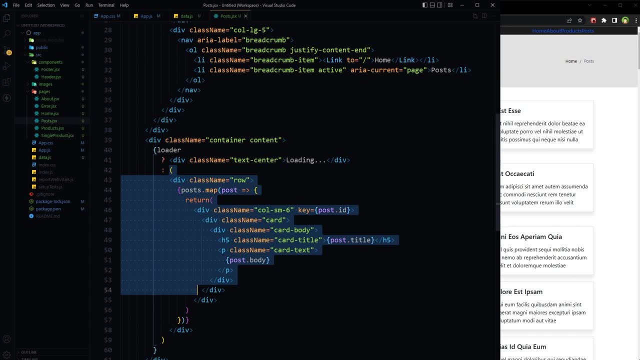 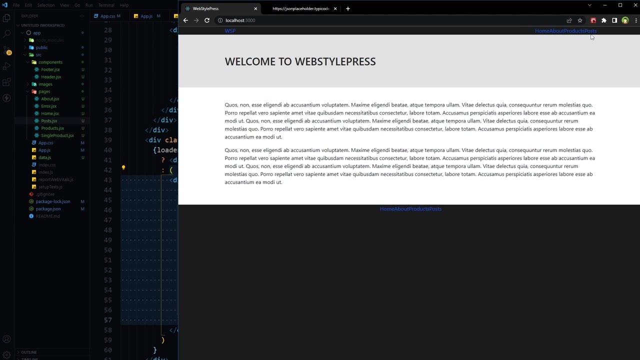 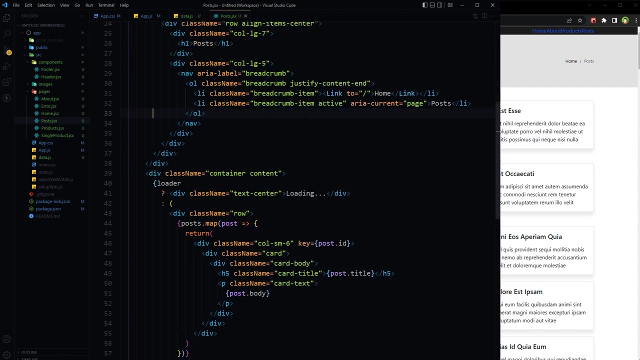 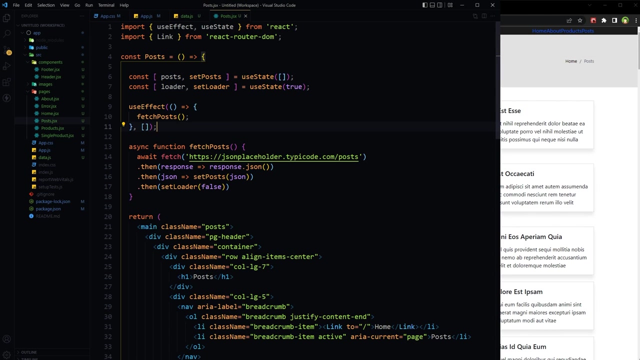 and saved in straight, then at the end then value for the loader will be false and then we'll save this data. so we've got the page for the post form posts products about home. so what we did here, we would use effect and use state and we fetched data and stored in state. but we did not do it in products and called data directly. 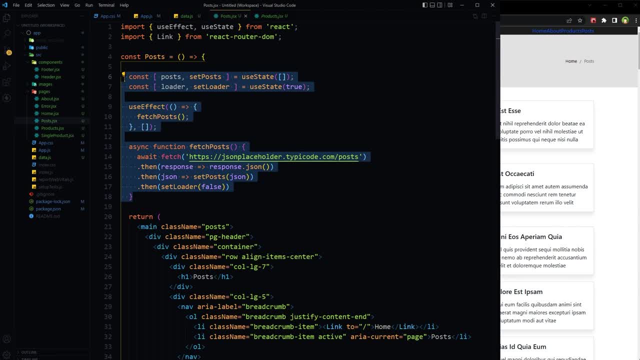 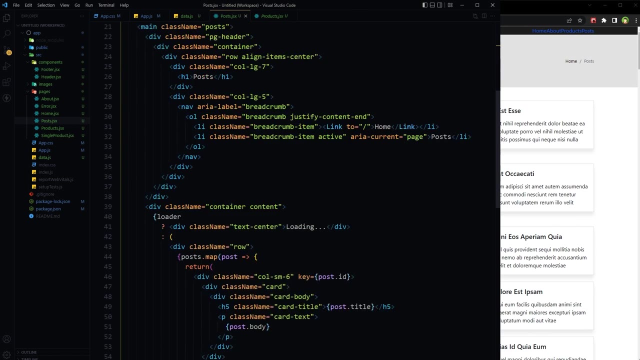 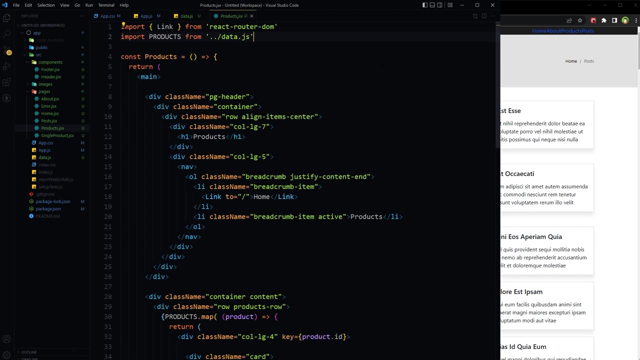 here. you can do similar thing that we did here with this data. it's up to you, but definitely better ways. this one, we'll come back to this in a minute, so all right. so we're going to type in a new, a new product and, as you can see the table, it will do this so that this is the product. so the first thing: 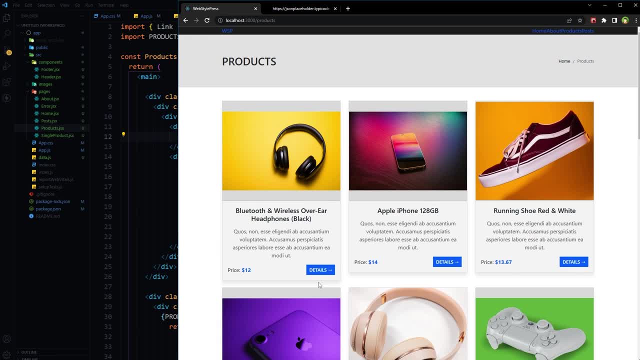 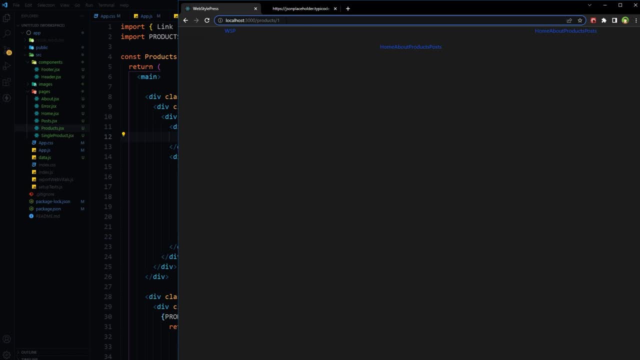 we're going to do is: this is what we're going to do is we're going to add a single line. you can change your name, so let's change it to say Monnie, Monnie, Monnie, Monnie, Monnie. and now let's change the name of this product. text: two elements, products, and then we are going to. 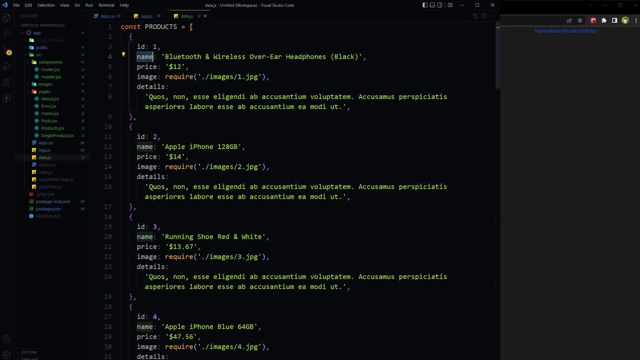 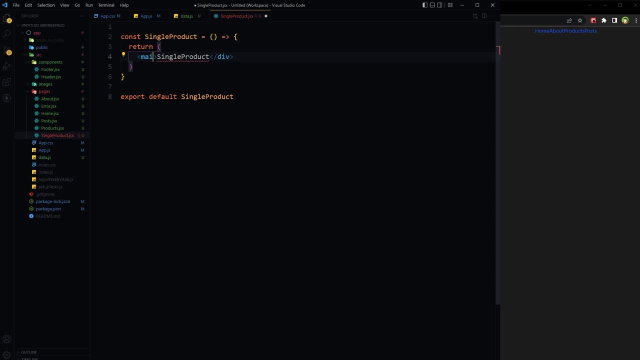 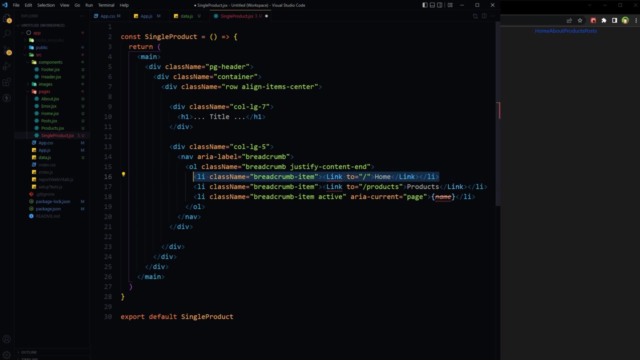 so single product page, is this one okay for single product, main header container, first column. inside it will have heading and well, for the data will have to fetch the data yet but let's use title here. and for the second column we have breadcrumb, the link to home, link to products, and page name will import link. 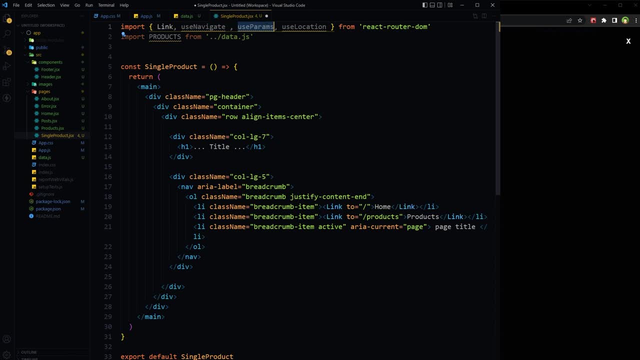 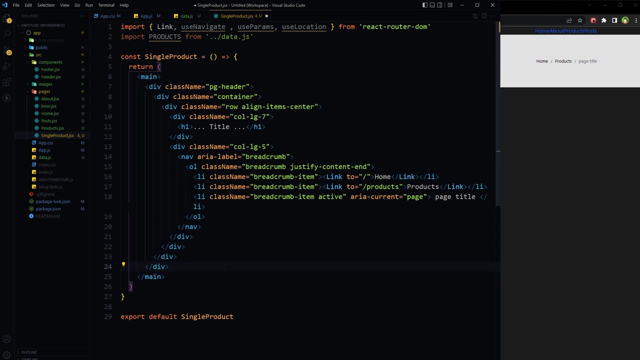 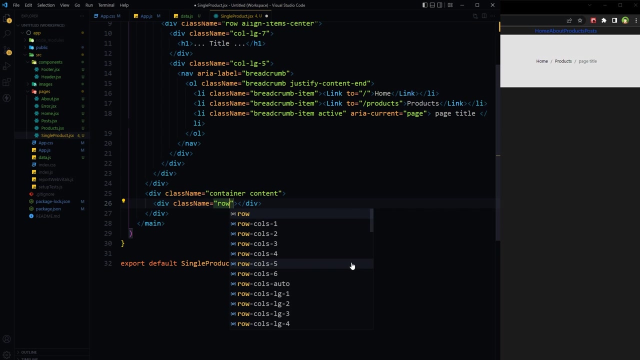 use navigate, use params, use location from react router, Dom, and will import data from datajs. this was the header and we have content for content: class name raw. inside raw, we'll have two columns call lg7 and call lg5, and here we will display image and here we'll have data. for the data we'll have product name. 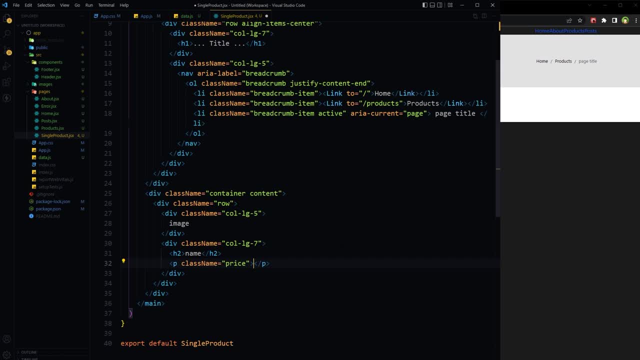 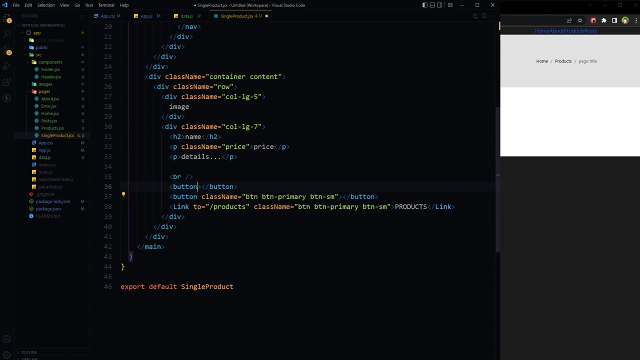 then we'll have price, then we'll have details for a single product, then let's use a break, line break, and then two buttons and one link link to products. products, let's make it look like button same, classes for button, same as for this button here we will use: back here: navigate to products. and for back we will use: 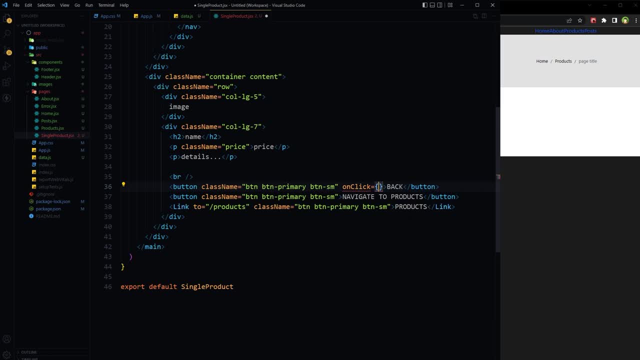 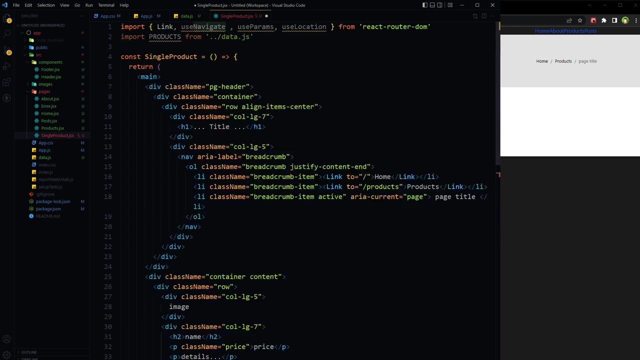 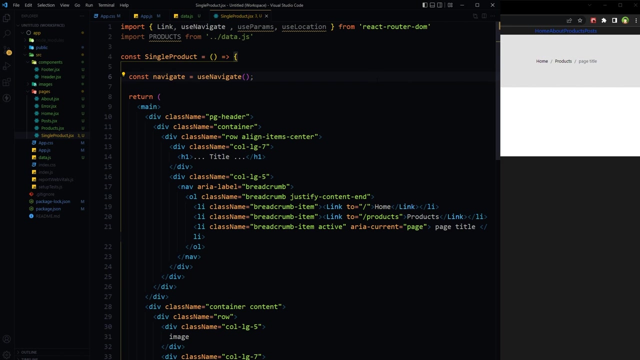 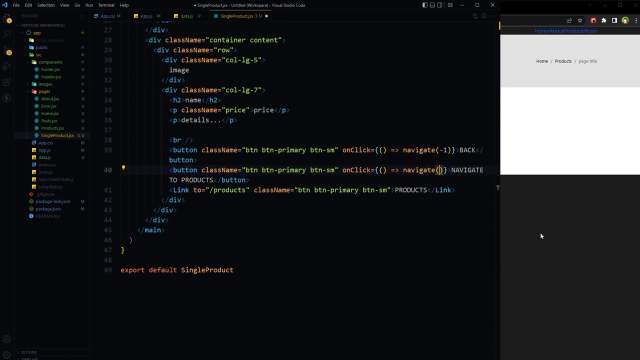 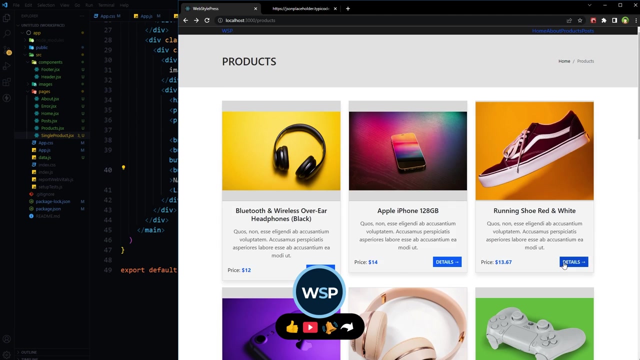 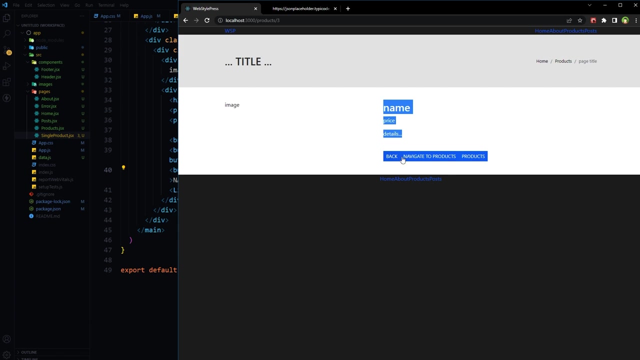 on click function. navigate minus one, one step back, and this navigate is here. cons navigate, use navigate and that's it. navigate to products on click. navigate products back details. navigate to products products. so these are different ways to navigate away from this page: navigate one step back. navigate to products by using navigate and. 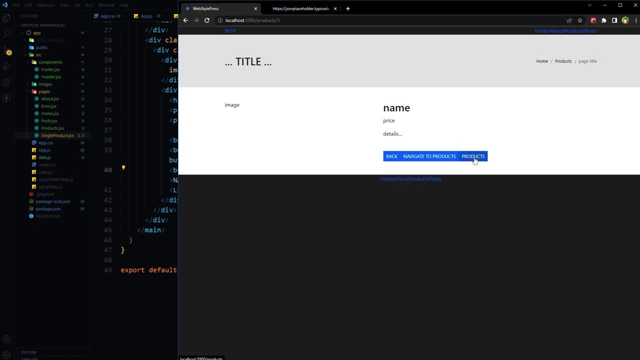 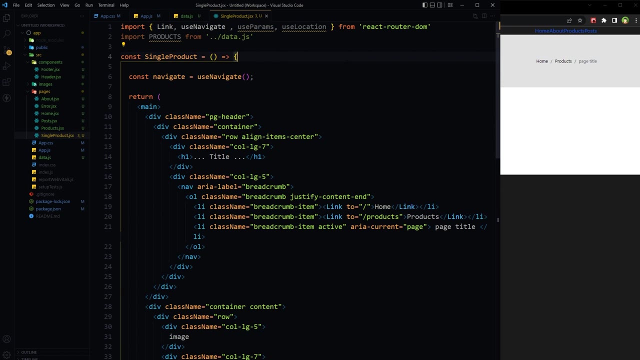 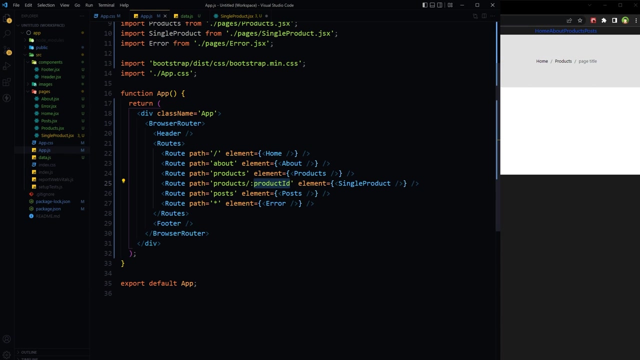 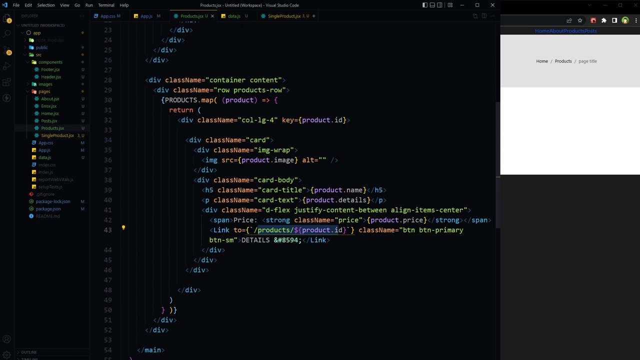 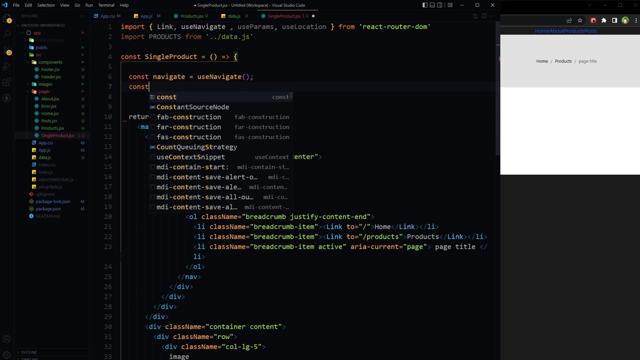 this is to navigate to products by using single link, just link. okay, so this is our page structure. now let's fetch actual data. let's get the product ID that we passed here: product ID, products, slash ID. basically, we are getting the product ID from URL. we'll use const. product ID equals, use parents. so let's get the product. 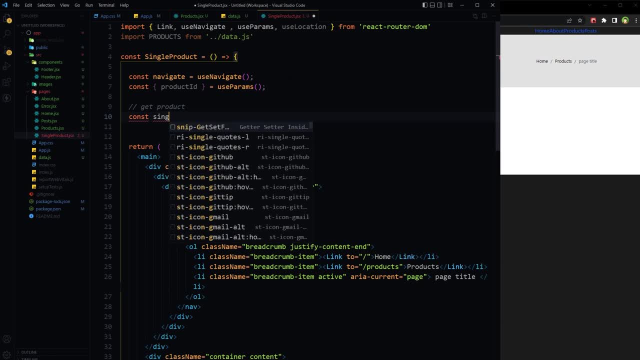 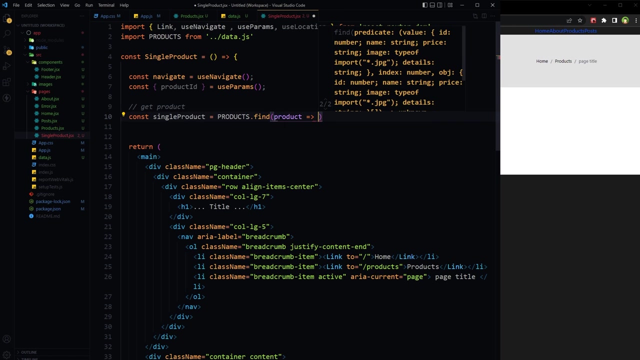 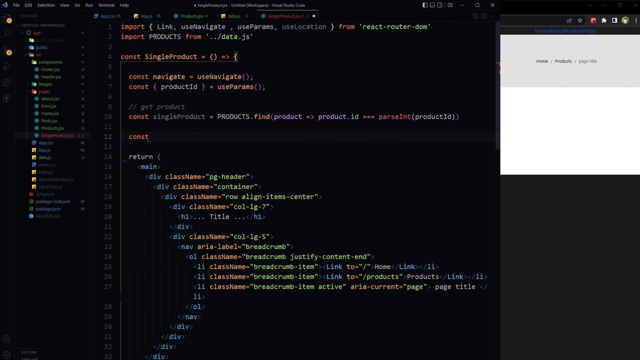 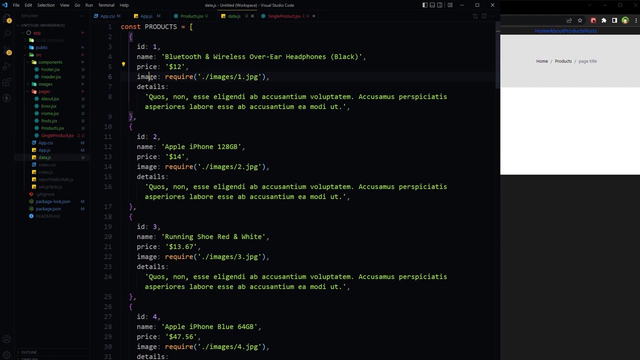 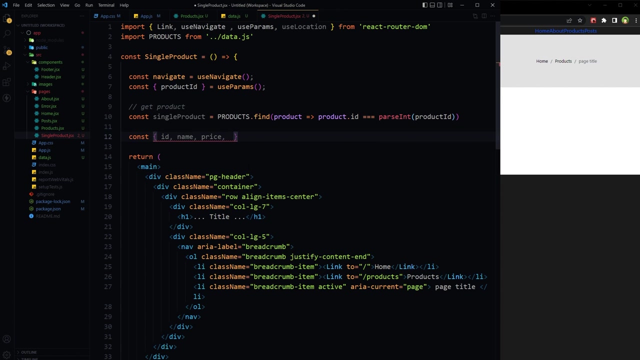 const single product equals. now we will get single product from this product. this data dot find product. product ID equals, parse int product ID and then const. let's de-structure the data like in this data. we have got ID, name, price, image details. so here ID name, price, image details equals single product. 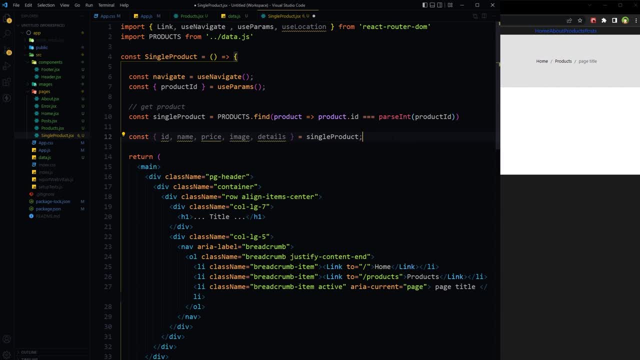 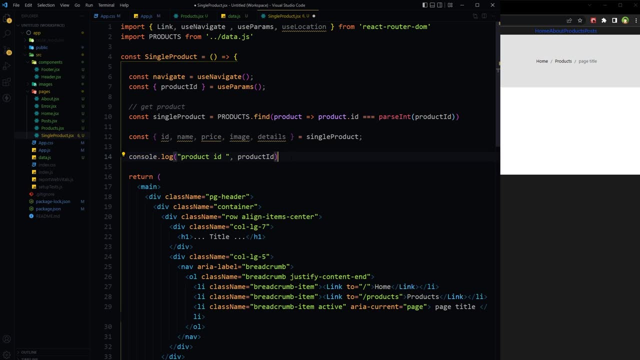 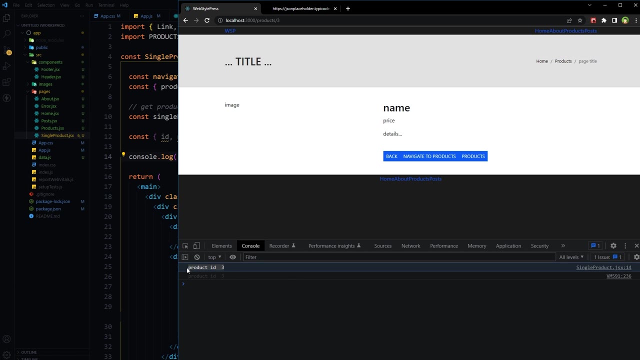 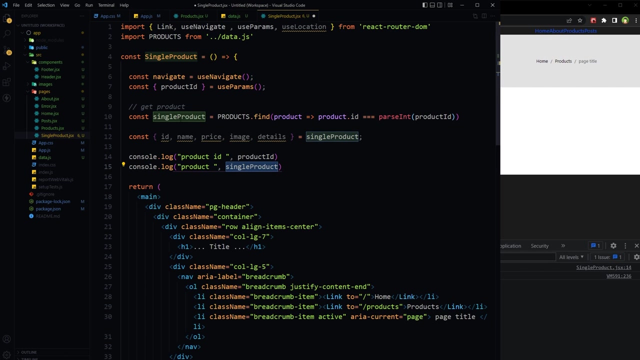 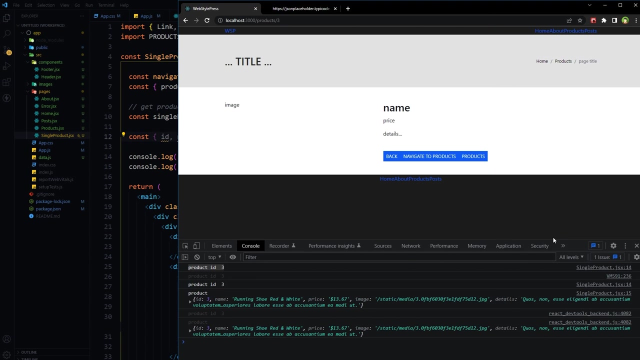 okay, so are we getting the product ID- this one, that's console log- and find out, save, inspect. yes, product ID 3. and are we getting single product console log, single product- this one. are we getting the single product save? yes, we are getting single product with ID 3. 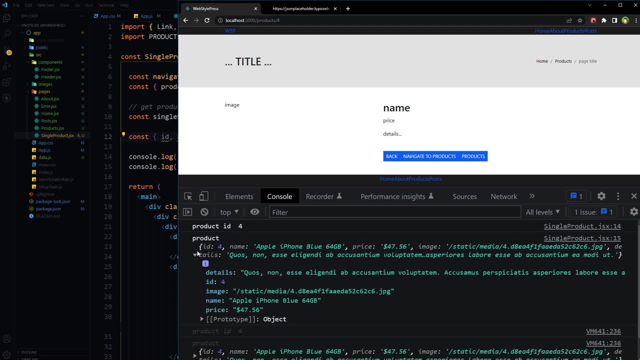 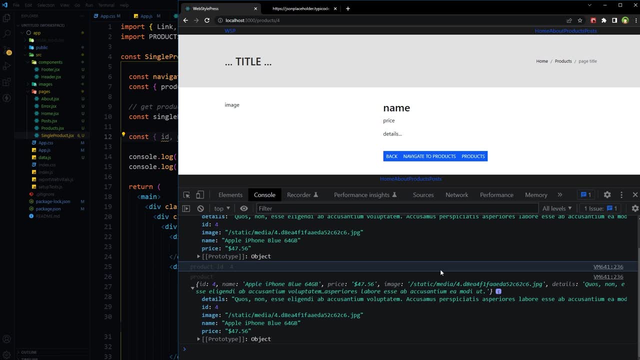 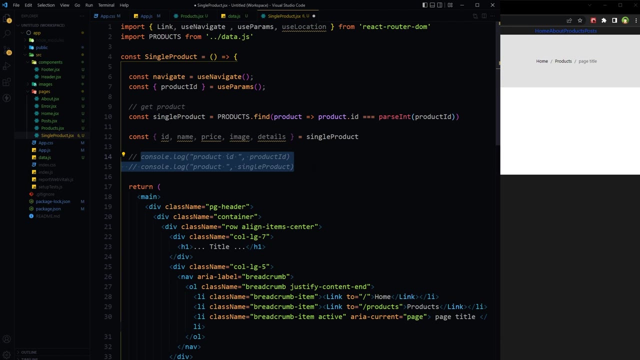 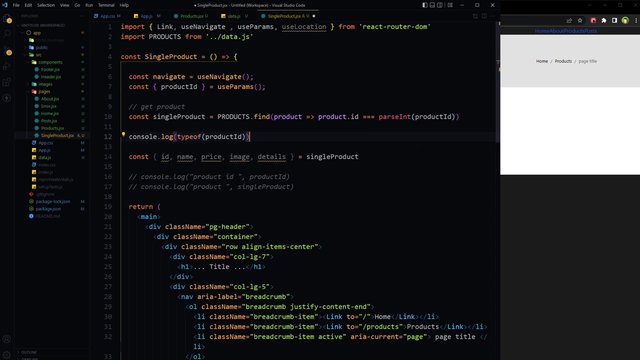 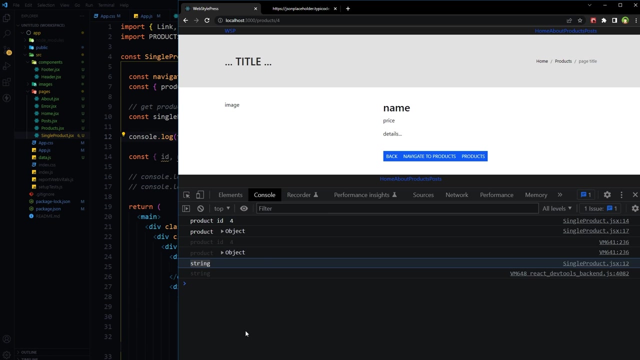 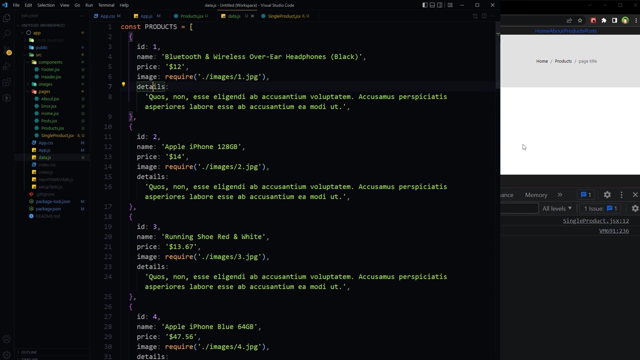 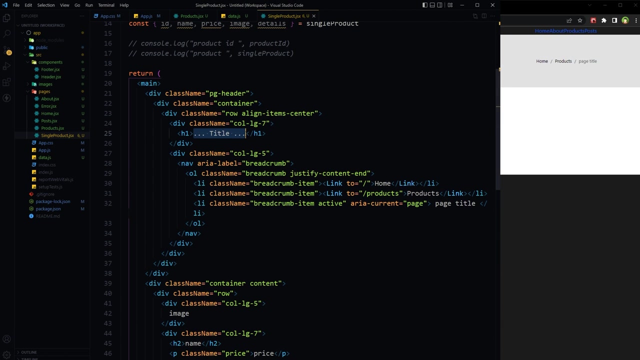 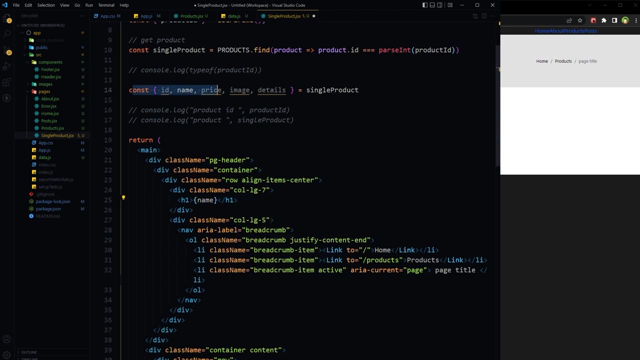 if I use 4, here we are getting this product with ID 4, right, okay? and the type of product ID is: let's console log string. okay, now let's call the data name, price, image details instead of this title. we have de-structured it, right here we have destructured it, so I've used name. 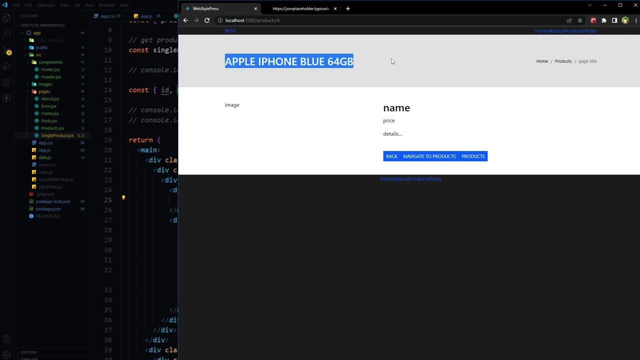 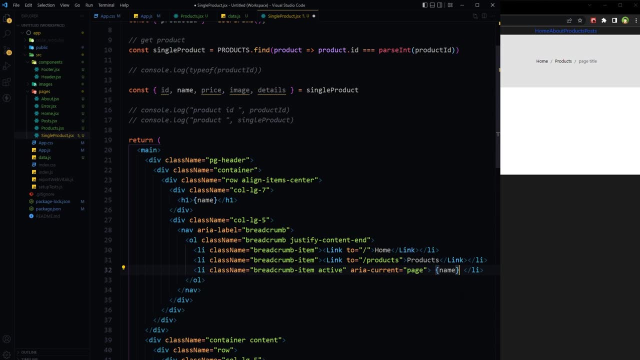 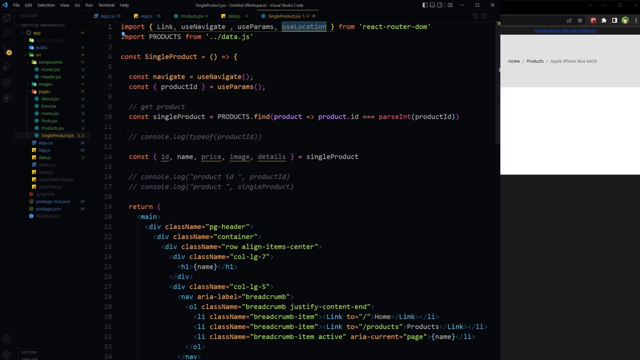 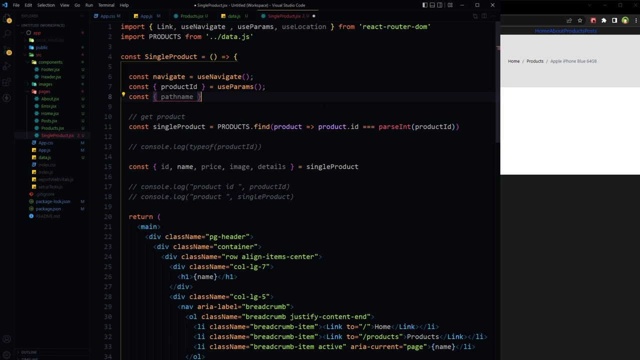 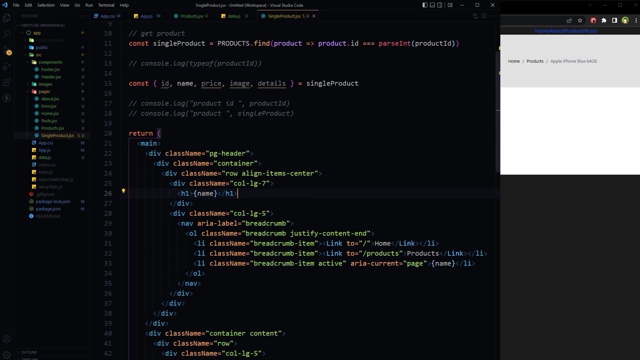 and name is Apple iPhone blow 64 GB and again we will use the same name here for breadcrumb. we have use location as well. we can use it like this: const: path name, use location and path name now can be used here as well if we really like to use it. path name. 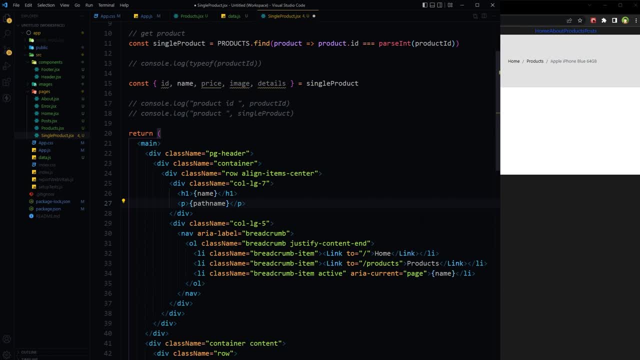 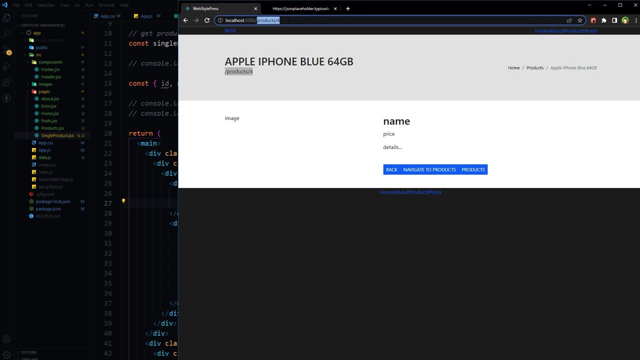 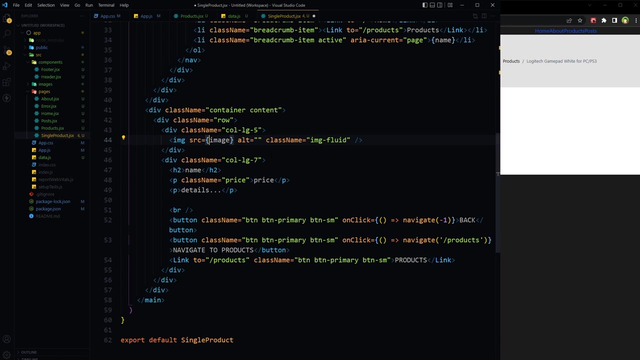 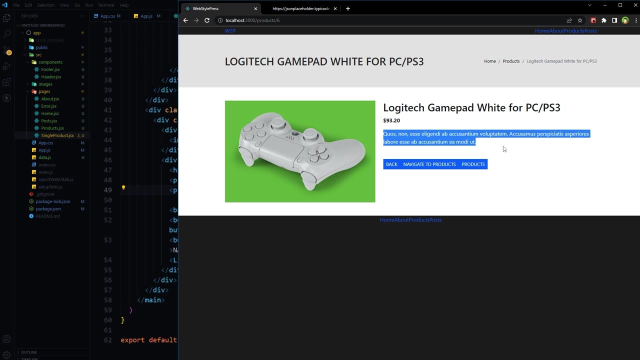 let's use paragraph here and you see this part. if you need this kind of path, products, slash 4, you can use it. use this: okay. products: product 6, ID6. okay for the image: image name, price- let's make it strong- and for the details. so we have got the image, we have got the details, you have got price, we have got title and everything. 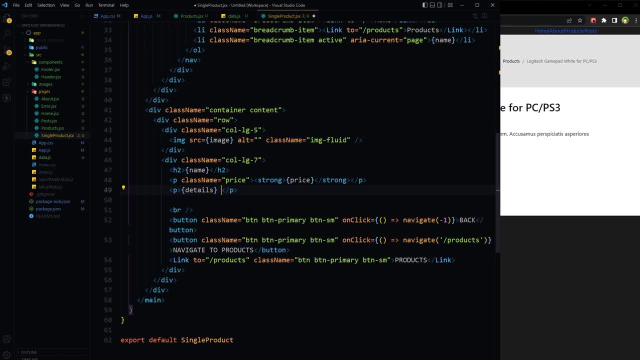 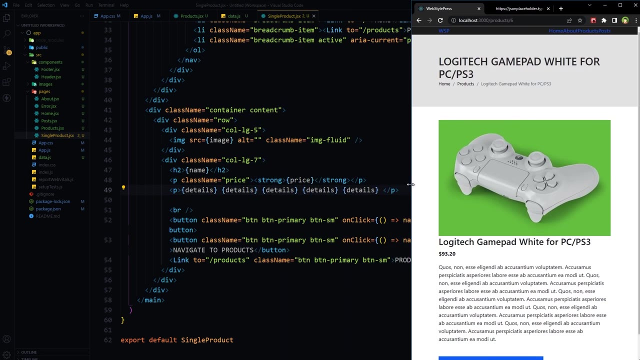 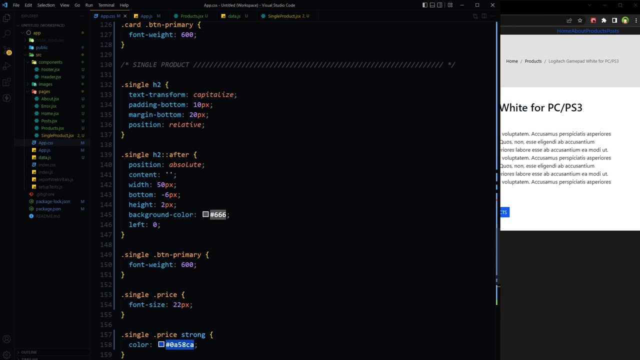 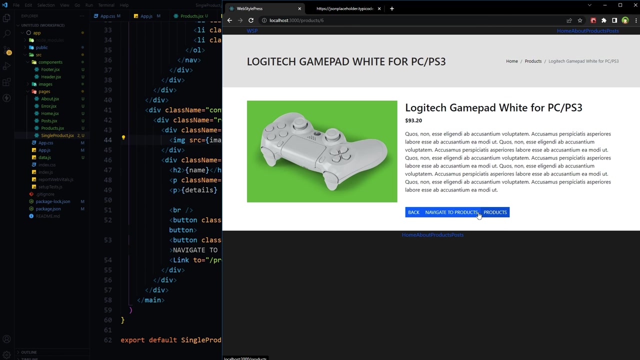 let's make this. let's make some copies of the detail for the product to just show the data. yeah, like this. okay, for the single product, we have got some styles. yeah, we have already used here the styles, so we are fine. so single product is also done. 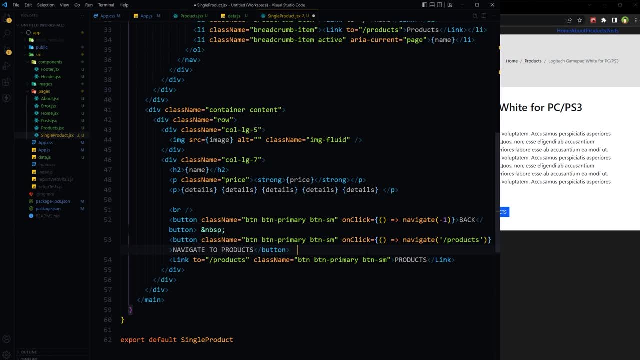 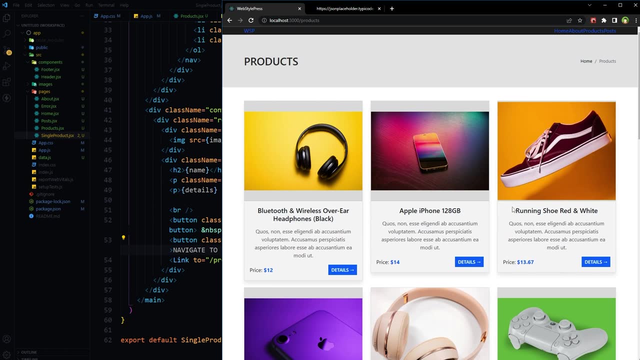 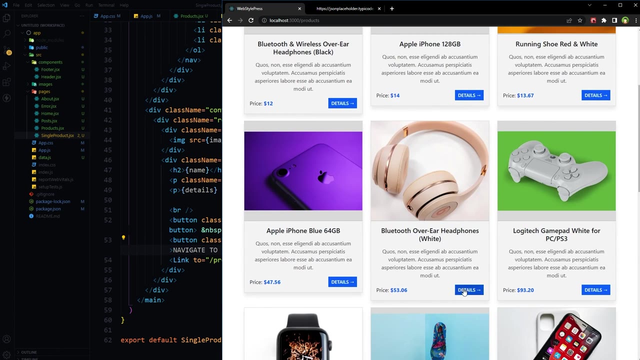 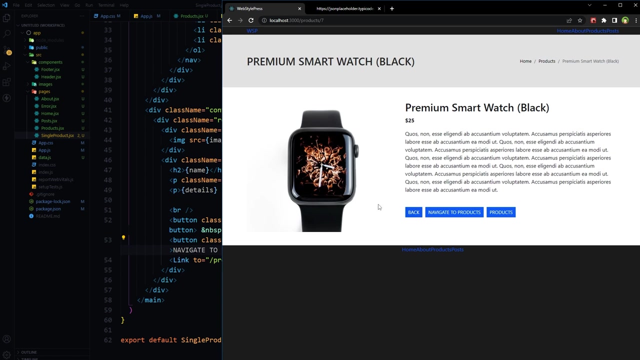 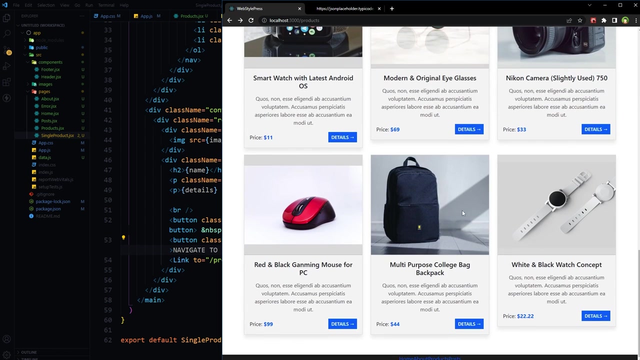 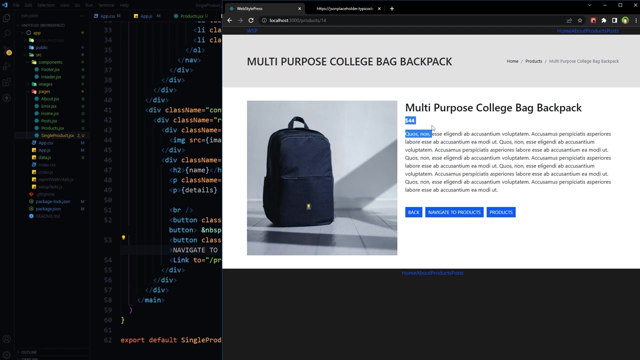 I want a little space here after these buttons, so this is better navigate to products and let's see this running show products. let's see this headphone back. let's use these- uh, this watch. let's use this. backpack price: 44 details is 44. multiple college bag backpack details. 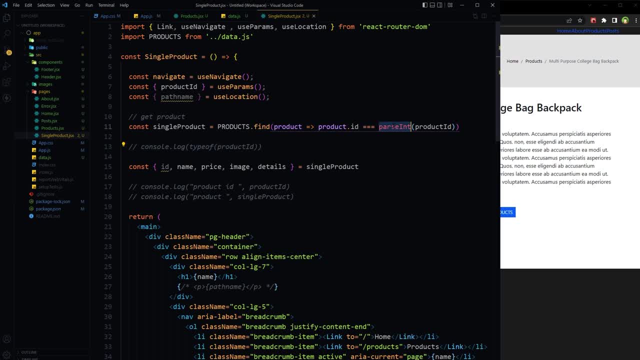 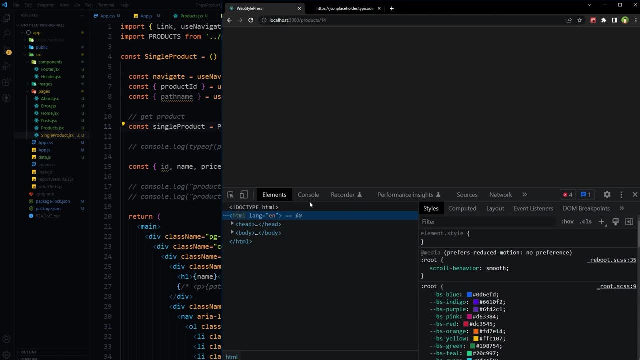 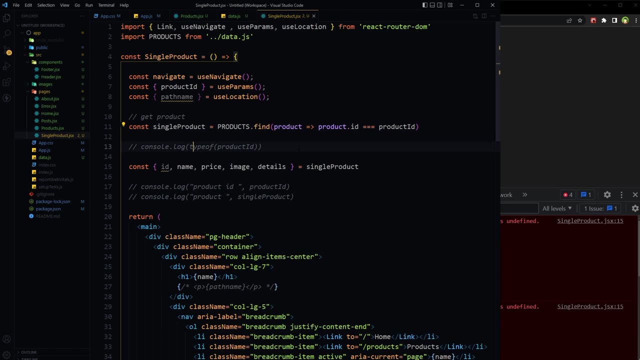 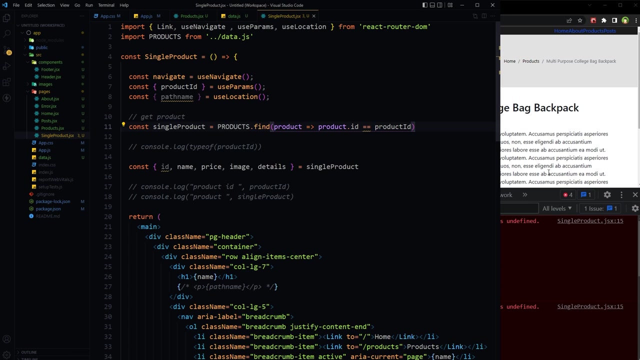 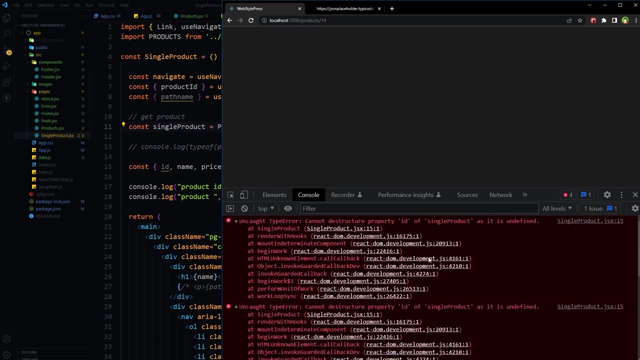 and everything is fine. so I have used bars in here. if I don't use it here, we'll have problem. you cannot destructure property ID of single product as it is undefined. but if I change this equal sign to this, then we'll see this product ID 14. if I change the equal sign, then reload. we don't have product ID, so that is why. 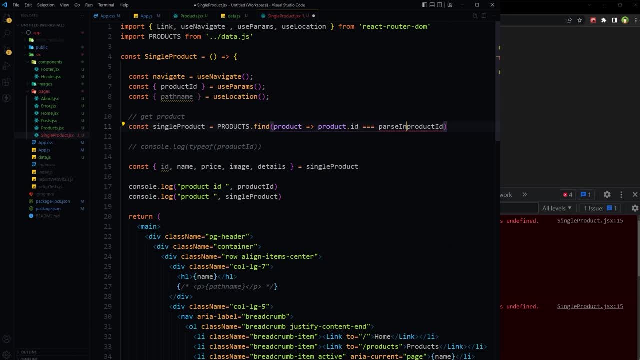 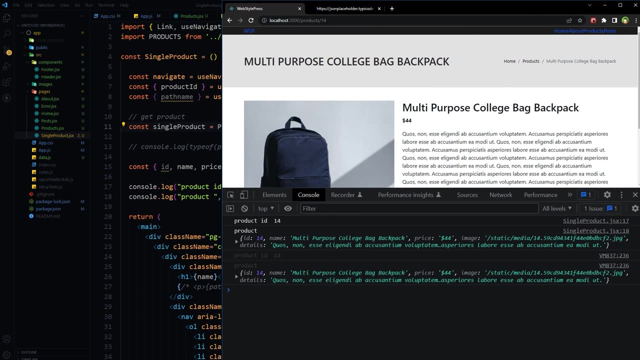 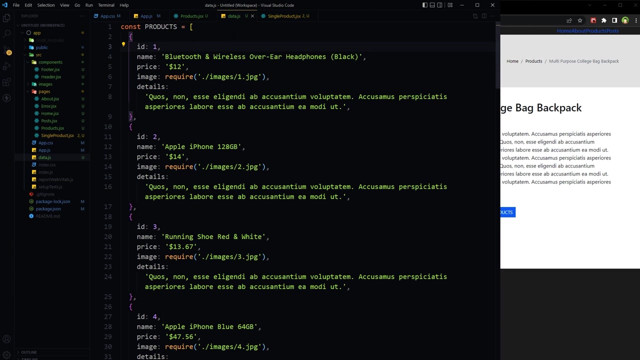 I'm, I was using powers and here, so that is why I'm, I was using powers and here, so that is why I'm I was using powers and here reload. now we have got it, so make sure you check these things. data type: that is because in our datajs file- and this is datajs file- it could have been JSON file as well. so here we have. 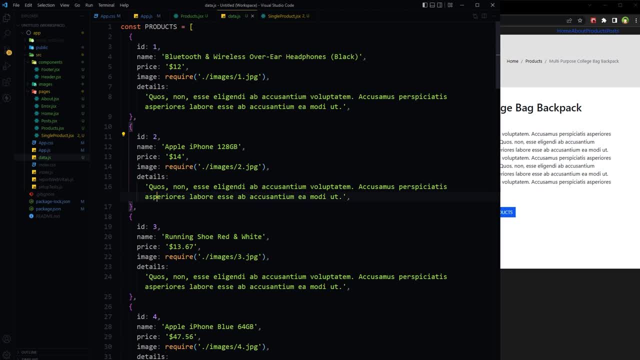 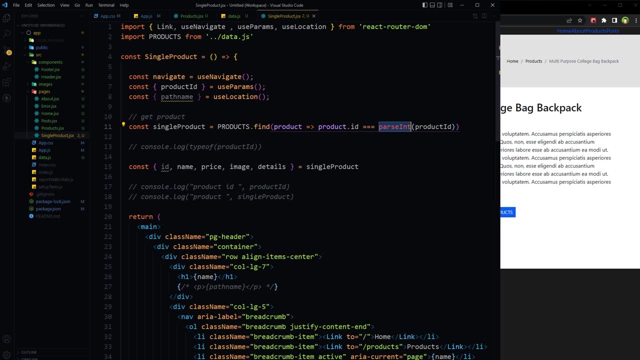 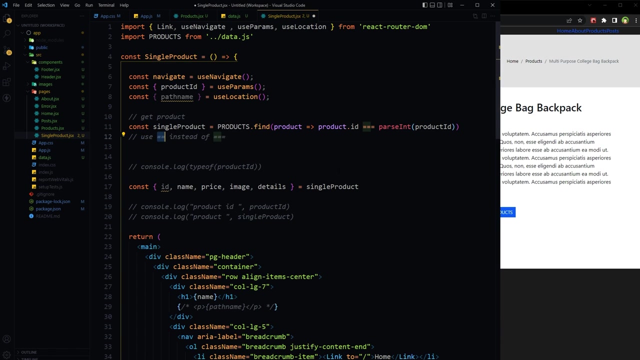 got one. this is number, so make sure you check data type and use parse in here, or change or adjust this sign if you're getting error. in case you are not getting product ID from use params, let me just type it here: use equal, equal instead of equal, equal, equal if use params fails to get the id. 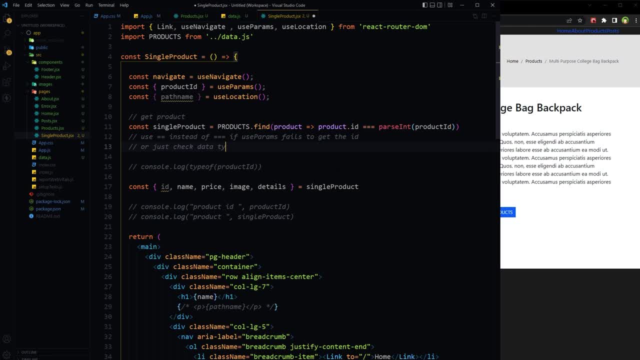 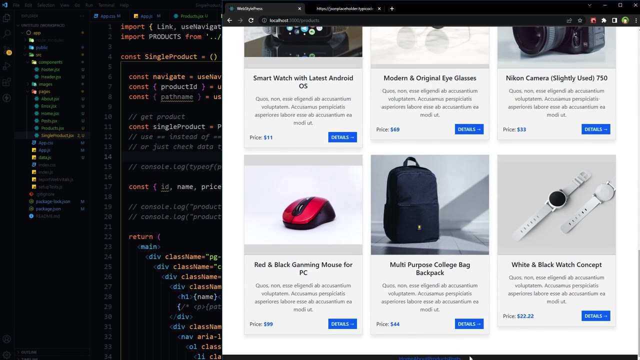 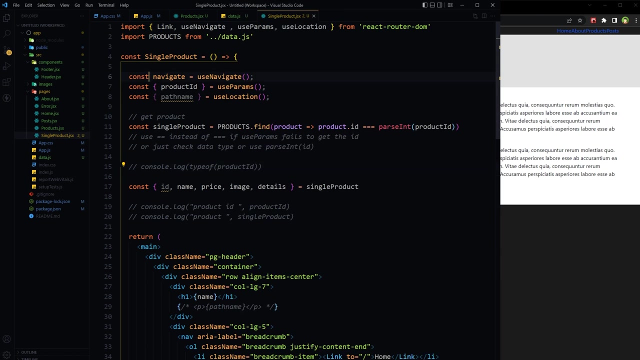 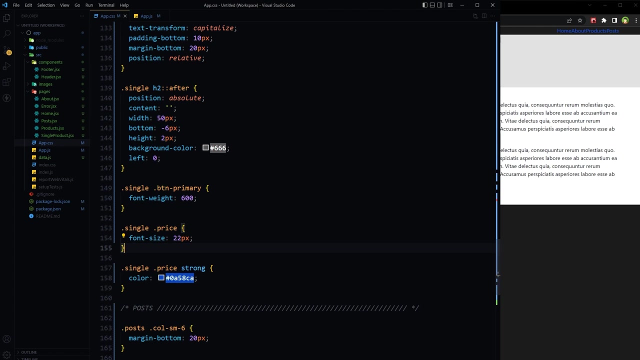 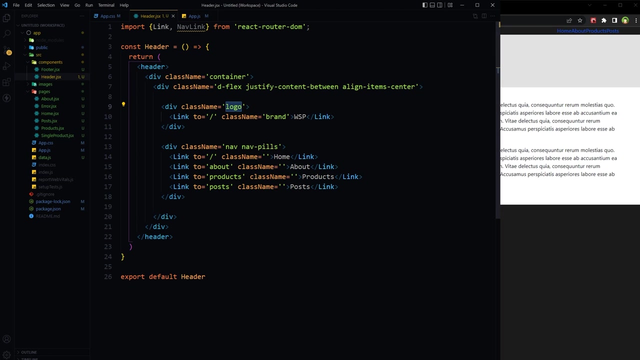 or just check data type or use pass and right. okay, so we have to style the footer and header. now let's style the header, let's close the single product, component data gone, products gone, header. so for after we have got the logo class and we have got header element, then we have got class, brand and then link. 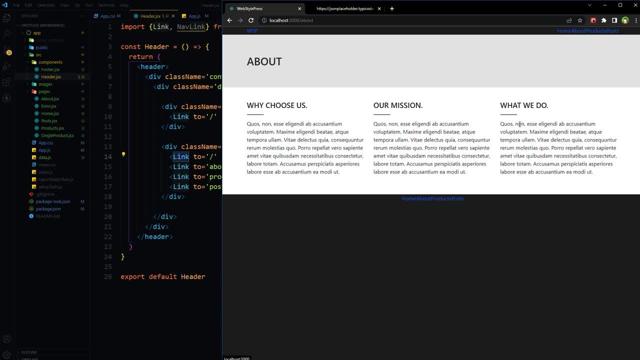 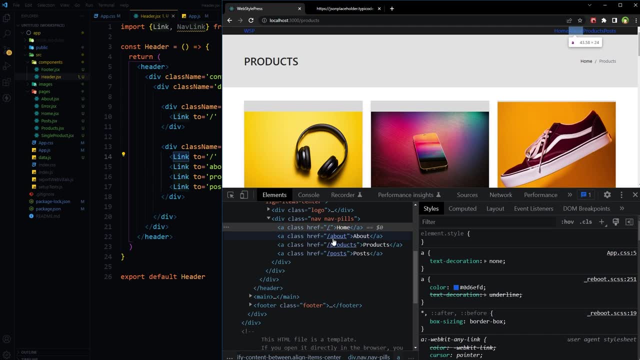 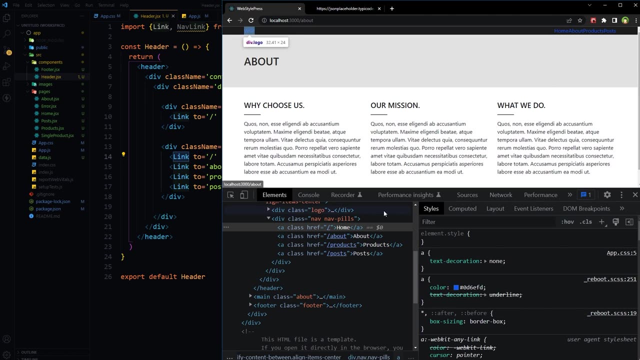 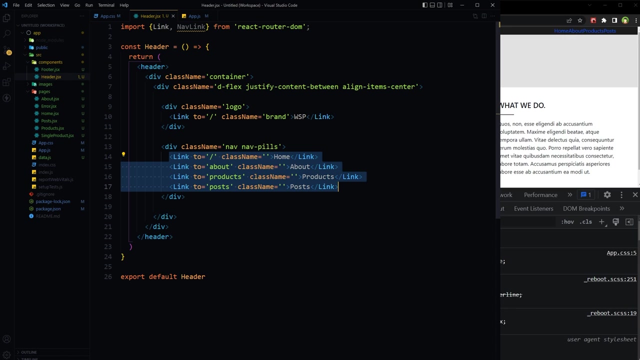 but here is the thing: this is simple link without any class. i want to display active class for active component, like if i am at the about page, then this about link should have a separate class indicating that we are currently displaying this component. for that this simple link thing will not work. we will have to use this nav link. so we will adjust that for logo this link. 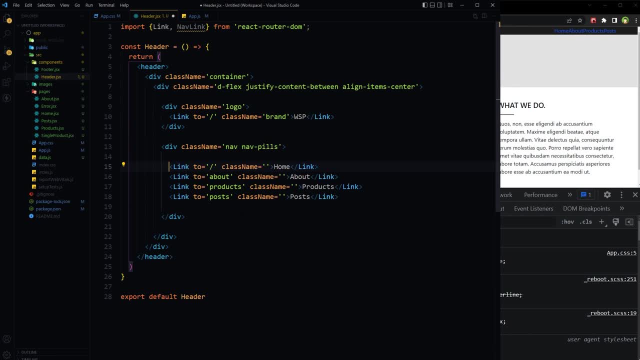 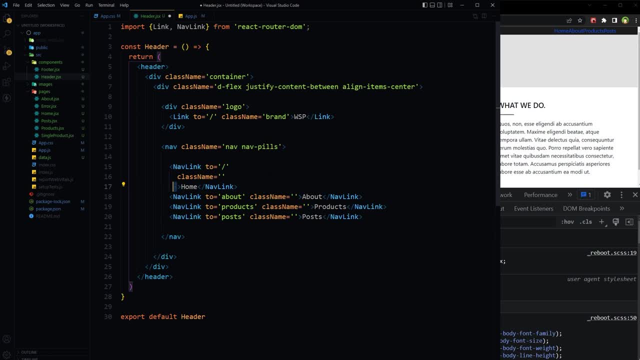 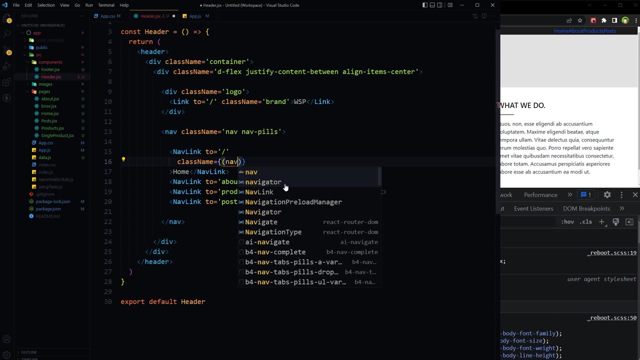 but class name will use a check. that will be we will take a parameter: nav data. nav data is active, then the class will be nav link and active otherwise. otherwise class will be just nav link and that's it basically. we'll have to use this thing for all. 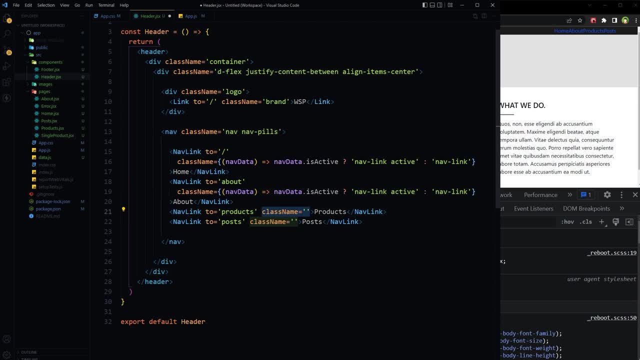 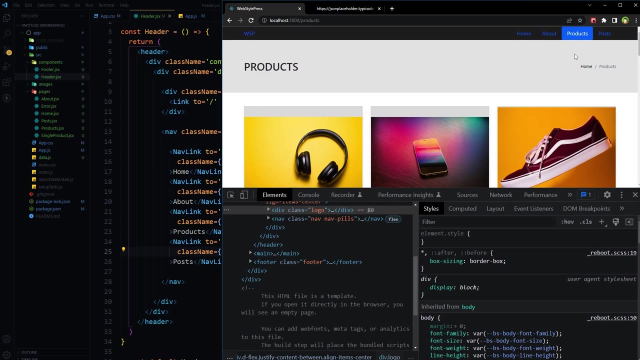 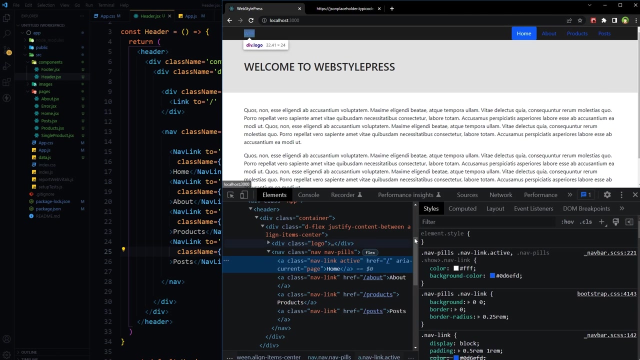 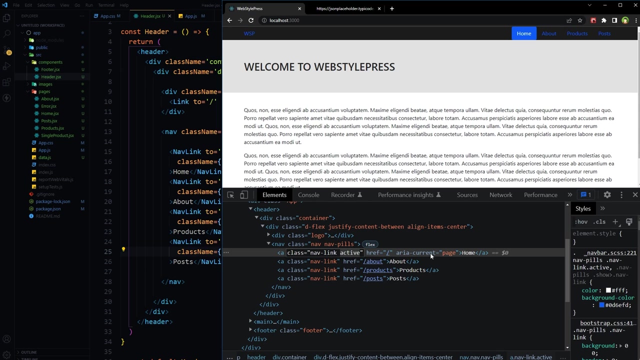 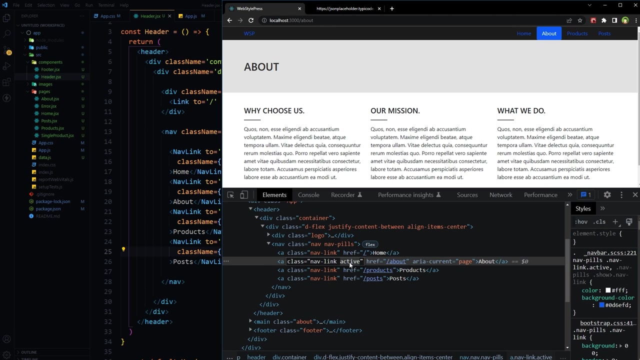 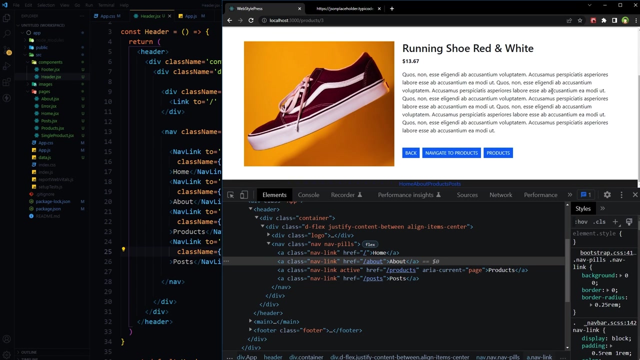 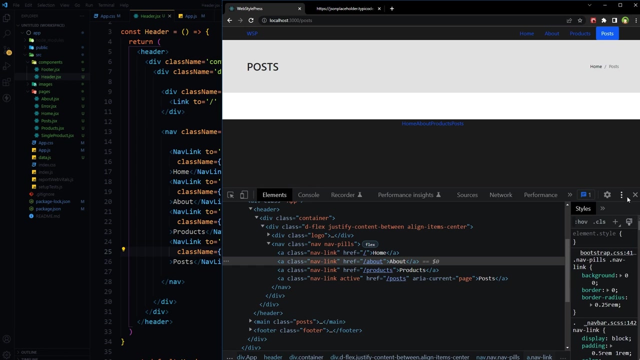 of these: save and now you see the class is changing. inspect is this nav link and active extra active class for this home page and if i go to about, then active is active. class is shifted here and for products about hosts, right, okay, so we've got extra classes now. nav link: active. 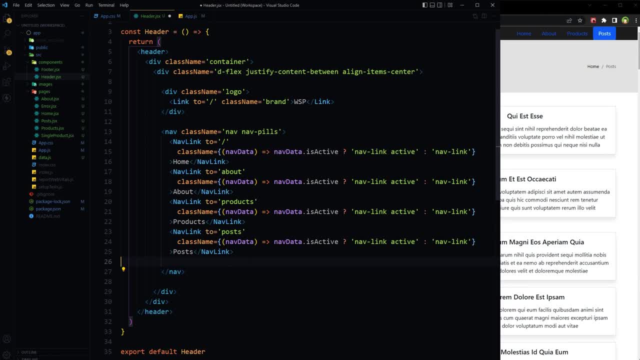 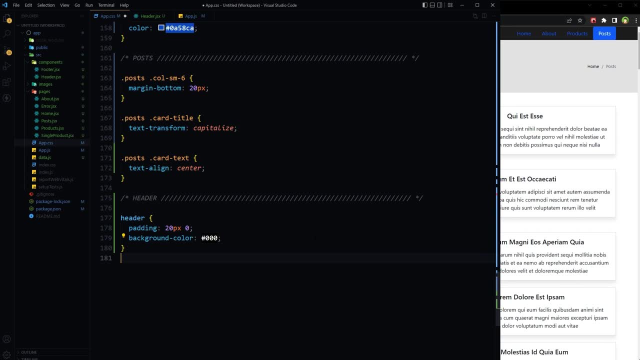 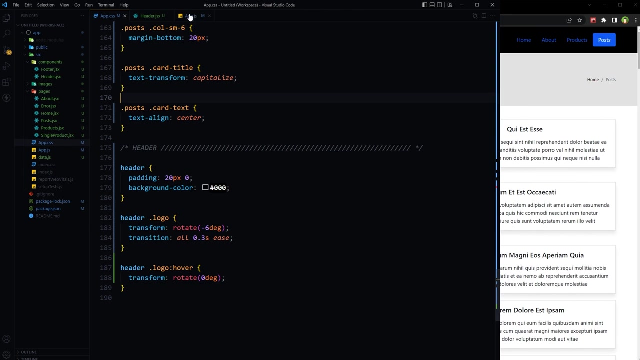 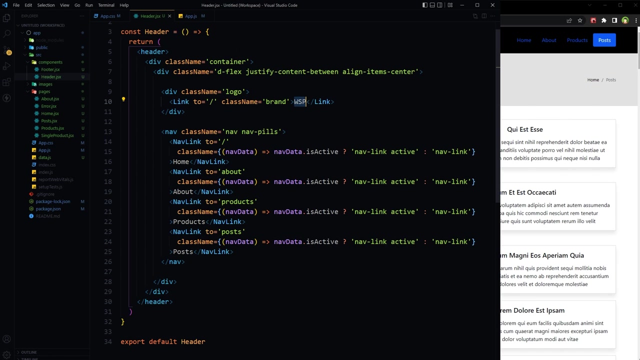 so let's handle these in css for the header. new css header will have padding and background header has got a class with name logo. it will have some transform property and logo at logo and edits over it will. logo will rotate and basically logo is this one and we've got brand here for this text. so header brand class. 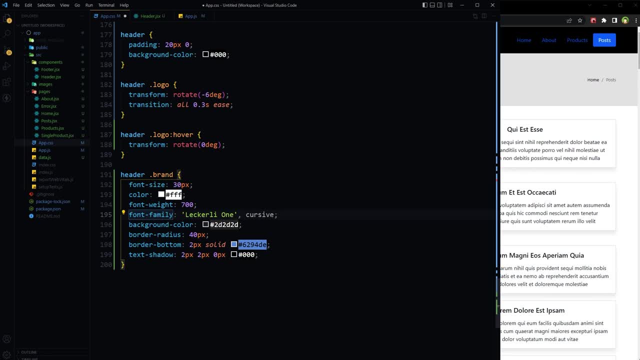 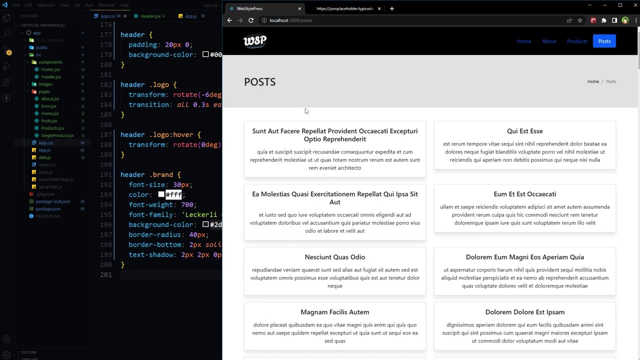 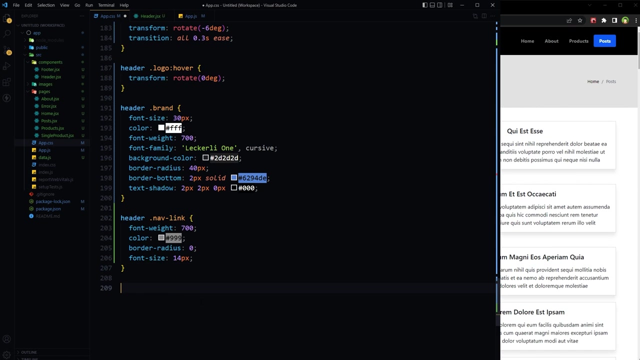 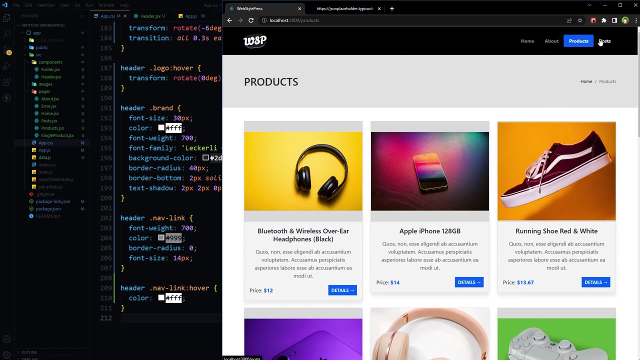 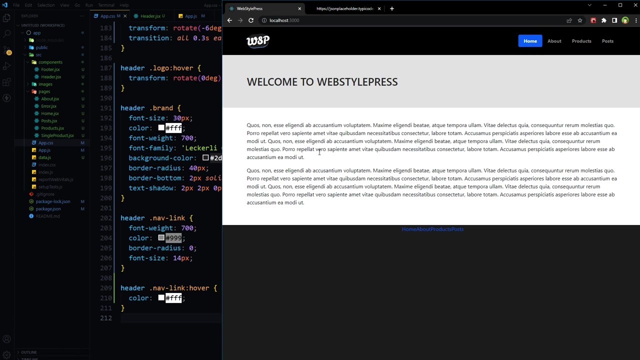 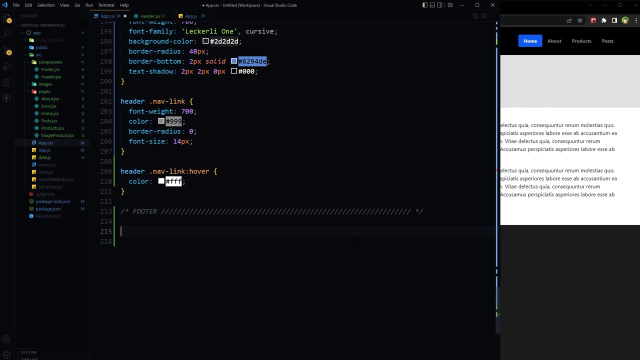 will have font size, color font weight, font family, specific font family. I don't color border radius, border bottom text shadow to make our logo look like this. then header has got nav link and a nav link hover. looking better now, right, so we want similar thing for the footer. similarly, CSS for the footer will be like this: like: 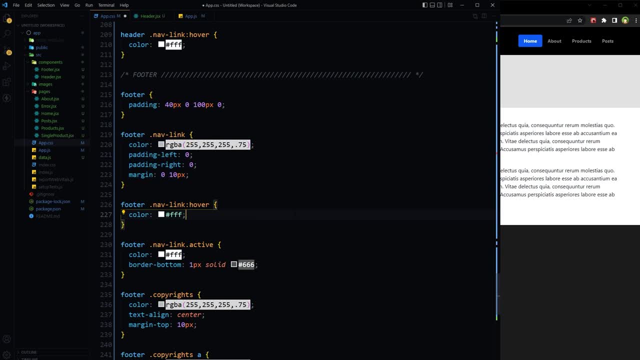 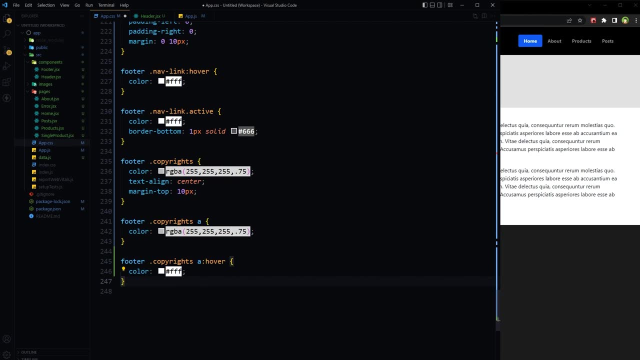 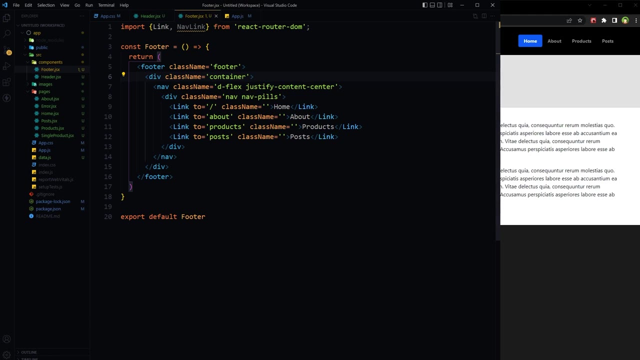 footer will have padding. footer will have nav link, nav link, hover, nav link, active for copyright text that we'll have to add. so let's open footer file, put a component file. so again, similar thing here. we don't need this div here. now nav element is fine. 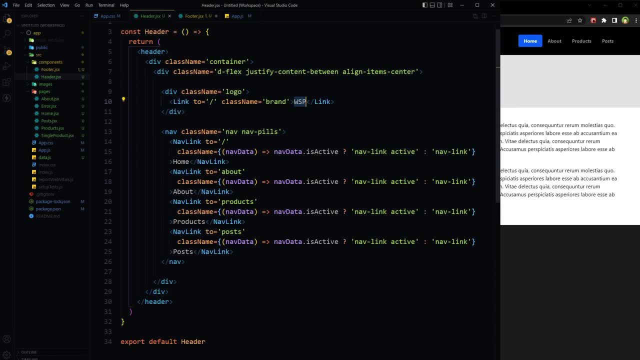 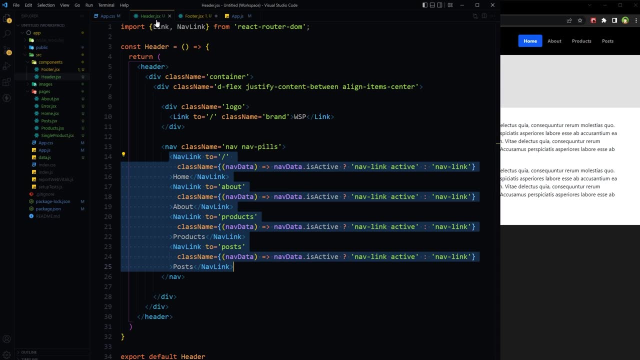 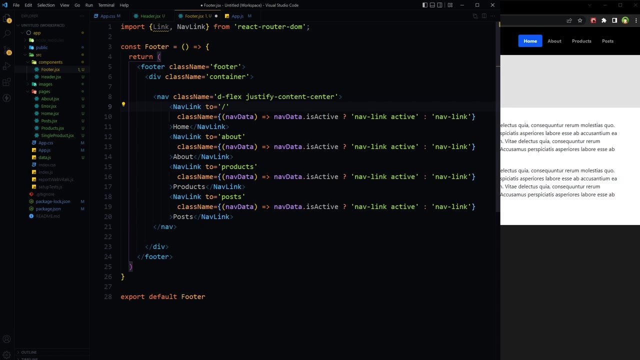 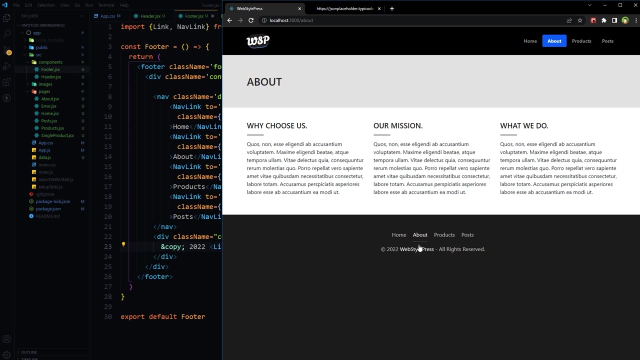 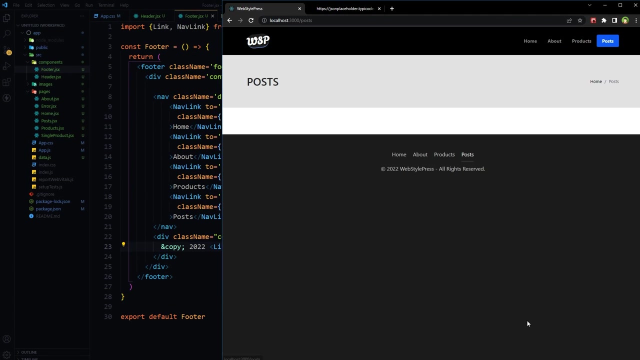 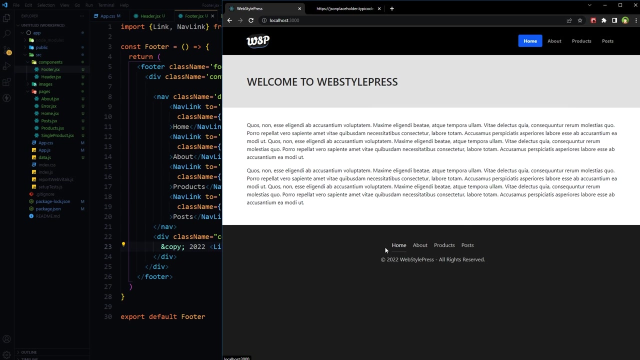 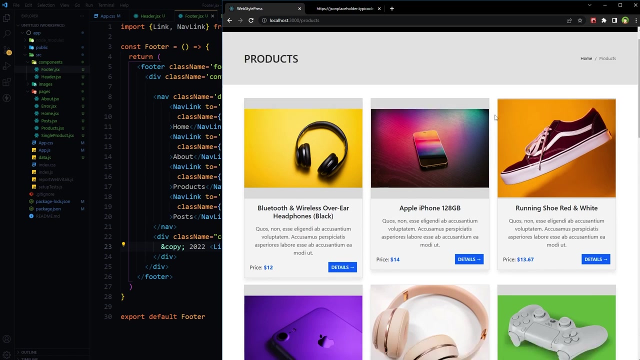 but they. this area will be similar. we'll use nav link instead of just link for footer. this same thing, basically, and after nav, we'll have copyright text. yeah, and we have got this result. now about you see this active active state products posts home about. see if I click here here: active class also ships about products posts. 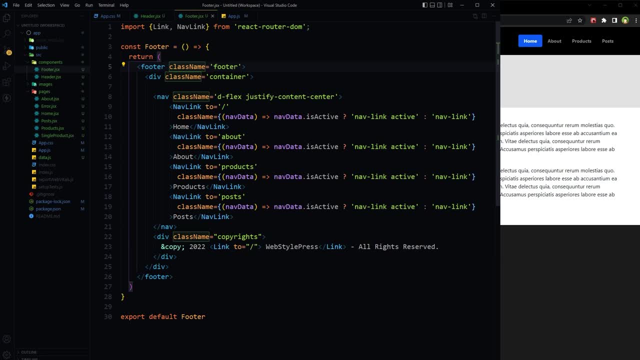 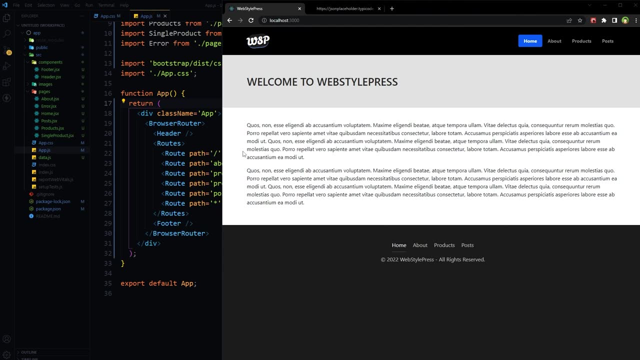 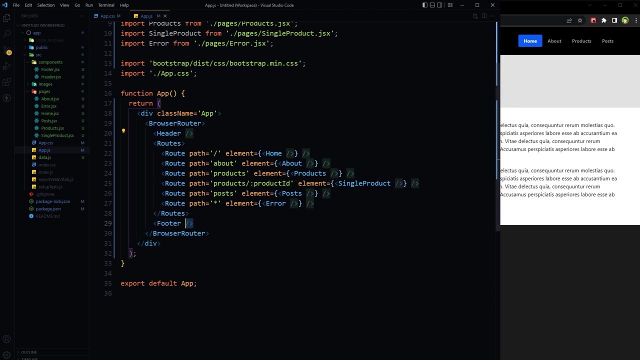 looking much, much better now. right, so there was our footer and this is our header, but still there is something that can be changed, or should we changed? you know we have used header here and footer here, and then here are our routes, and these are. you know we have used header here and footer here, and then here are our routes, and these are. 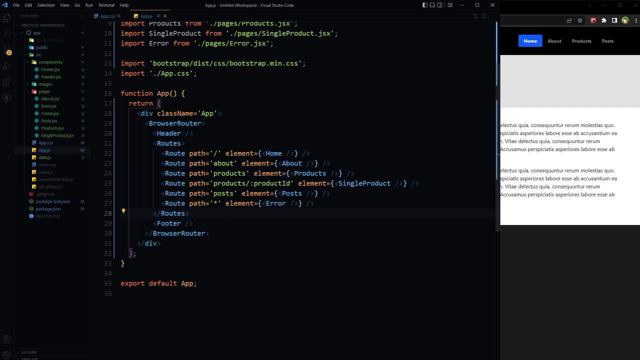 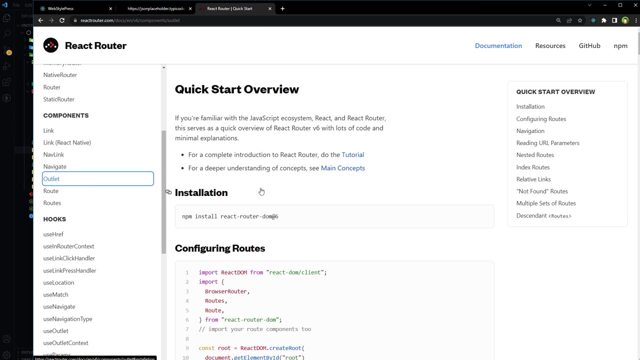 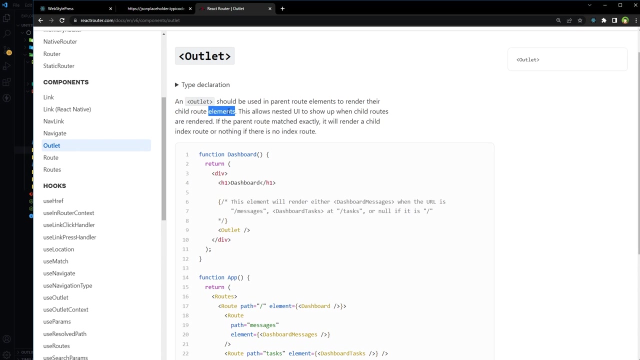 individual routes, home of our products, single product and header and footer are outside routes. this is wrong. this is a better way. this is react router and here we have got. outlet outlet should be used in parent route elements to render their child route elements. this allows nested ui to show up when child route. 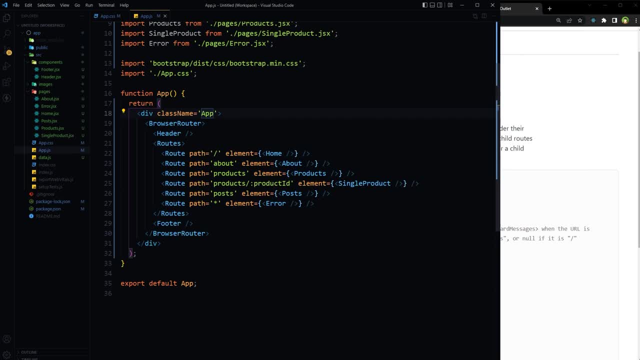 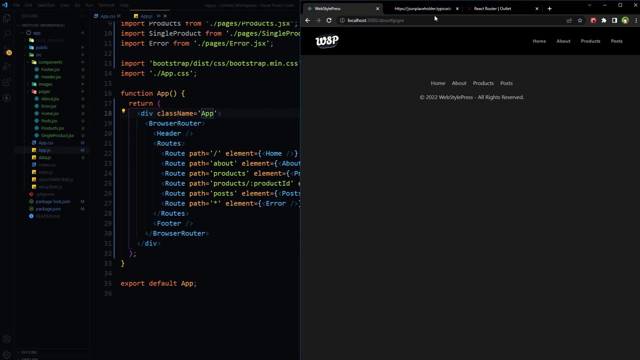 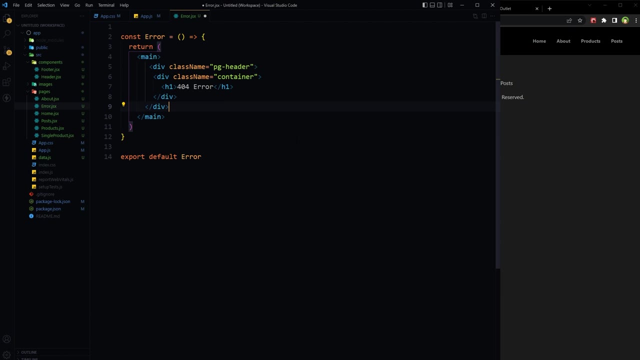 how do you do that? this is an easy to see type, if you are finding it because, for example, we have an cousin. what we are perfectly fine with does that keep our executors real to poisoned, and this is why it should not get to Value Pages. as you know, it's hardriser system because 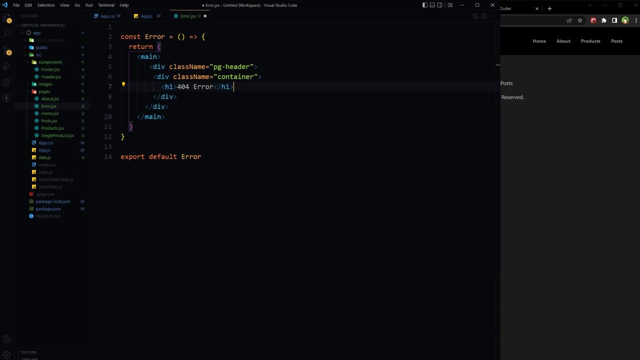 it may not be stable at the scheduled release date, but I really love display component valid. so this is just a tip, guys, that's for when you want to display saver for code. may you perform a little bit with your suiting consultants please我们就 trabal gest offended了. 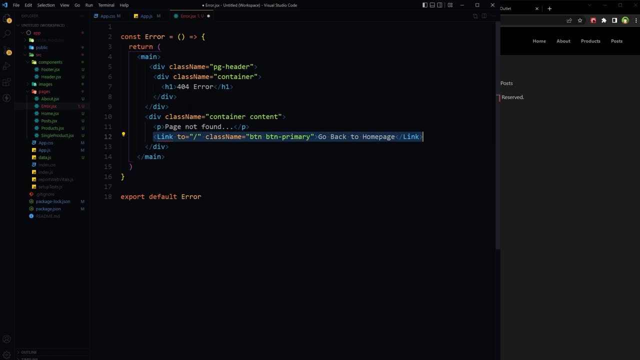 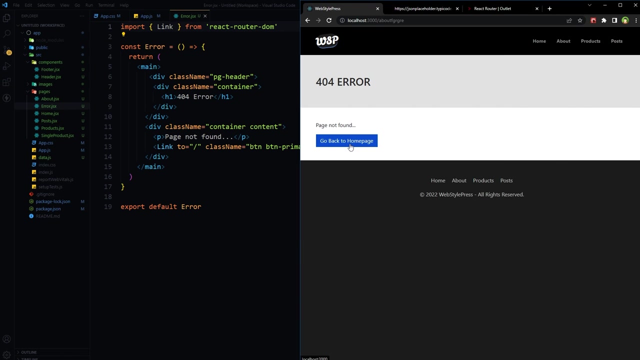 container content is not found and link to home page and that link for that link will import. link from react router dom like this. go back to home page. now we have gathered 404 as well. this is 404 page. okay, page not found. go back to home page. 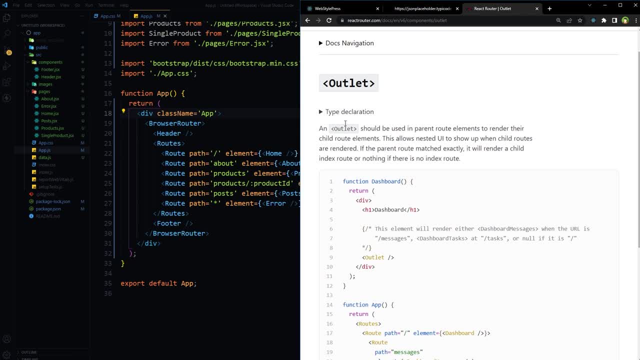 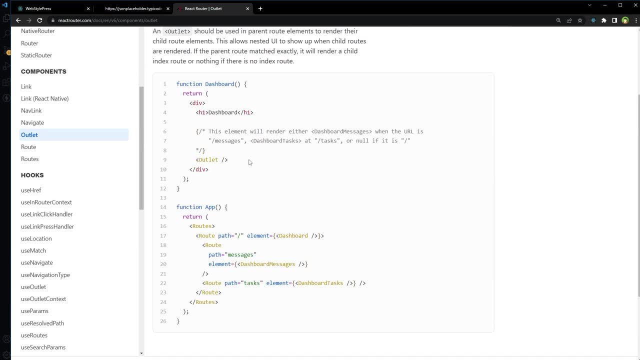 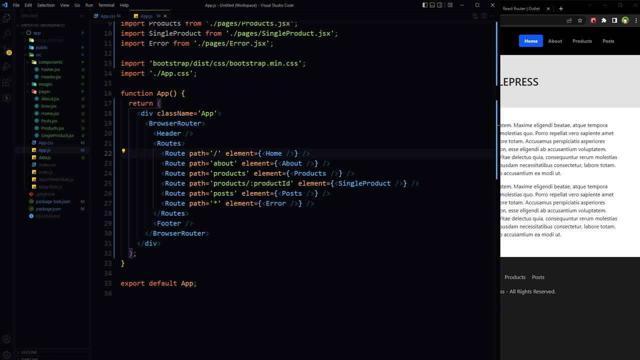 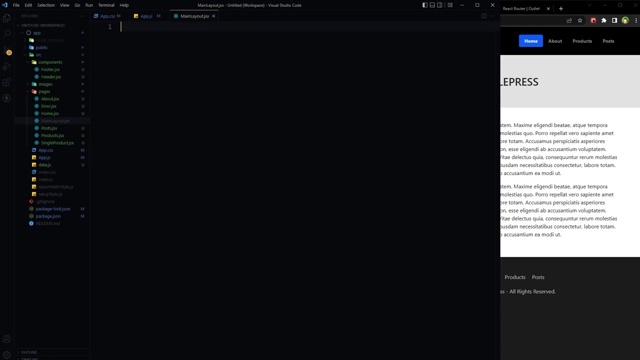 this is home page, cool, okay. so outlet, drought route, so this outlet. okay, we'll have to define a main layout, main layout for our app, like inside pages. let's create a new file and let's name it: main layout, dot jsx. inside main layout, let's import outlet from react router, dom, and then we'll import header. 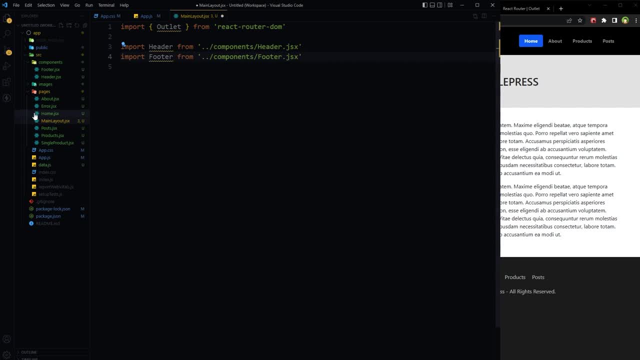 and footer from components. we'll go back from pages inside components and we're importing header and footer components because we'll be using these here. so here rafc main layout and it will return header and footer and also outlet outlet. so this is the proper way. this is our main layout that will have header, outlet and footer. 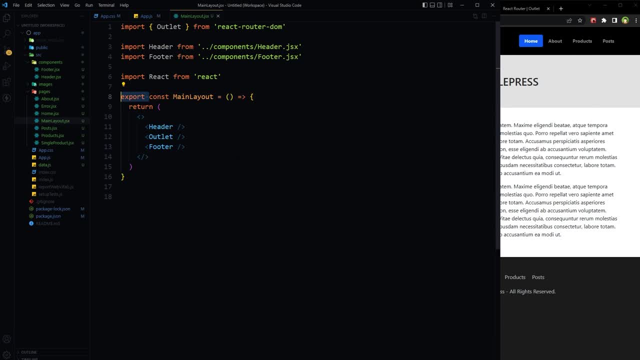 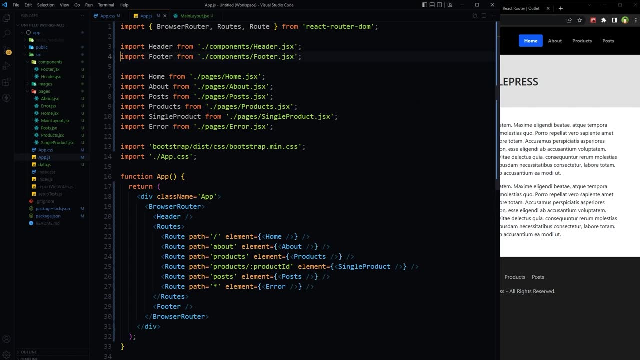 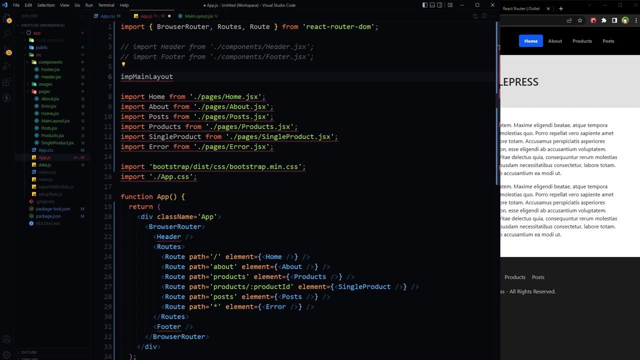 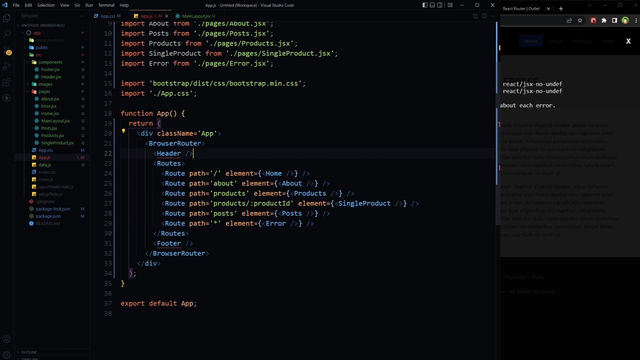 right now let's use just const and export default main layout. and now here we don't need to import header, footer now. instead we will import main layout from pages: main layout, dot, jsx, save. okay, so we now don't need header and footer like this. and now inside routes: we'll have main route and these will be nest. these will be child routes. 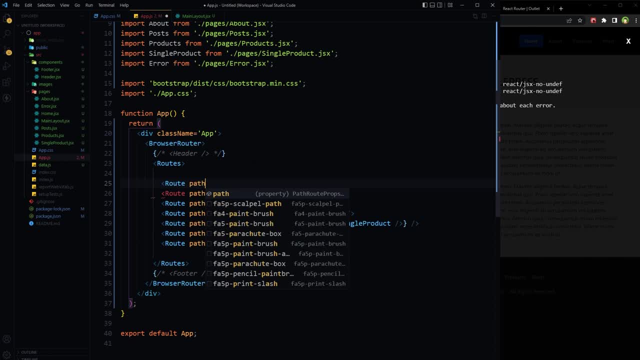 so here route path will be main medical route and these will be nest. these will be child routes, so style routes. so here route path will be ignore. test is Empty. current path of the page and password is normal. personal access is存在. dotum page and click save as awhats k? Yeap this site answer. we will match the file level in nur es hay think y dip it. in the yandere terminal file space will be the pic Command. 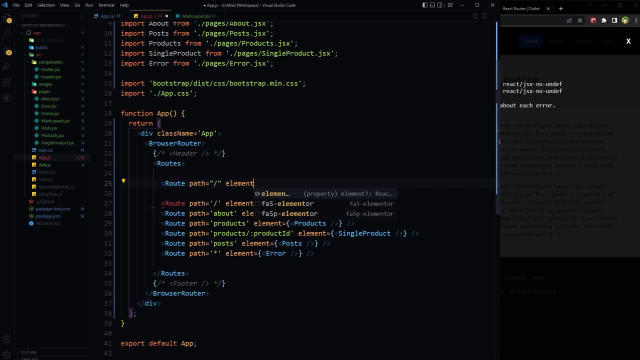 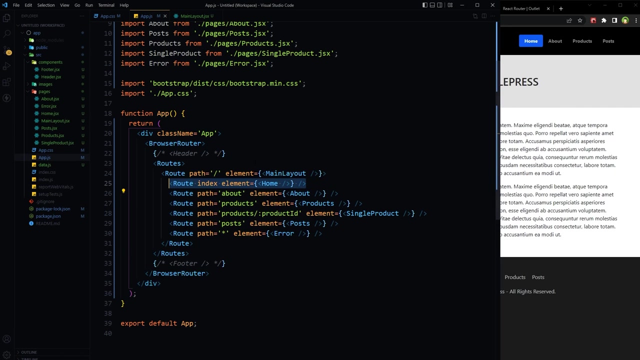 like root path and element will be main layout and that's it. and this route will enclose these routes or wrap around these all routes, the routes, and here now this will become index save and that's it now. this is the root and this is home page index page. 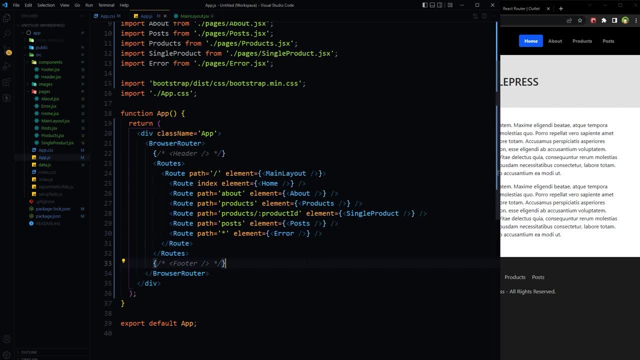 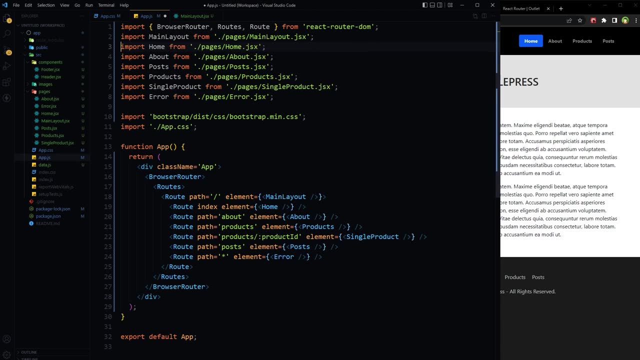 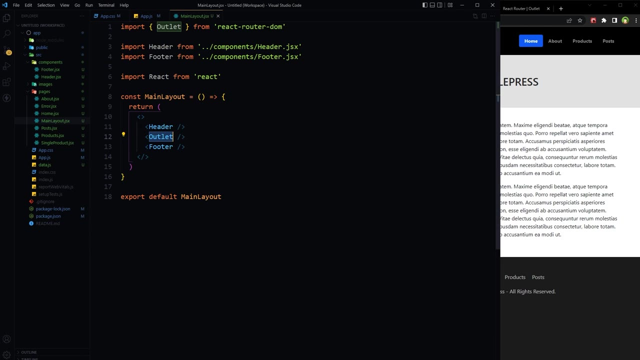 and rest of everything is same. so now we don't need this footer here, don't need header here and we don't need to import header footer here, and this is our main layout with outlet. we should use a main, main layout for our app or website and use header footer inside. 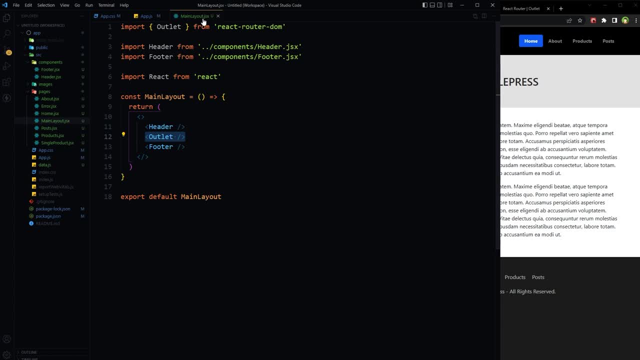 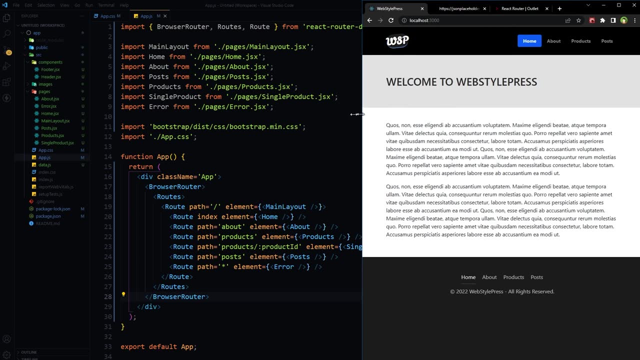 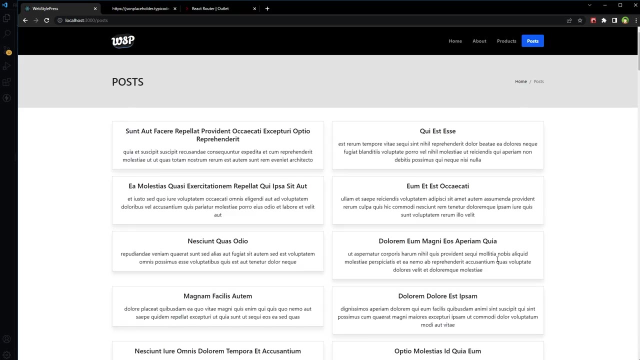 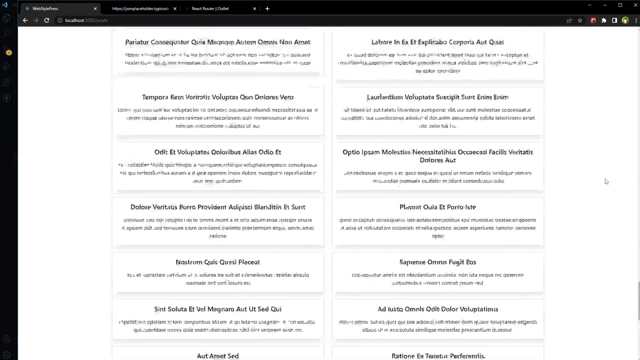 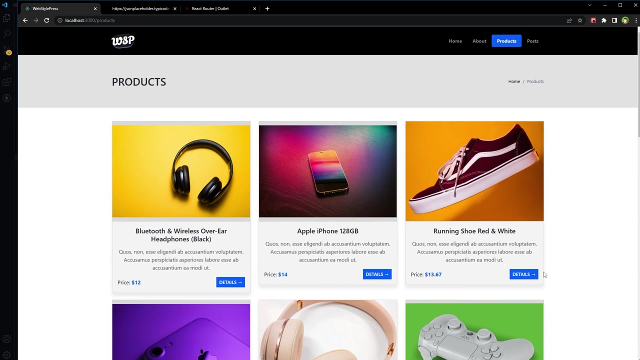 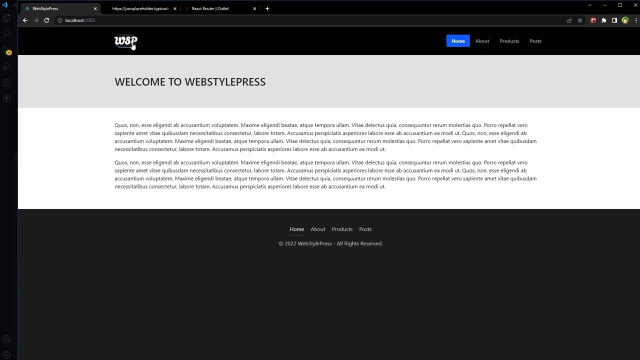 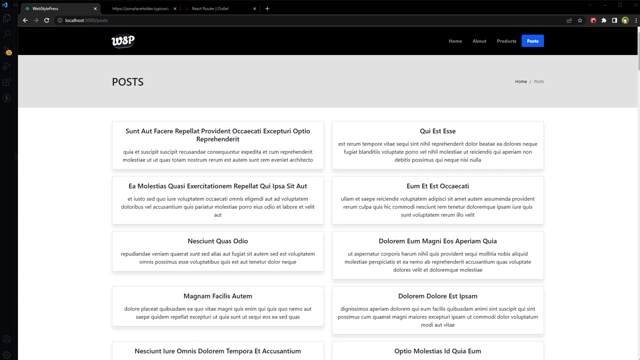 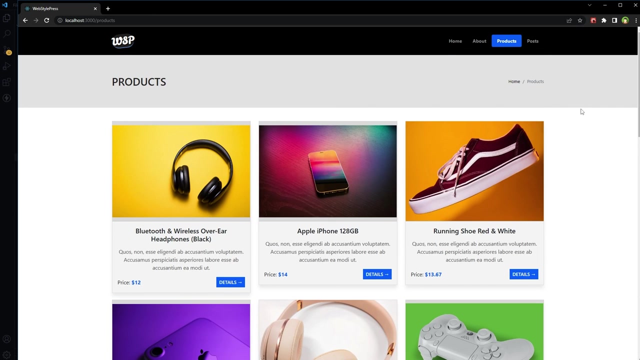 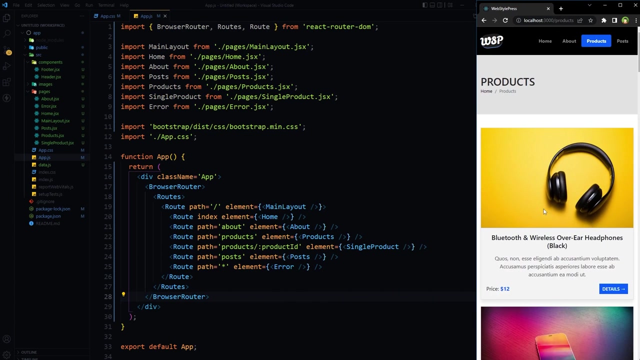 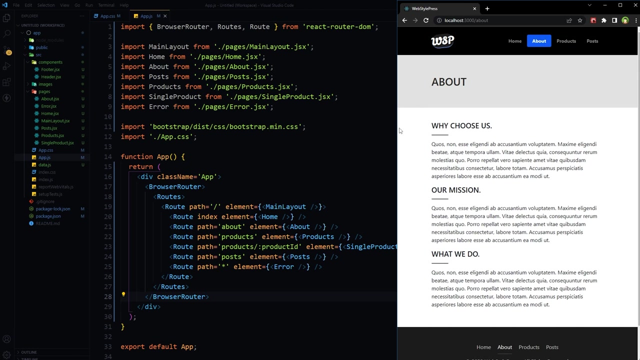 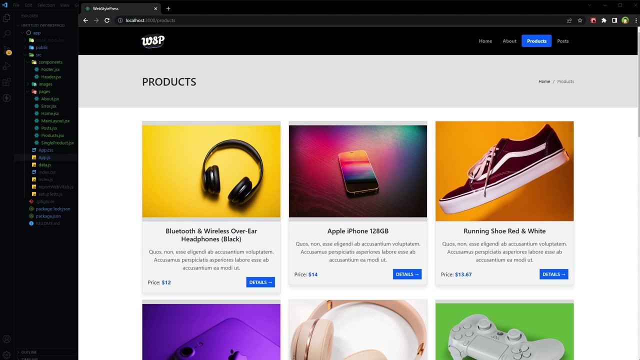 and then in between outlet, and then arrange our components like this: and now it will work as expected and fine posts, no errors products, single product about home working, fine right, and our app is also responsive. thomas, this is how you can create routes by using latest react router. 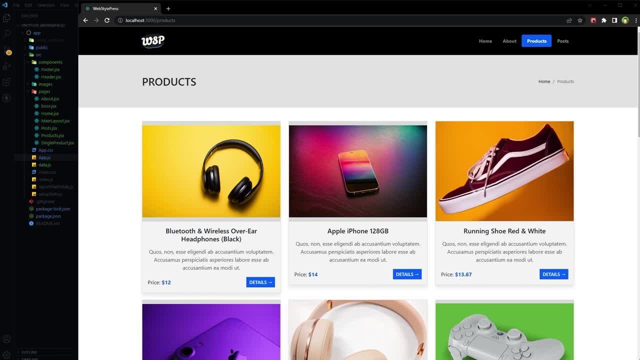 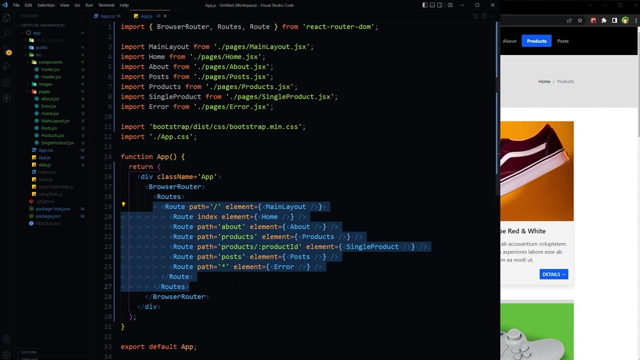 use dynamic classes in menus, get url parameters to show specific data and all that good stuff. this new react router has smart router where router has better algorithm to understand request to navigate to better result from given routes. okay, i will link the files. uh for this tutorial in description. 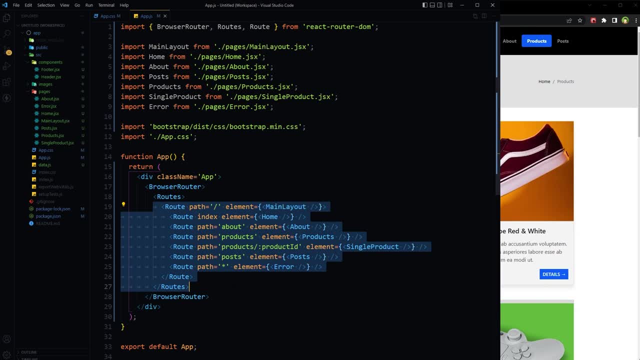 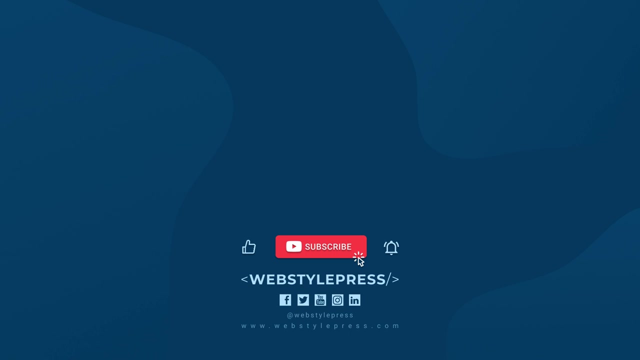 you can download this app from there. if you have any question, you can comment down below and please give this tutorial a like and subscribe if you haven't already, and i hope this tutorial helped. and again, like, video, comment and subscribe and i will see you in the next video.